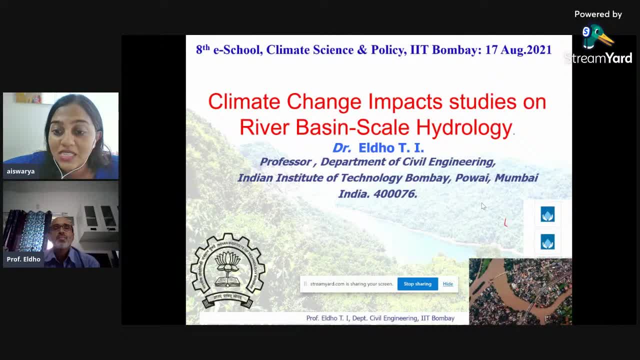 many prestigious awards, including eminent water resources scientist cons constituted by Indian Water Resource Society in 2018.. Welcome you, sir. Okay, thank you, Aishwarya. So all participants, very good evening and welcome to this ATE school on climate science and policy, which is yesterday. 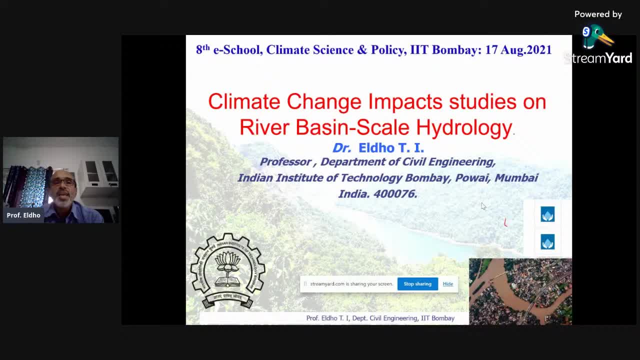 was inaugurated and that will be continuing another few more days. So the first lecture which you are going to hear is on climate science and policy. So the first lecture which you are going to hear is from me only. So, as Aishwarya already introduced about me, I will not go further. 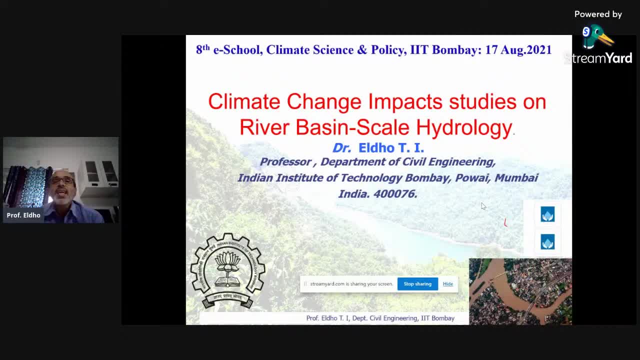 on about me, but I am working this area for last 10 years, especially on climate change in the area of river basin scale, especially hydrology is concerned. So current, today's topic is climate change impact studies on river basin scale hydrology. So, as all of you, how recently I 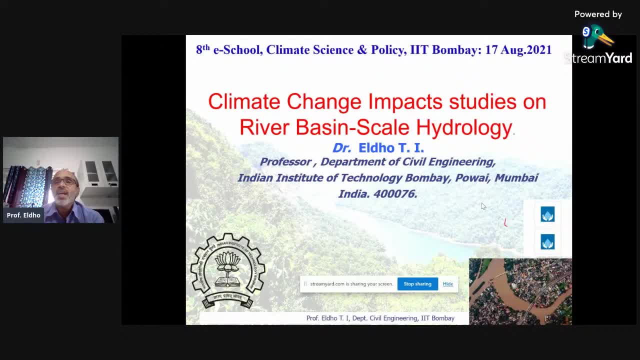 mean last few days. you would have seen in various newspapers and media about the IP 6 report and assessment report 6, and then it's various contents you have seen. So, as we have already observed, so there is a major issue of climate change which is going. 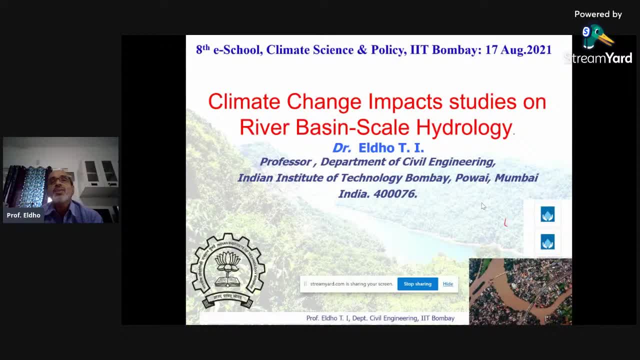 to come and then various issues we have to deal, as the climate change is going to be, it is a reality and then it will be continuing for a long time and we have to take appropriate actions. So that way, this course is very relevant and various aspects of climate aspects and climate. 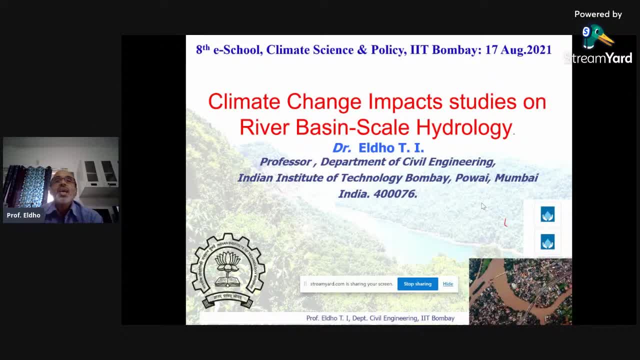 science and policies will be discussed in the coming lectures. So, anyway, this first lecture is on the hydrology. what are the impacts on hydrology is concerned? So, as all of you know that say water is life, without water we cannot live. So that way you can see that the what are the impacts of climate change on water resources. 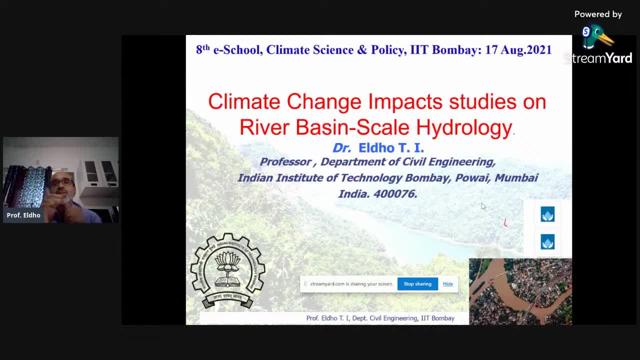 or hydrology. So it is a very, very important question and the past few decades of studies showed that say very severe impact is there on hydrology as far as climate change is concerned. So today's topic is on climate change impacts on river basin scale. 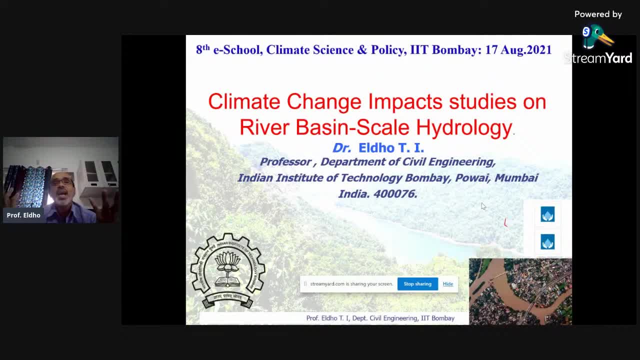 So why river basin scale? Of course I could have presented for the entire country or for the for the particular region is concerned, but I am concentrating on the river basin scale, since that is as a hydrologist concerned. Hydrologist is concerned. River basin is the fundamental unit on which we do all the water resource assessments and 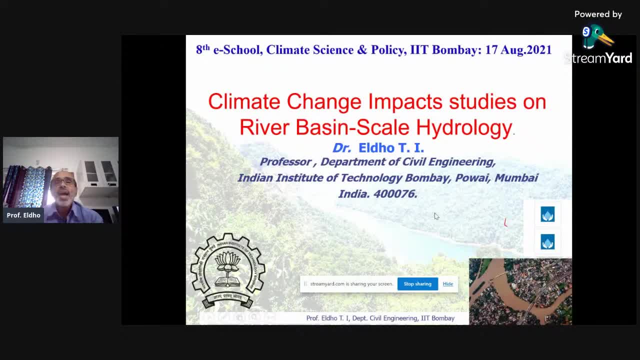 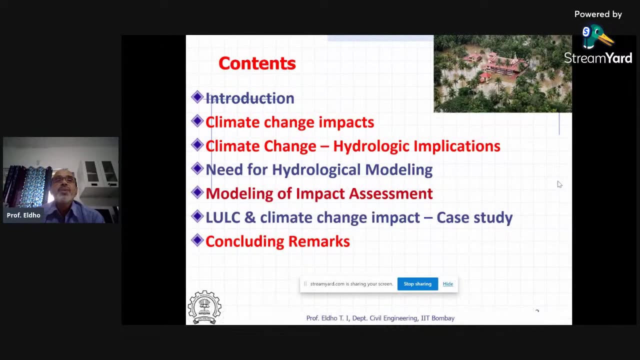 all the aspects as far as the hydrologist is concerned. So that way it is very relevant and very important to do appropriate assessments as far as the climate change related to river basin hydrology is concerned. So in this topic, first we will have a brief introduction and then we will be looking to 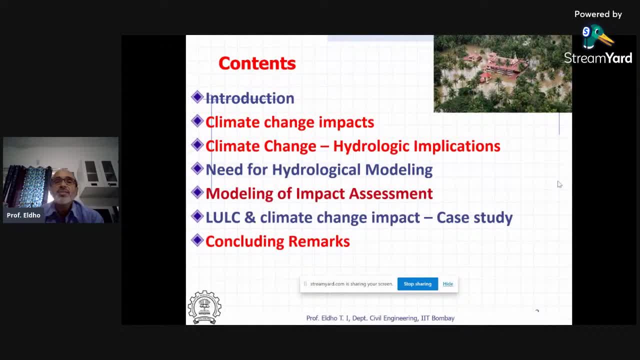 various aspects of climate change and its impact, So especially in types of hydrological impacts, and then we will be discussing why we need to go for hydrological modeling. So, as I mentioned, since hydrology is so complex, so especially to take a river basin large, 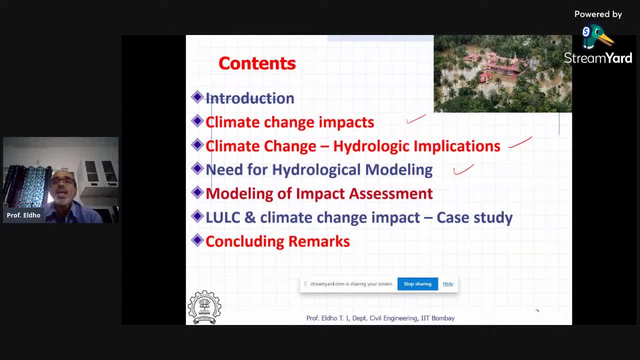 river basins or river basins can be very small to very large, like it can be even of the 500,000 square kilometer or above, or it can be 50 square kilometer. like that. it can be very small to very large. So what are the implications? 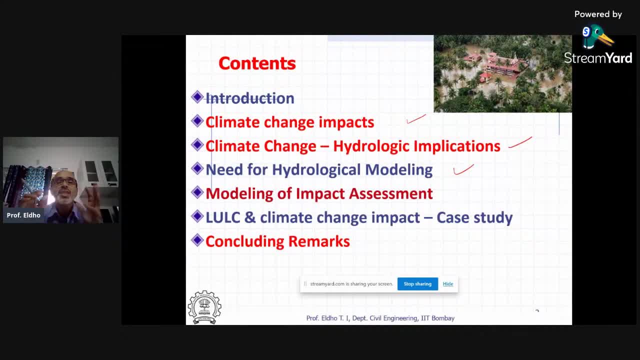 Say, of climate change with respect to hydrologist concerned on a river basin scale. we need models, So hydrological models are essential. So in this lecture, main emphasis will be how to utilize specific hydrological models for climate change impact assessment. So then we will be looking to how we will do the modeling of impact assessments and 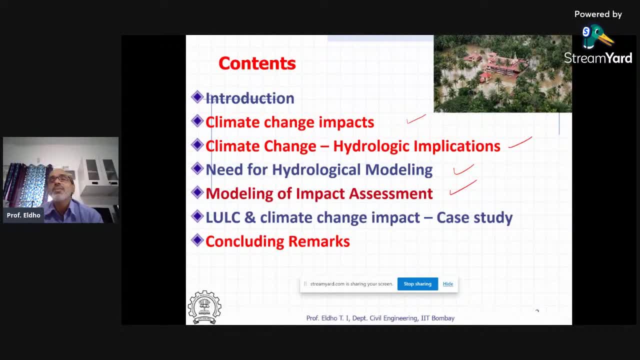 then we will be further discussing a case study, a detailed case study we will be discussing here to show how we can do this. So if any of anyone of you- those who are interested to do further research or studies like this, you can take this into account- how we are going to do such studies and then how we get 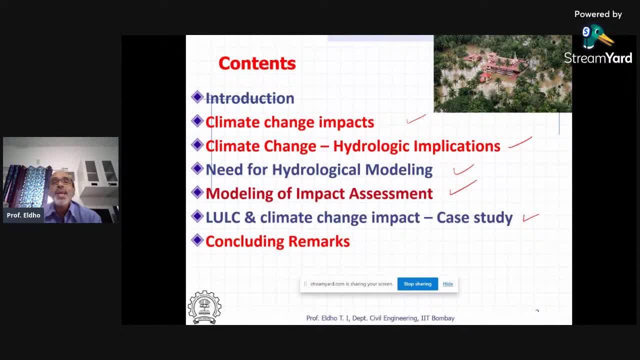 the results and then how we interpret it. So that will be the main theme of this lecture and we will be concluding with a few remarks. as far as the climate change impacts on hydrology is concerned, So as all of you know that. So water availability is very important. 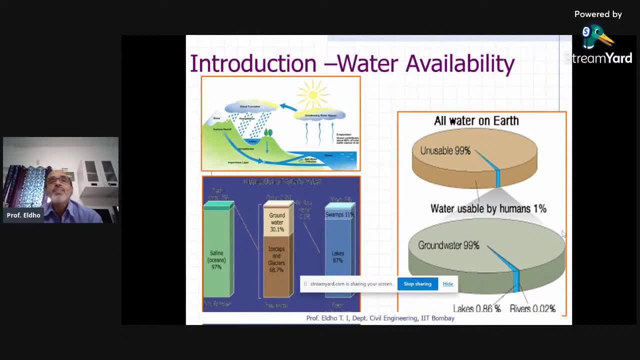 It is very important. It is very important Even though we have got so much water on earth but water usable is hardly 1%. is water usable by humans, Even so much water, I mean say, the remaining water, whatever is there, maybe in glaciers? 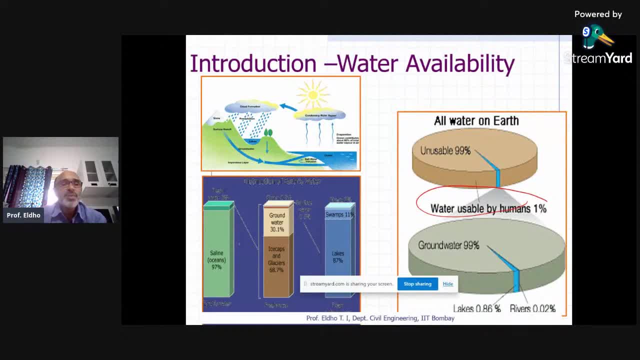 So of course you can see that sea water is, say, larger amount, and then whatever is available. So humankind is only 1%, And out of this 1%, even mostly, 99% is in the groundwater, And 1% is actually what is available for surface water in terms of rivers, lakes. and then what? 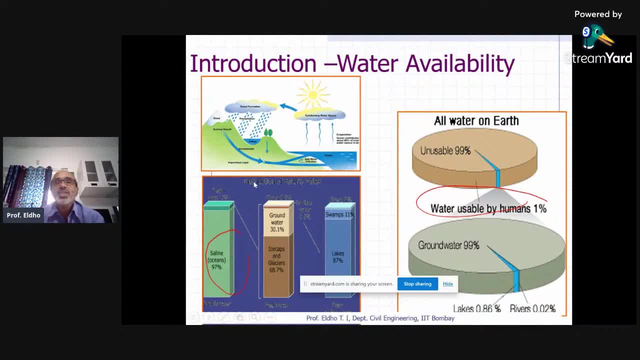 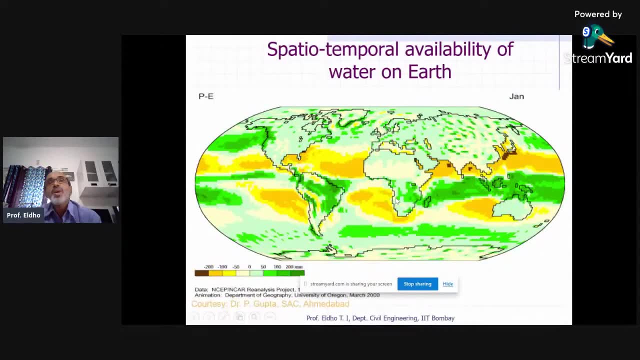 is, we can directly extract as far as our utilization is concerned. So that way, water resource is very much affected with respect to the various like climate change or other aspects. So when we look into water resources, They make issues. These things are changing. 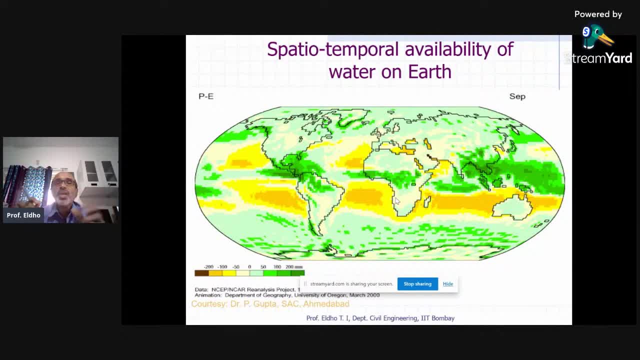 I mean whatever say the availability of water, or with respect to rainfall, or whatever is happening, That will be keep on changing with respect to space and time. So say, for example, in India we have got a monsoon starting from June to say September or October. 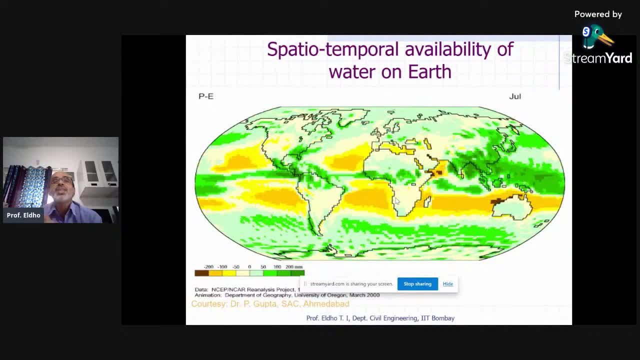 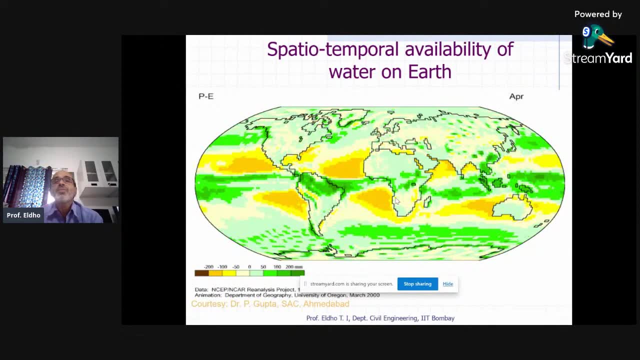 And then say 4 to 5 months all the rains happens and then there is no rainfall. say afterwards: So that way, say next 7 to 8 months we have to deal with whatever is What we got through the rainfall. So that way it is so important to study, say using a particular hydrological model. 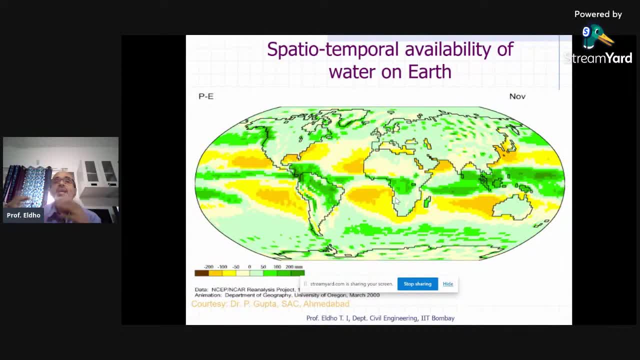 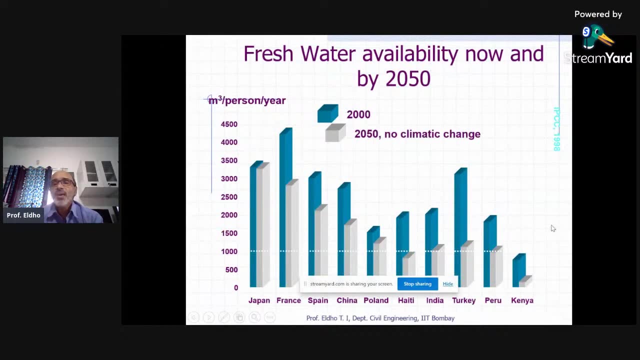 What is what can happen on a river basin scale, on a state or a region scale, or the total country. So that is the major issue as far as hydrology is concerned is ratio, temporal, with the water on earth and its variations. So now, as I mentioned, so water availability is so important. 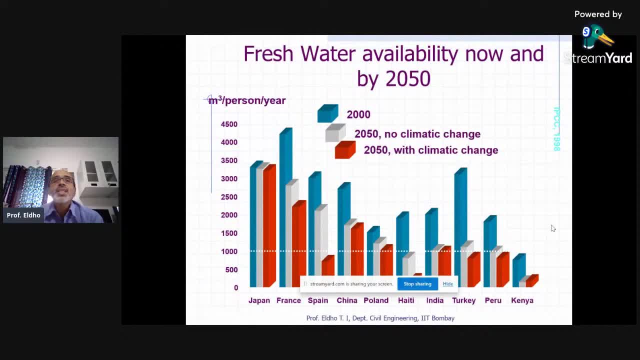 But now if you look into, say, for example, as per the past studies say fresh water availability now and by 2050. So even though this study was done by 2000, so you can see that country wise, so huge variations you can see, Say, for example, in India's consent, if you are having say, for example, say around 2000. 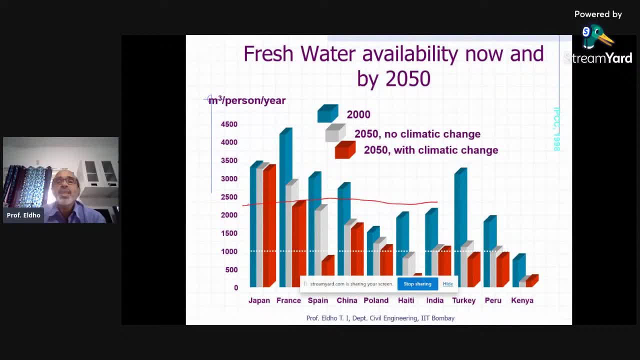 cubic meter per person per year, say by the year 2000.. Now it has drastically reduced, And by 2050.. By 2050. It will be hardly thousands a meter cube per person per year. So that way, so then impacts a quite much income. 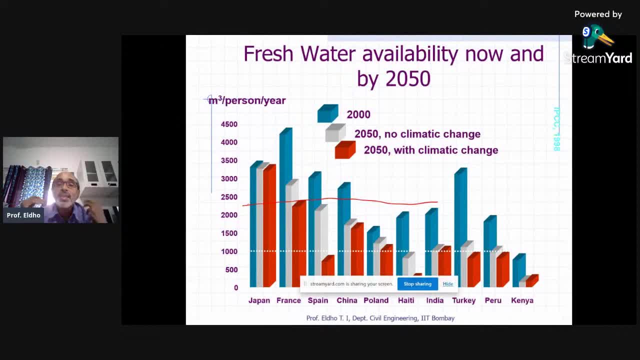 So those thingsщё, whatever is water available is so low And we the climate change impact also in a severe way coming to picture As far as hydrology is concerned, It would be a major challenge and a major issue As far as available water sources conservation. 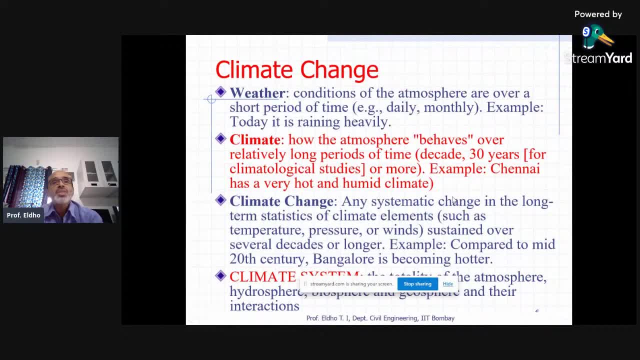 So that we need to study the impacts on this climate change, change as far as hydrology is concerned and especially a river basin is concerned. So why river basins? as I mentioned, River basin is the scientific unit through which we can do all kinds of water resource. 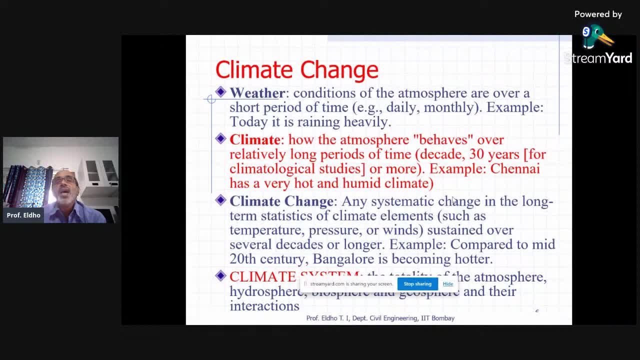 assessments And so, with respect to climate change, what is happening, it is much better to study on a river basin scale. So, coming back to climate change, as all of you know the difference between weather and climate, So weather means conditions of atmosphere. 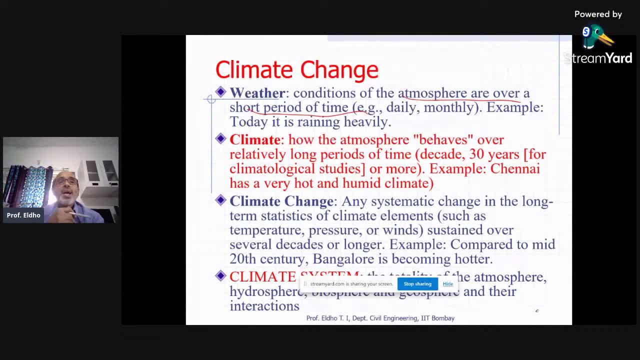 over a short period of time, So like daily, weekly or monthly. So today it may rain heavily means So it is only today or tomorrow, like that. So within what is going to happen immediately or what happens last few days. So with respect to that is what we call it as weather. 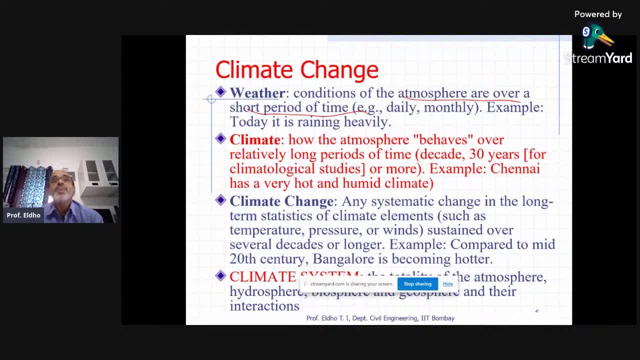 But climate is concerned. So this is when we look into. we are looking for what is happening long time. So climate means how the atmosphere behaves over relatively long periods. So generally, in all this analysis you take 30 minutes. You take 30 years for climate studies. 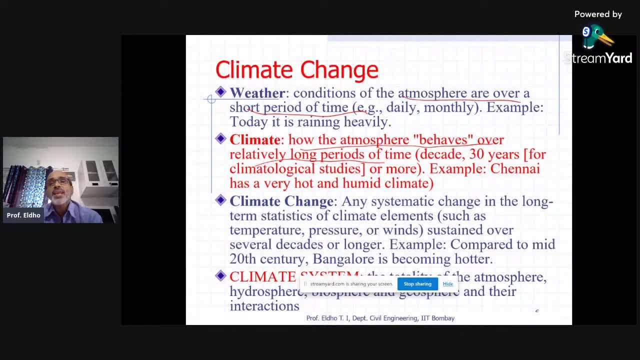 So now say, for example, if Chennai has a very hot and humid climate nowadays, so compared to say so when you assess, when you analyze last 30 years, so it is that, what is the behavior, what is happening. So that is what we call it as climate. 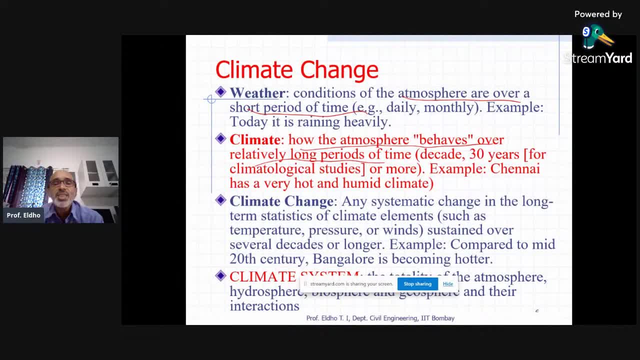 So then, coming back to climate change, So climate change, as you can observe, so it is any systematic change in the long-term status of climate elements, such as it can be. So climate change, as hydrology is concerned, generally, we talk about temperature. 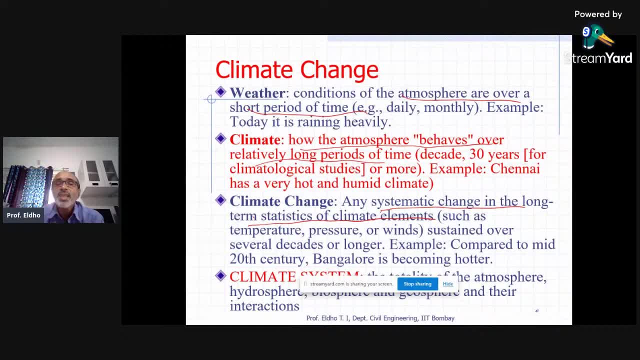 And then, of course, climate change is mainly- we are mainly on the temperature increase And then due to the GHG gases, like carbon dioxide So, such as temperature pressure or winds sustained over several decades or longer, So, as I again mentioned, compared to mid-20th century. 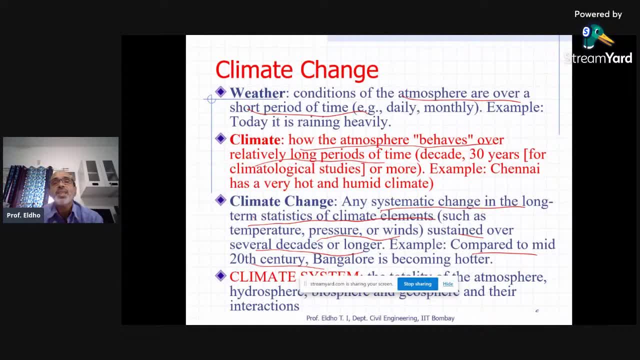 so if you say that Bangalore is becoming hotter, so that is the reason, is that that is what we say as climate change. So now the climate change, climate change, climate change system is concerned. So here, so you can see that it is a complex system. 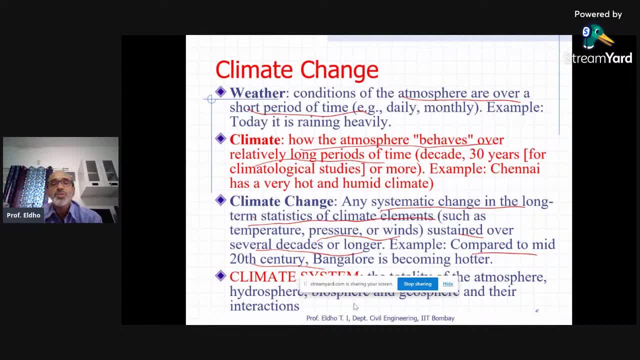 So atmosphere is there, hydrosphere is there and biosphere and geosphere And all these interactions we need to study. So that is the climate issue is concerned. So luckily we are having global circulation or general circulation. models are with us. 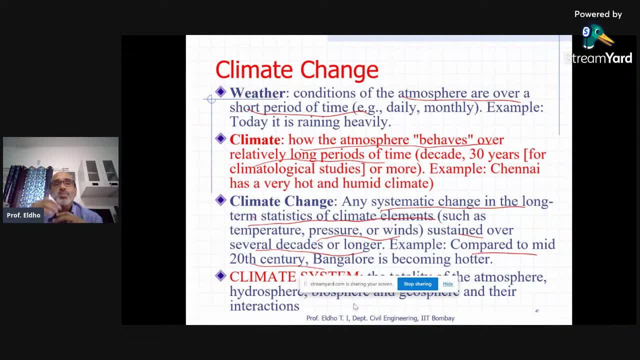 so which we can effectively utilize to study in terms of what can happen. It can be with respect to changes in temperature, changes in precipitations and then the climate change in, say, like pressure variation or winds. So all these things, we call this a climate change. 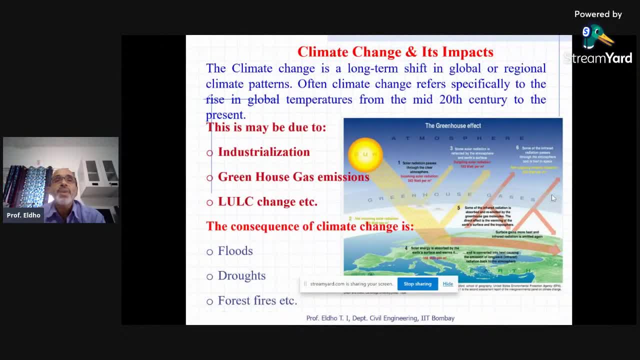 So now the climate change as you can see that we are feeling now. this climate change last a few weekends, And then what are its impact? So the climate change at its impact is it is a long-term shift in global or regional pattern, as I've already mentioned. 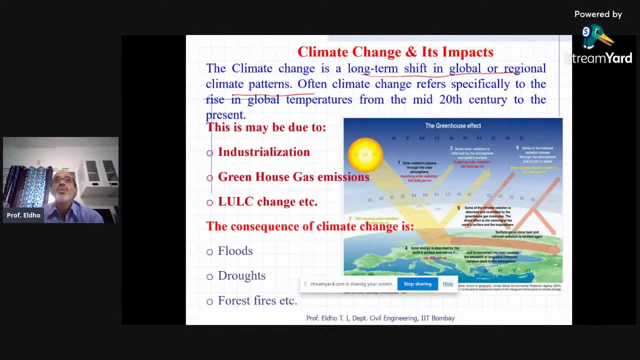 So often, climate change refers specifically to the rise in temperature. We always talk about the rise in temperature. so that is now. we have already identified that this is due to greenhouse gas emissions and the industrialization that has happened last one century, And then so, of course, other than that, say the agro-political effect, like land use, land cover changes, so that is happening, that is also contributing as far as the climate change is concerned. 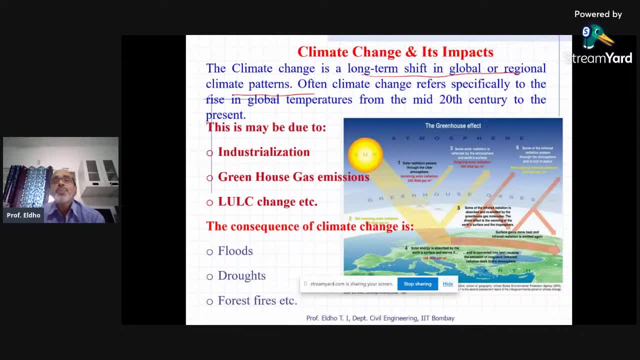 So, as you can see, that, say within the perspective of climate change, there are so many impacts we can observe and so much of studies are going on, So that can be, in terms of hydrology, like floods or lack of water, say, like droughts. 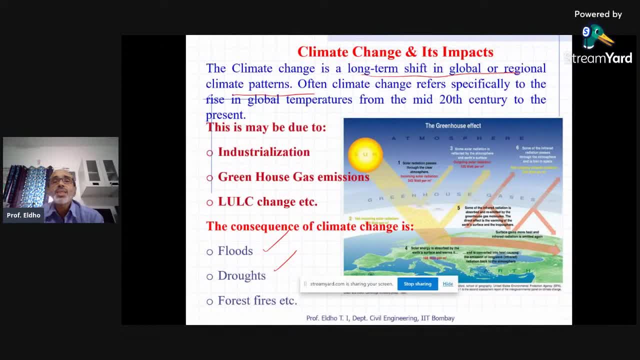 So that can be, or just you can see that say now in US you read in newspapers forest fires, or in Australia last year or two years back, And then this kind of all these kinds of issues can come. 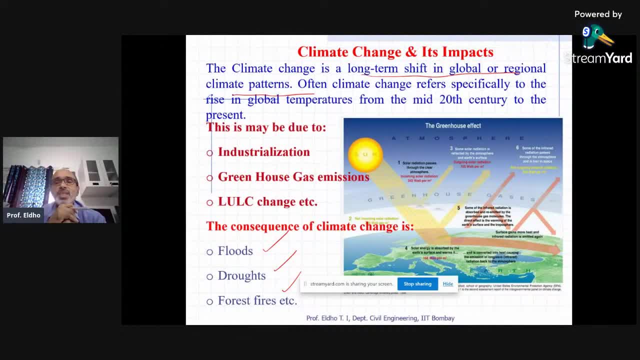 So these are some of the impacts as far as climate change is concerned. So, as you can see here, the greenhouse gas- and then what is happening is very clear with respect to some of the infrared radiation- is absorbed and then the atmosphere is heating up, and that are the main impacts. 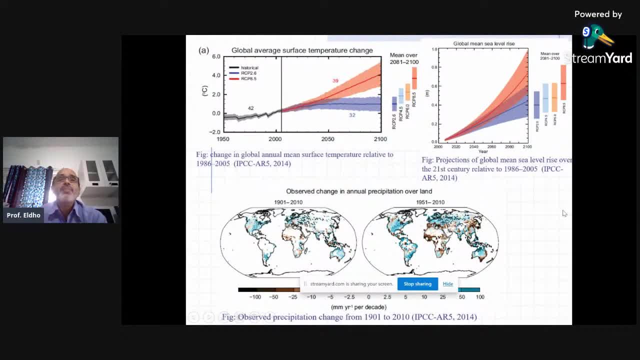 So what are the effects, after effects we can see, from this climate change? So, as I mentioned, mainly what we can feel, or what we can observe directly, is the change in climate. So you can see that, say now. these results are from assessment report 5, which was published in 2014.. 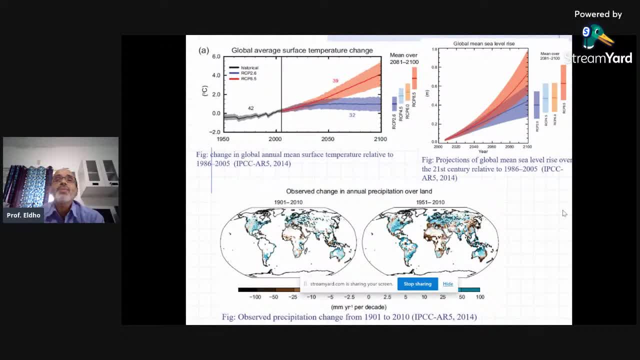 I will show what is there in 2021, what is published in CMIP 6 also. I will just have a brief introduction, But most of the studies, what I will be presenting is with respect to the CMIP 5 reports and then corresponding the assessments. 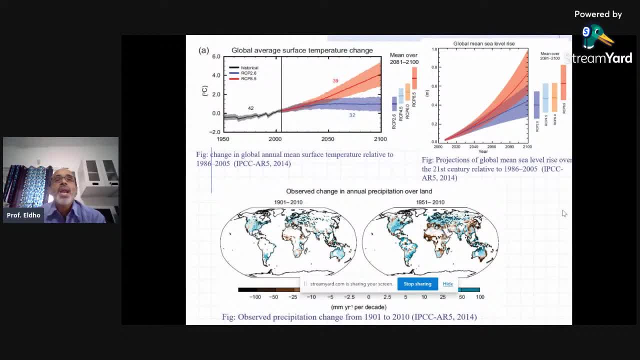 So here, as you can see that, so global average temperature, Surface temperature changes, So you can see that So generally in the last assessment report with respect to AR5.. So generally we will be putting in terms of RCPs. 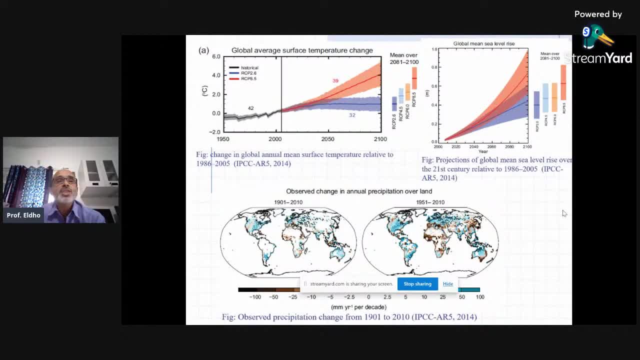 So which is we call it the surface negative concentration pathways, So RCPs, So generally, so the best possibility is 2.6.. And then, so the current way it is continuing, then it can be RCP 4.5.. 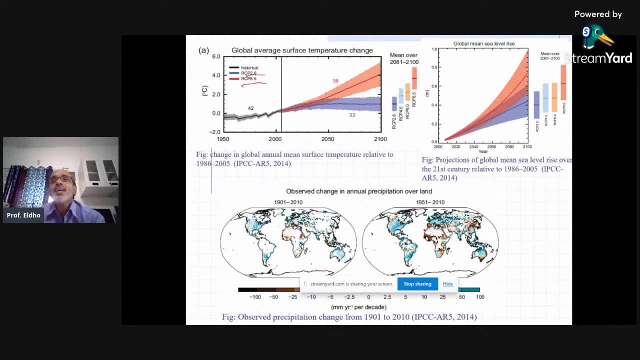 And extreme condition is 8.5.. So if you look into, mainly say, some of the issues, as I mentioned, say the daily climate change, what is happening which we can feel or we can observe. So one is the temperature change. 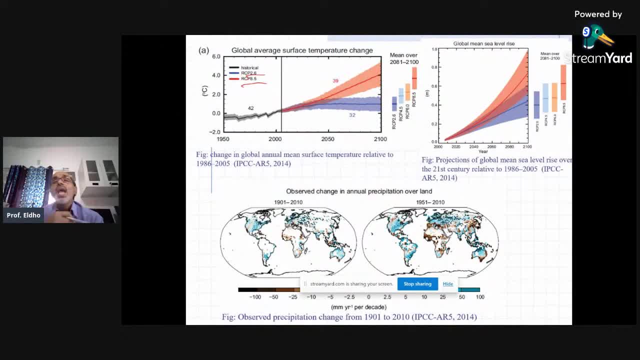 Then second one is the precipitation change or later issues, And then third one is the sea level rise. So all this comes together, Then you can see that. So that is what we are going to discuss in terms of hydrology, especially hydrology's constraints. 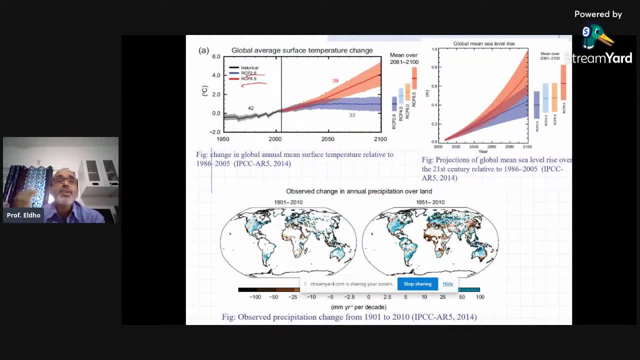 How it is going to affect the hydrology And then especially river basin scale, hydrology's constraints. So as you can see here in RCP 8.6, it can be. upon increase it can go beyond 3 degrees centigrade if it is going to RCP 8.5.. 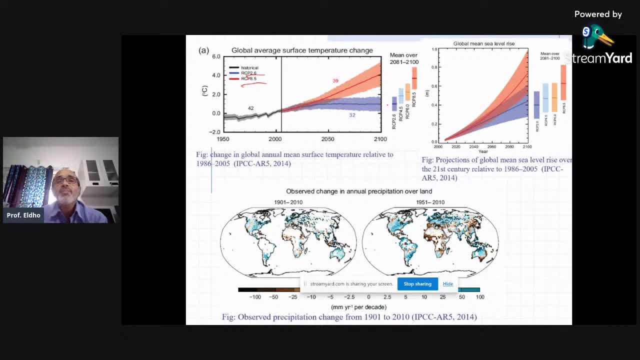 So, but if it is 2.6, then it will be say we can pull down to below 1 degrees centigrade, But if the same trend, current trend, goes, it can be RCP 4.5.. 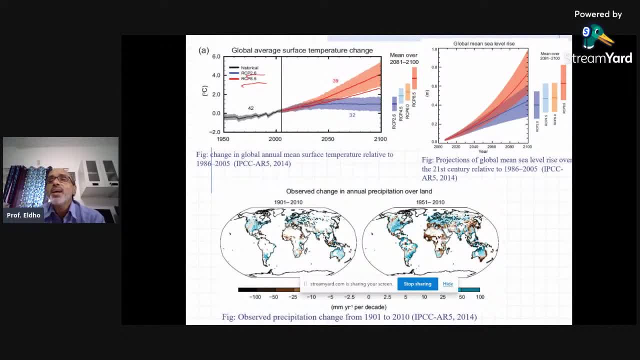 So that will be in between these. So that is what is generally the way, The way we analyze. So here you can see that correspondingly, as projected by the IPCC, the global mean sea level rise. So you can see that if you study from, say, 2000 onwards. 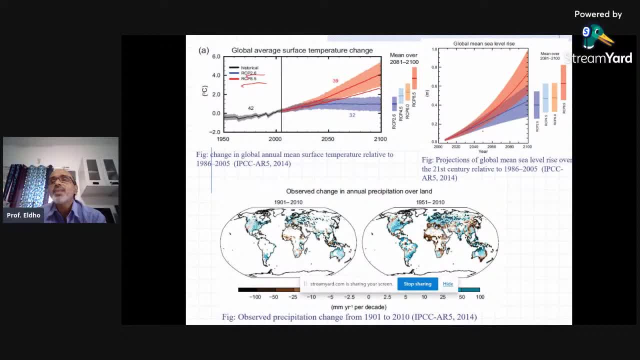 So what is happening? you can see there is a trench in the sea level rise. So here you can see what is happening. now, say, 2020.. And then you can see that it is with respect to RCP 8.5,. this line: 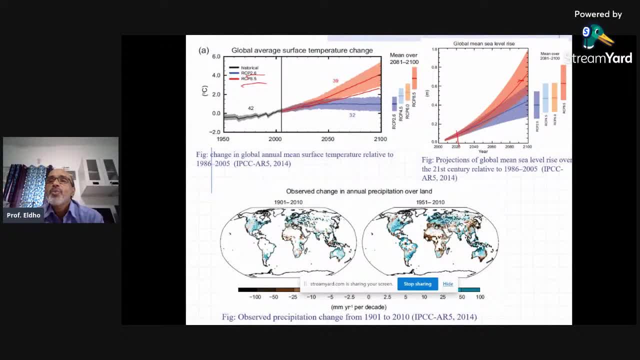 And then this is RCP 4.5. And then below you can see that RCP 2.6.. But what we say generally in this kind of assessment we are much more than about RCP 4.5 and 8.5 and the corresponding projections. 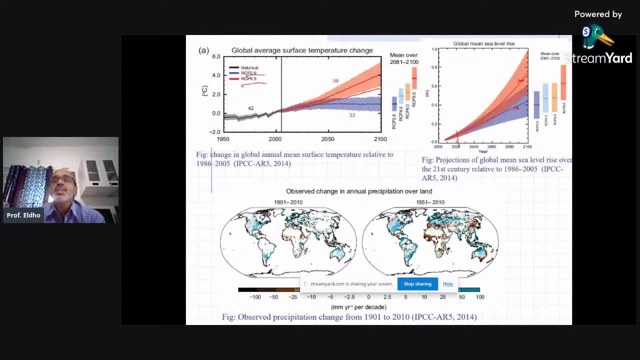 So now that is about the sea level rise. So you can see that, say, even last few decades already, say 30 centimeter to above or above the sea level rise Or above the mean sea level rise is observed. 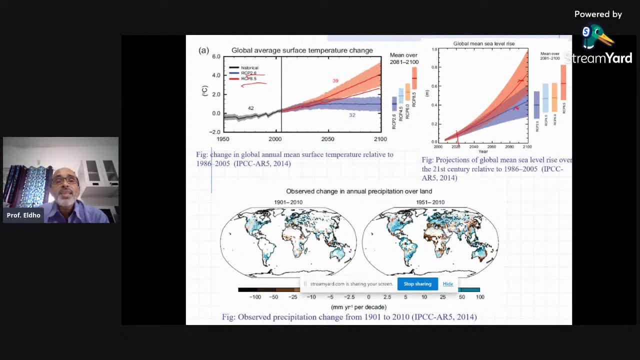 And that is already reported by many researchers. And then next one is change in annual precipitation over the land. So you can see that there is huge changes are observed. So here this shows the observed precipitation change from 1901 to 2010 as per IPCC airfare report. 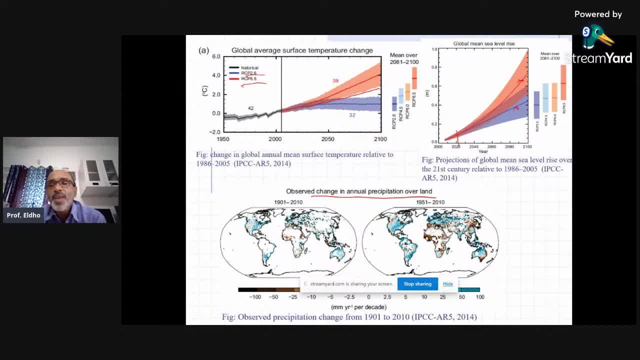 So you can see that what is happening. Some locations it is same, Increasing rainfall is increasing, Some locations it is decreasing. So that kind of trends, we can see what is happening. as far as the precipitation- annual precipitation over land is concerned, 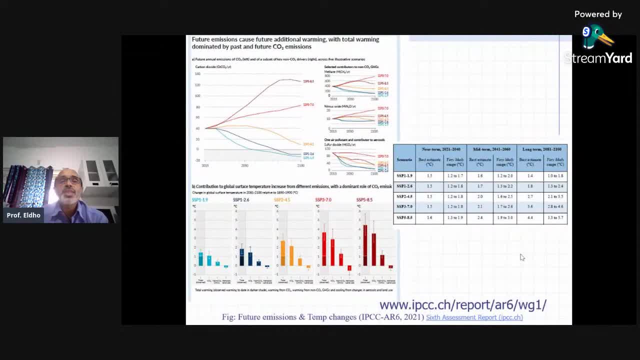 So, as I mentioned, the last few weeks, we are discussing about the IPCC reports, AR6 reports, CMIP6 reports. So here the details are there. These are available now in their websites. So here you can see that future emissions cost future additional warming, with the total warming dominant by past and future carbon dioxide. 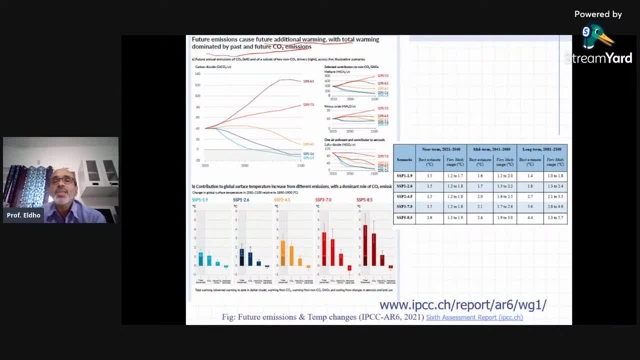 So you can see that in this now current assessment, as per current assessment report, instead of RCP, So the IPCC is putting as the shared socioeconomic pathway So the SSP, So here SSP 1, 1.9, SSP 1, 2.6.. 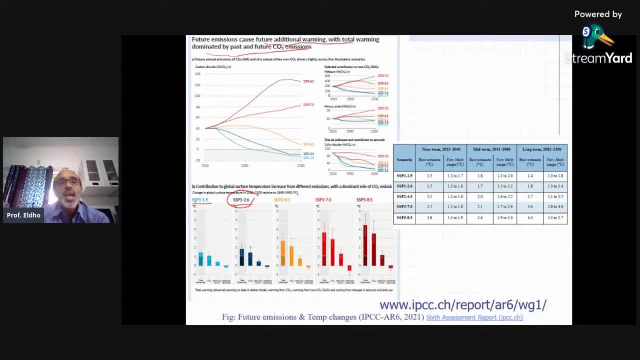 So this is what is related to RCP 2.6. And then SSP 4.5. Almost similar to RCP 4.5. And then this is similar to RCP 6 or 7 between that. And then this is 8.5, the severe condition. 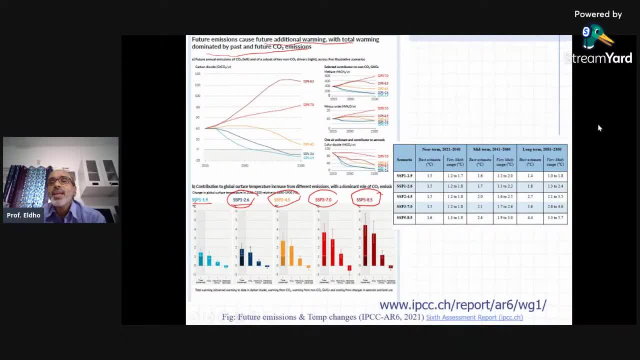 SSP 5, 8.5.. So, correspondingly, what can happen in the near future, up to 2040, 2060 in the future, long-term future? What are the temperature changes Also reported, as you can see here in the IPCC report? 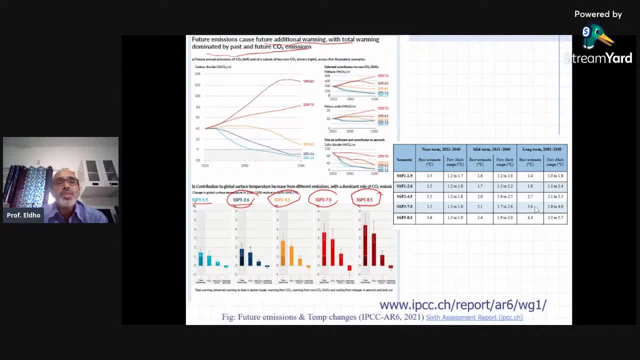 So here, So here, the contribution to global surface temperature increase from different emissions with a dominant roll-off. So you can see that this is a total change. And then the second one is: this is due to carbon dioxide. So that is. 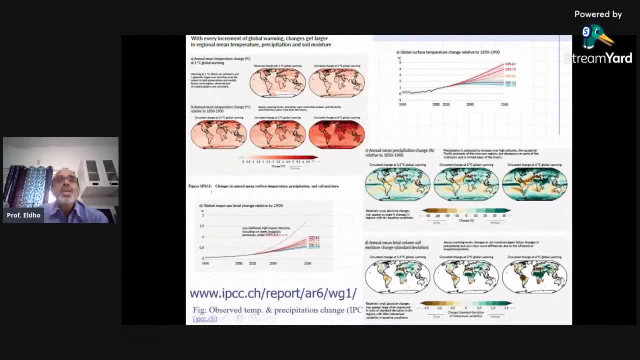 You can see all these details available in this website. So now, as we are discussing about hydrology, So we are mainly bothered about the global surface temperature, And then we look for the annual, The changes with respect to temperature and the precipitation. 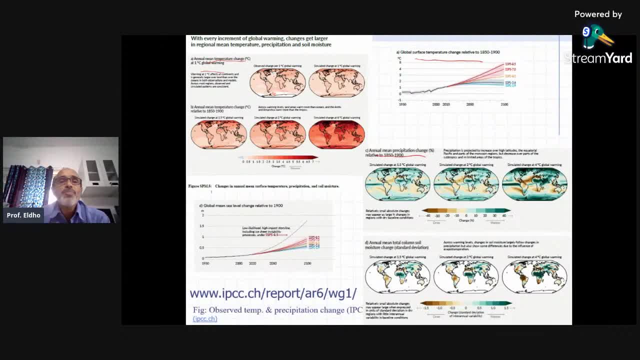 So, as per the CMIP 6 reports or AR5 reports, you can see that when we look into 1850 to 1900, 1,900. And then correspondingly similar to change for 2 degrees centigrade of global warming. 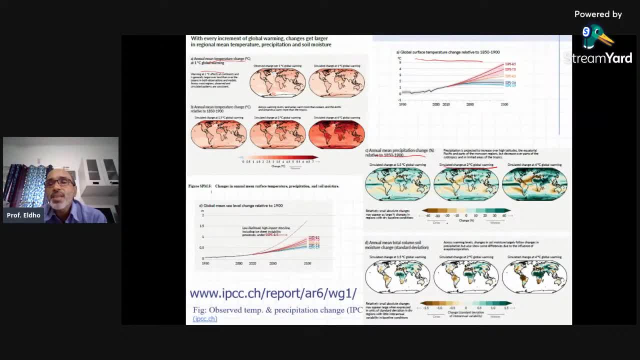 What are the changes possible related to the precipitation? you can see So most areas It is as per this current assessment report. There is a possibility of more precipitation, as you can see, if the temperature is going for 2 degrees rising- And this is the situation- by 2100.. 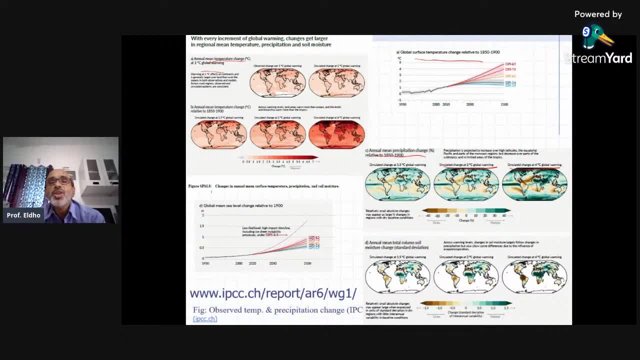 And then a similar to changes with respect to 4 degrees centigrade with respect to what is happening with respect to 1900.. So then, annual mean water, soil moisture. accordingly, all the changes will be happening. So that is why it is so important that we need to study all these aspects. 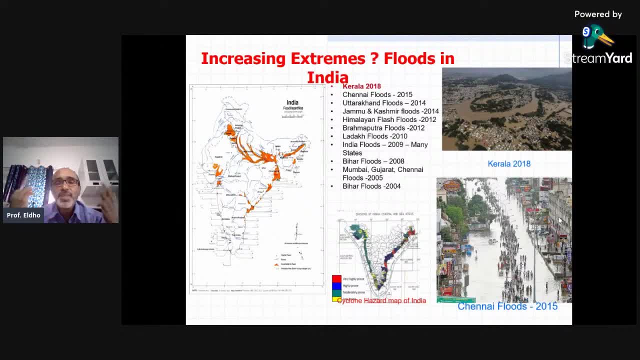 So that is about the climate and climate change and what are the possible impacts. So coming back to our topic, So on hydrology, what are the impacts on hydrology? So that is mainly our topic. So here last few years say, for example, India is concerned. 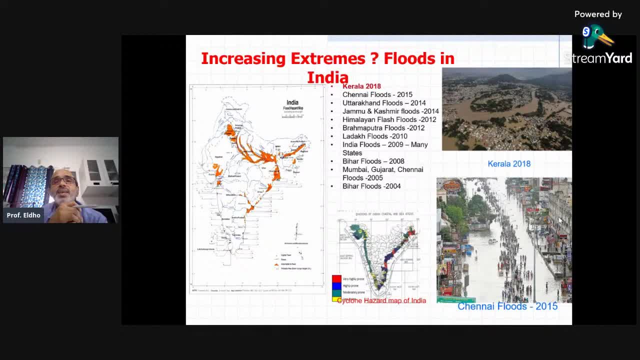 We can see that in every year we can see severe flooding in one or another part of the country. So for example, say, starting from Bihar 2004,, then Mumbai 2005.. So like that in Bihar and all places. 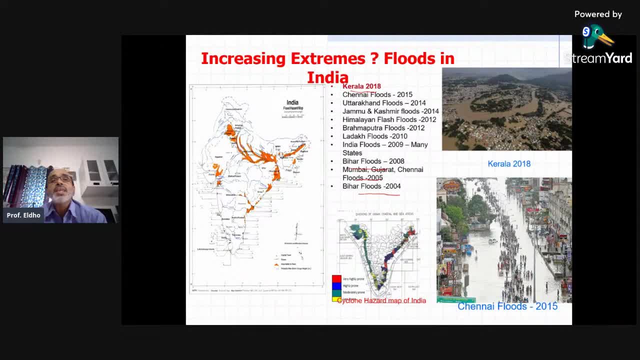 The latest, the last one, I mean 2018, it was very severe flooding. You can see this photo from Kerala, 2018.. And this year also, we have seen flooding in Bihar and other areas. So that way, the question is whether this increasing extremes, whether this is only due to climate change or due to climate change and land use, land cover changes. 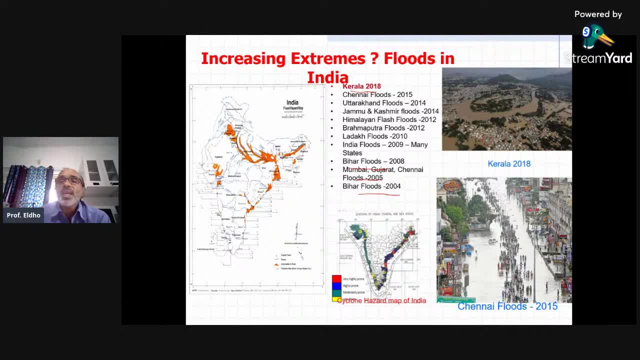 All these things we need to assess. We need to assess appropriately to see that say how it is happening and what are the causes and what are the way And we can say how much impacts are there and then what kind of mitigation measures are possible. 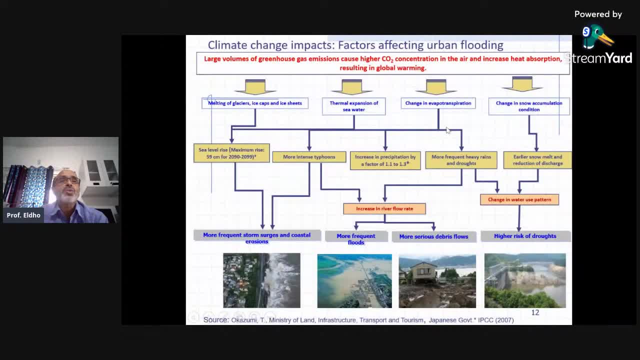 So that is why, as far as hydrology is concerned, we need to look into. So, coming back to the climate change impacts, factors affecting, say, for example, as I mentioned, two important aspects. One is flooding. hydrology is concerned. 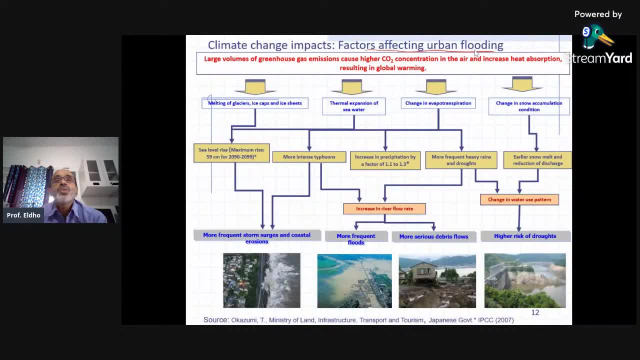 And another one is possibilities: Droughts or later conditions. So here, large volumes of greenhouse gas emissions, as we have already seen earlier. So melting of glaciers, thermal expansion, then changing of vapor transmission, change in snow accumulation condition. 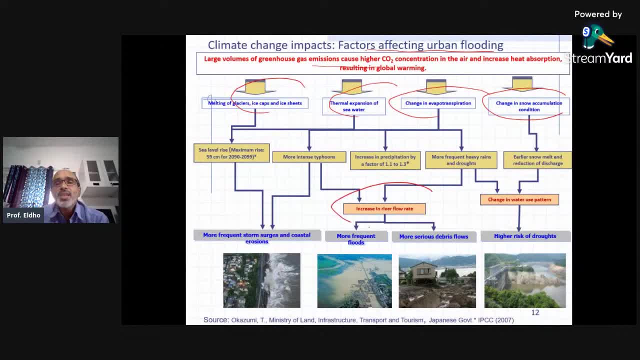 All those things happens And then there can be increase in river flow rate, So then change in water use pattern also takes place. So that way you can see that what will be the consequences will be more frequent storm surges and coastal erosion. 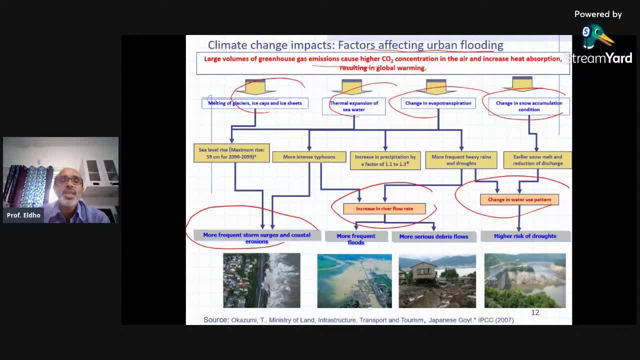 So when all the sea level is also simultaneously rising, then we can have more frequent floods, more serious landslides or debris flows And then, of course, as you can see that what we have, all the studies shows that whenever precipitation happens, it happens for, say, short duration and high, intense rainfall. 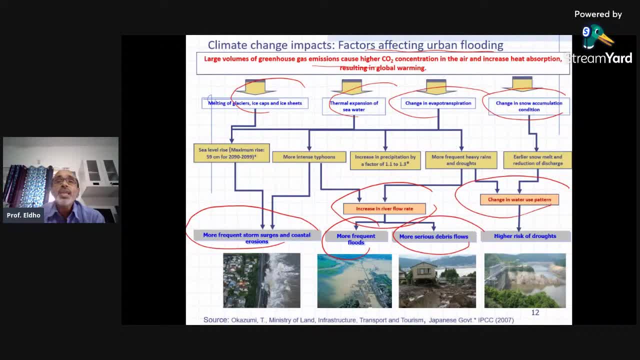 So that is the cause of flooding And afterwards there is a yield period And that is the high risk of droughts, So droughts possibilities also increasing. So these are the main observations as far as all these studies are concerned. 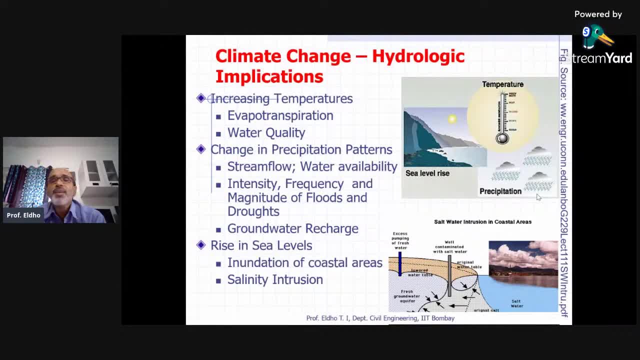 So now coming back to hydrology, since that is, our main emphasis of this lecture is on hydrological implications. So, as I mentioned, increase in temperature means we can have evapotranspiration can increase And then the water quality, say the total water quality- can be affected. 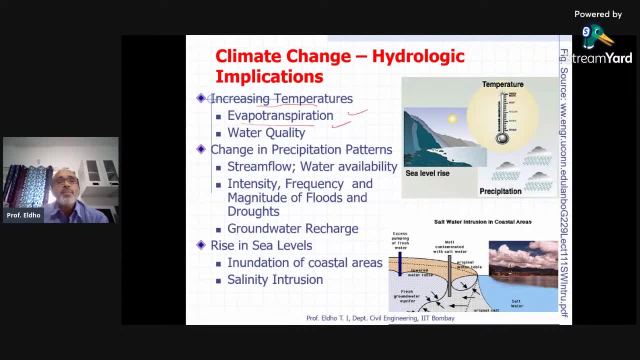 So then, with respect to hydrology, So then with respect to this change in precipitation patterns we can observe, with respect to the total runoff will be affected, The stream flow will be affected And water availability will be affected. So, as I mentioned earlier, so there is, the rainfall intensity will be becoming higher. 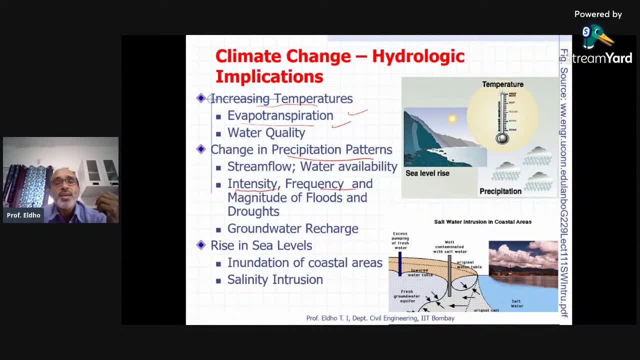 And then frequency and magnitude of floods, and corresponding that will be high. intense rainfall means the frequency and magnitude of floods will increase And then, as I mentioned, whenever precipitation happens, it is happening in a high, intense way And then afterwards so there is no rain. 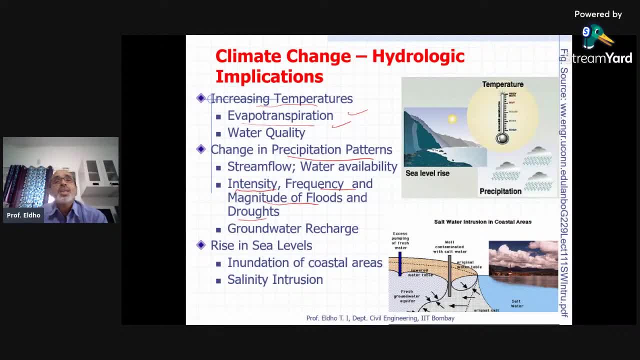 So that can lead to droughts, And then, of course, the implications are concerned. So what can happen is, with respect to all these changes, the groundwater, as I mentioned, a mega source of water, So that will be also affected. 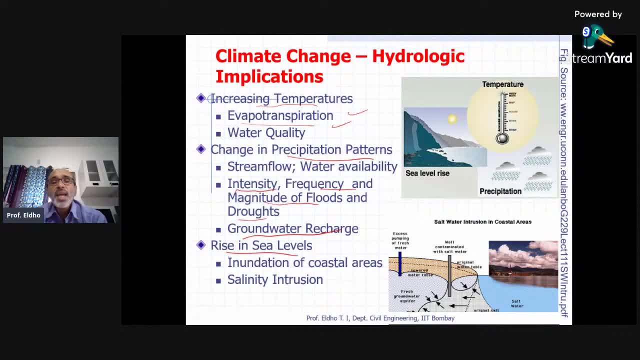 Groundwater recharge will be affected, And then the water quality, And then rise in sea levels can lead to inundation in coastal areas And then also the salinity intrusion. So these are some of the hydrological implications as far as the climate change is concerned. 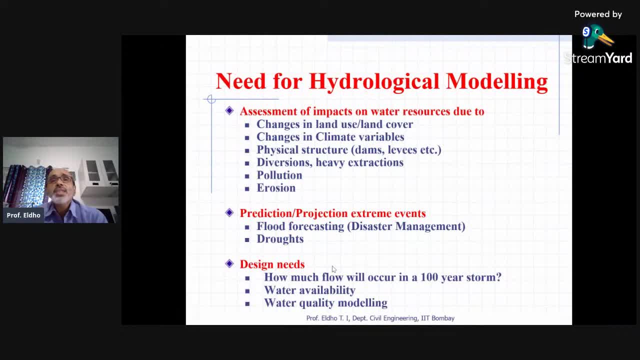 So now coming back to our topic. So here, as I mentioned, the hydrology is so complex, especially river basin escape. hydrology is so complex We need to deal with many, many aspects. So it is not only the uncertainties with respect to the rainfall. 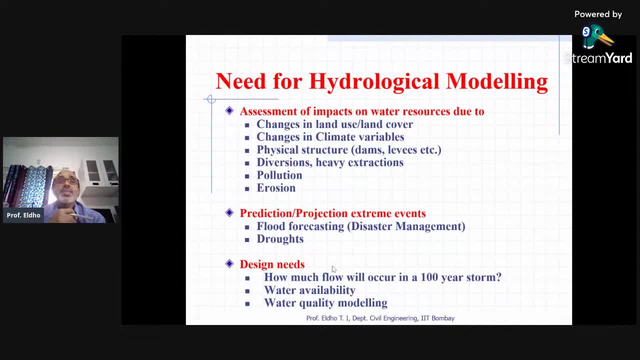 The rainfall, of precipitation and all of the other parameters. But we need to also. we are dealing with the large scale areas. So, for example, say, a river basin, as I mentioned, you can go from, say, a small river basin like 50 square kilometers to again 500,000 square kilometer area. 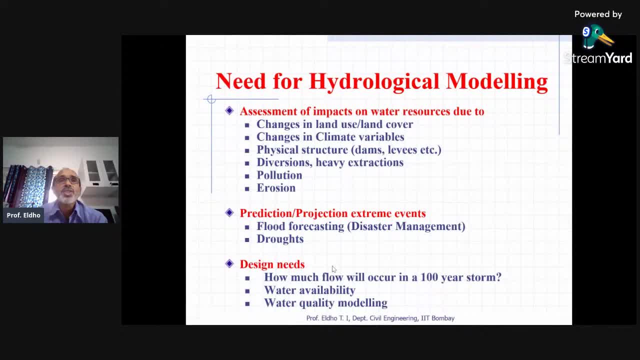 So that way we need to have appropriate models, So it is not only the climate change aspects, like general circulation models. use the temperature variation, The precipitation variations, all those things we can downscale, And then we need to have an appropriate hydrological model so that we can assess what will be happening. 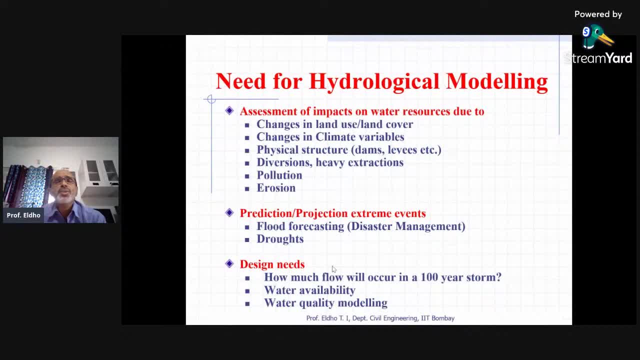 So here the assessment of impacts on water resources due to change in land use, land cover. We need to assess changes in climate variables, physical structures, So, for example, if you are having reservoirs and dams, So then so if the climate change happens. 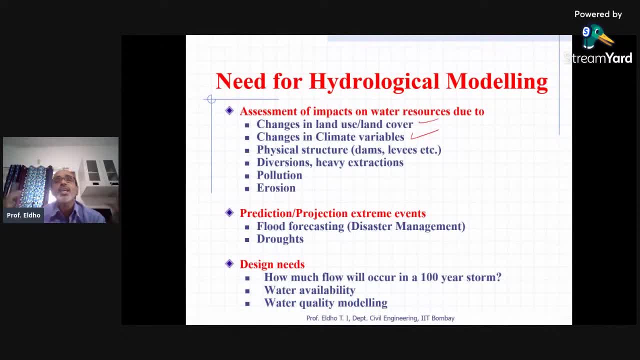 Then the pattern, the hydrological pattern, changes. So what will be the impacts? So all those things we can only assess through hydrological modeling, including diversions, pollutions and erosion, And then say, for example, as I mentioned, we are observing that there is possibility of the increase in precipitation in future. 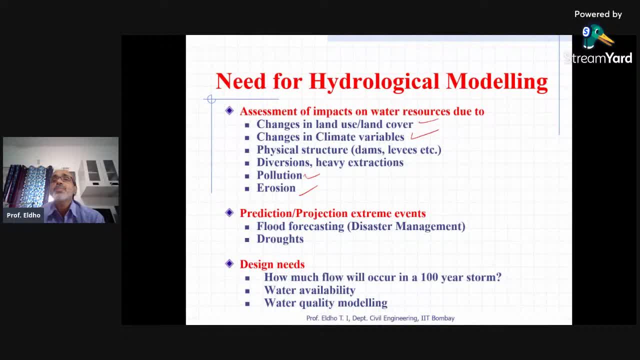 So that way we need to project what kind of extremes are possible, so that, say, some kinds of mitigation measures Or the decision makers can start work on it So that way flood forecasting or disaster management and droughts. So here in all these hydrologies concerns the design needs, how much flow will occur. 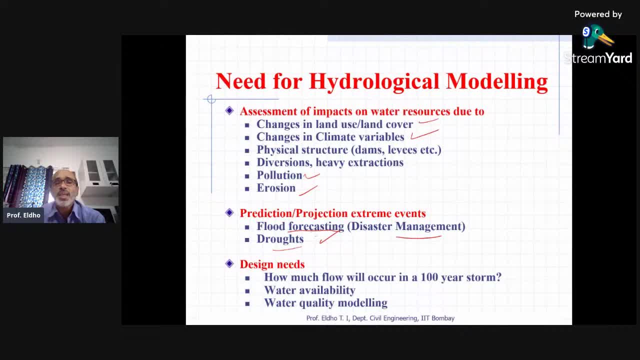 Say, for example, in a 100-year storm what will be say how much flow will take place, And then how it is going to say the flooding or how it can happen, And then how much water is available and water quality. 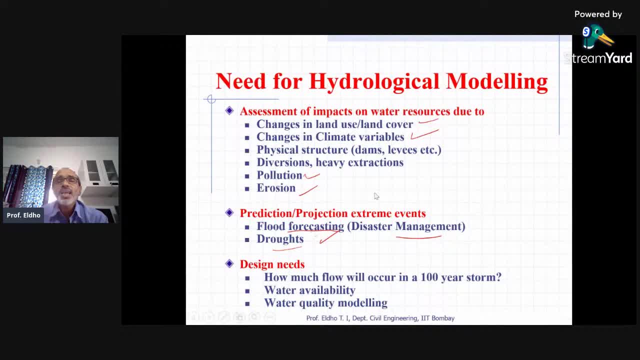 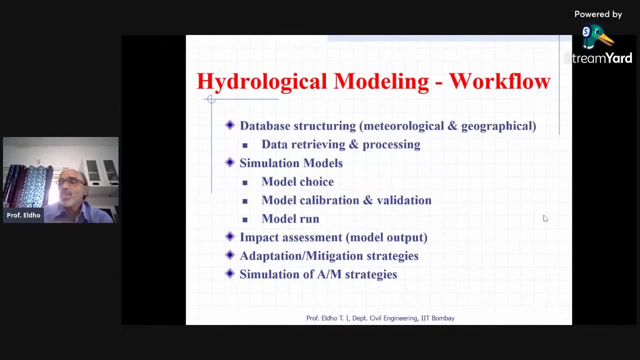 All these aspects we need to study in detail. Am I audible and everything is fine? Hello, Yes, sir, you are audible. Okay, So now if you look into the hydrological modeling is concerned. So, as I mentioned, hydrology is so complex. we need to go on a systematic way. 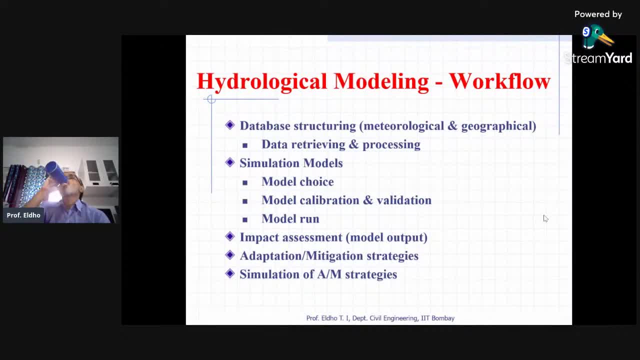 Then only we can get appropriate results. So we need a lot of data. So that is the major challenge as far as hydrological modeling is concerned, Like a database, certain meteorological data, geographical data, Then if we cannot directly collect the data, then say we need to retrieve the data from the available sources. 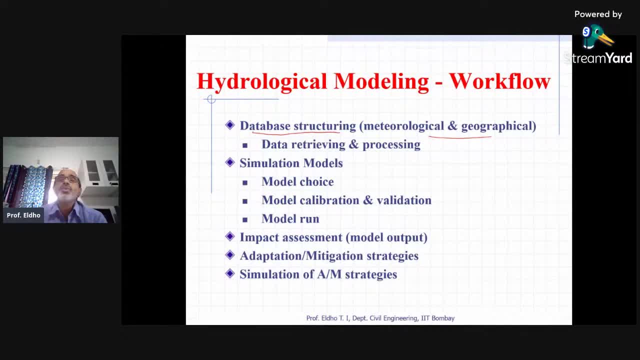 Like you know, we can use satellite data also, including for precipitation or temperature variation, All those things. we can use the satellite data And then we need to retrieve it and process it properly. So that is first aspect is data. 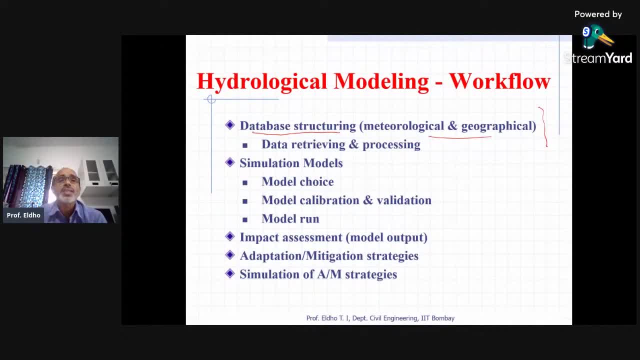 So that is in hydrological modeling is concerned. And then second aspect is the what kind of models we use. So there are plenty of models, So last say, so many beacons, So different types of models have been developed. 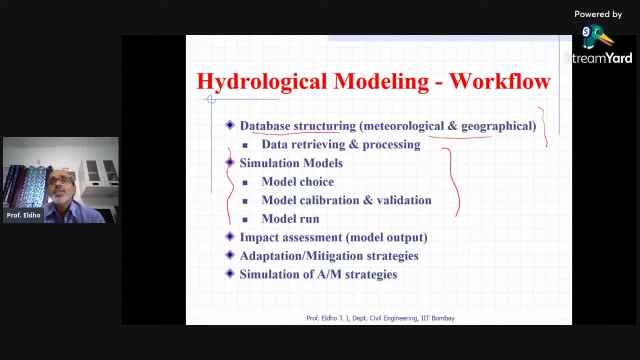 And then we need to choose appropriate model for, say, particular studies is concerned. So, for example, If you are going only for surface runoff, then say like SWAT or some kind of model will be possible. But if you need to also study the groundwater, then say how the interaction between surface water and groundwater takes place. 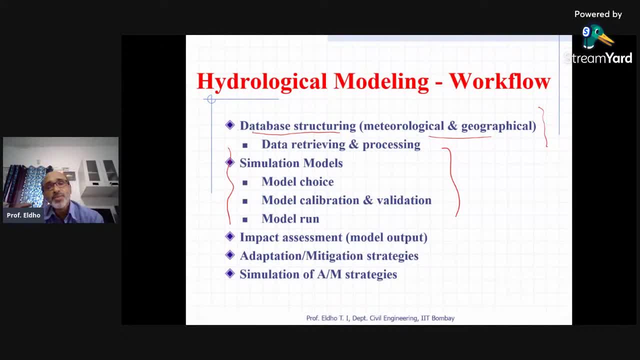 Then we need to choose other models like, say, whatever is connected, SWAT coupled with the mode flow, or that kind of models are needed. So we need to say simulations, hydrological simulation is concerned, We need to look into what is the model choice. 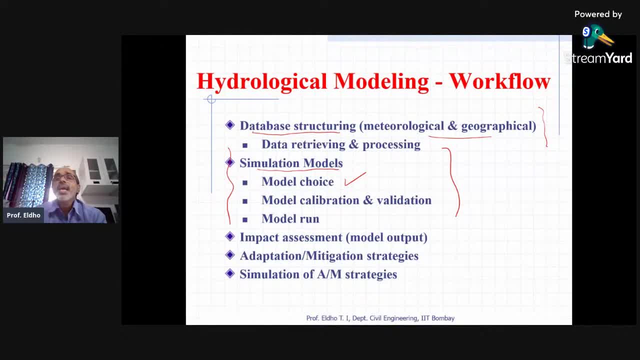 Then, of course. so, as I mentioned, the data is a major issue. So it is not only the climatological data, but the geophysical data, geographical data like the soil data, the land use, land cover data, all these data are needed. 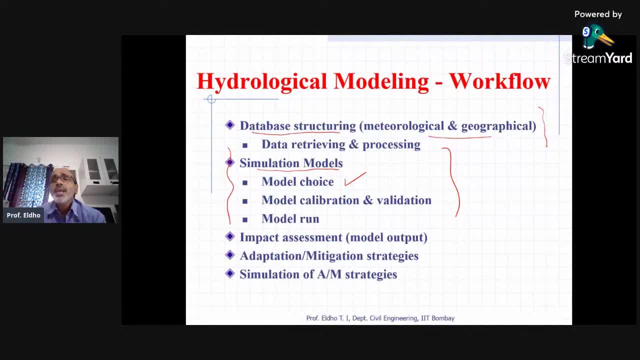 So that way there is a lot of uncertainty will be there. So that way, the appropriate model, the model which we are doing, we need to do the calibration and validation. So on a river basin scale. So, for example, 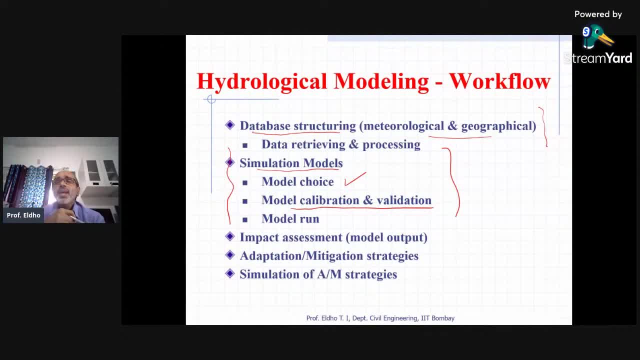 So, for example, to validate hydrological model means we need to collect the runoff data or the, say, the river discharge data And then say we need to run the model and whatever we are the model is given with respect to precipitation, whether it is given in the right way. 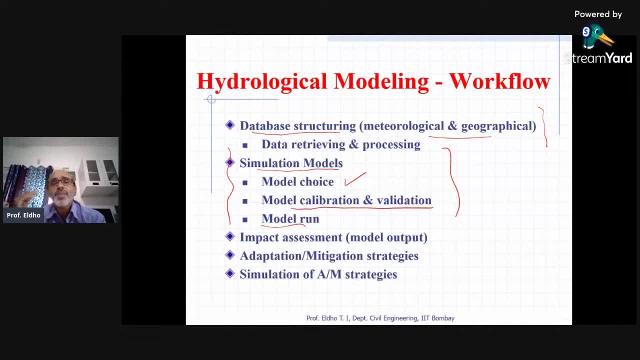 So then, next one is model run, And once we are having appropriate model, then, using the output of the model, we can go for impact assessment, And from that impact assessment We can go for adaptation or mitigation strategies. So that way, the hydrological model is so essential to understand what is happening. 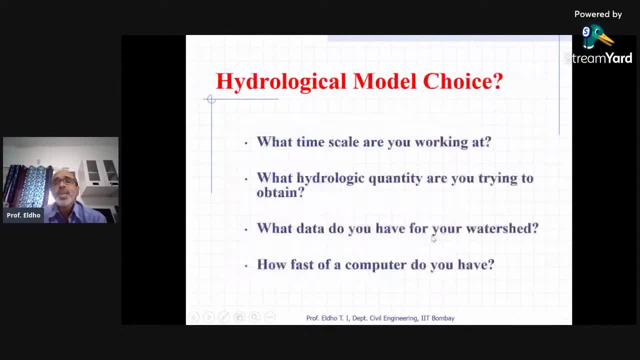 And then so with respect to especially climate change, how we can do this. So that is what we are going to demonstrate through a case study. So now the hydrological model. as I mentioned, a number of models are available. 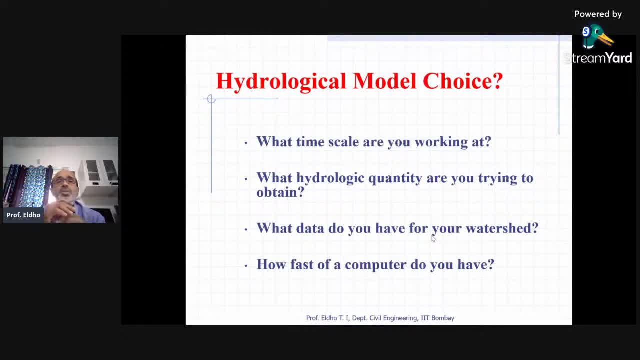 So what kind of model you should choose. So that is some of the important questions coming here: What time scale are you working at? So, whether you are looking for a daily scale model, or like weekly or monthly, or even say, for example, flooding is concerned. 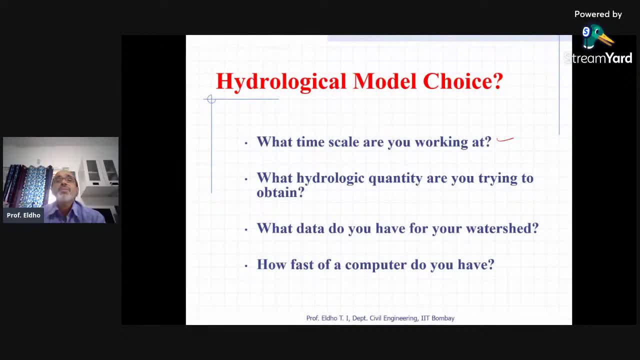 So flooding, if you take, say, monthly or weekly, there is no meaning in floods. Floods happens only for a few days or a few hours. So we need hourly basis simulation and so that we can understand how the flood is propagating and what kind of damages. 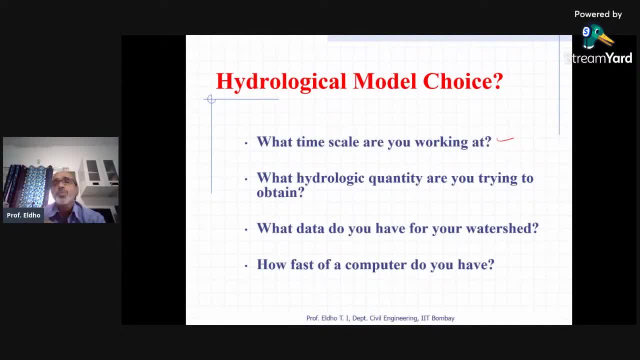 So we have to prepare a flood hazard map And then corresponding the risk assessment to do that. And then, what hydrological quantity are you trying to obtain? So, as I mentioned, whether you need only surface runoff or you want to get to the evapotranspiration: surface runoff, then base flow. 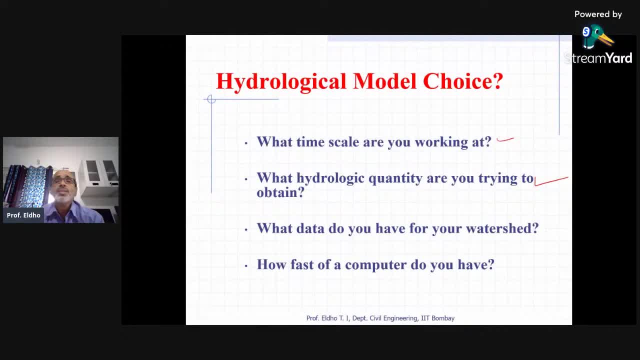 All the aspects are required as far as hydrology is concerned. So that is another question. And then so another important question, as I mentioned: what kind of data you are having, So say, for example, most of the time when you are dealing with large scale areas? 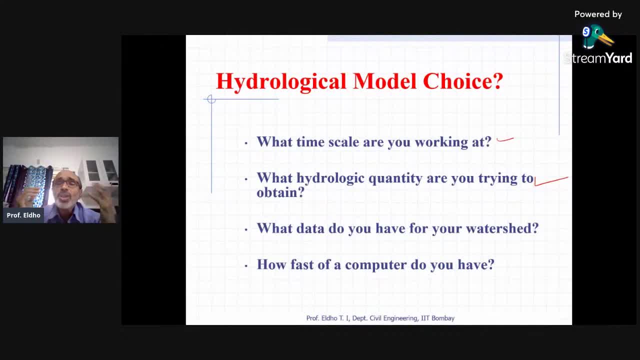 so we need a deep elevation models, then appropriate land use, land cover models and then soil map. All these details are needed. So that is another important question. And then you see that now though computers- fast computers- are nowadays available, even available PCs we can directly use for these kinds of studies. 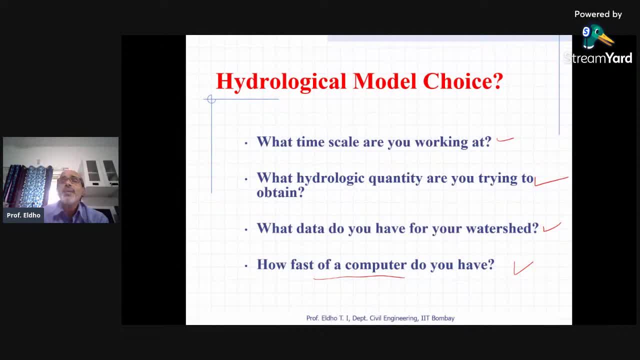 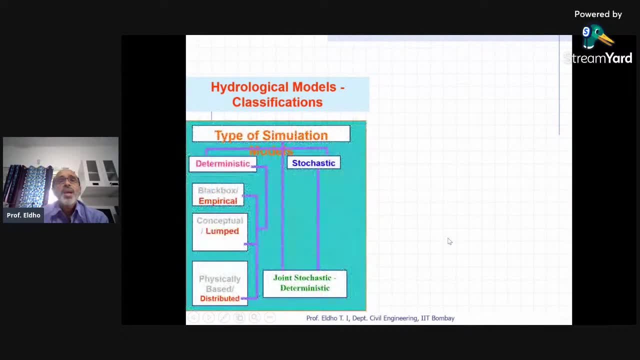 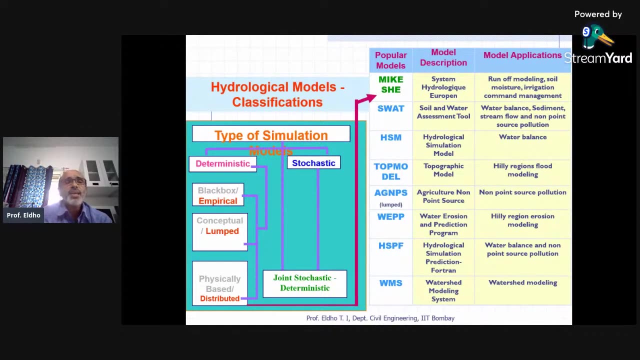 But when we are looking for long-term simulations, we need a high-end computer, like high-performance computing is required, Especially climate changes studies. So now, as I mentioned, there are a number of models that are available, So hydrology models. there is a say like models can be deterministic or empirical or lambda or physically based model. 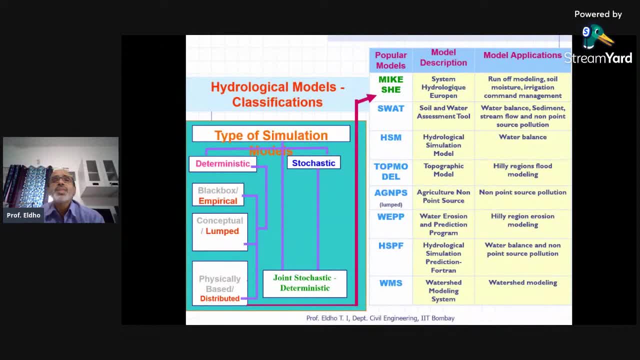 So here are a number of models available I have listed here. So like a distributed model, like a Mice Sheep. So if you are looking for a knob modeling soil moisture irrigation, command management, So there, we need to have such a distributed model. 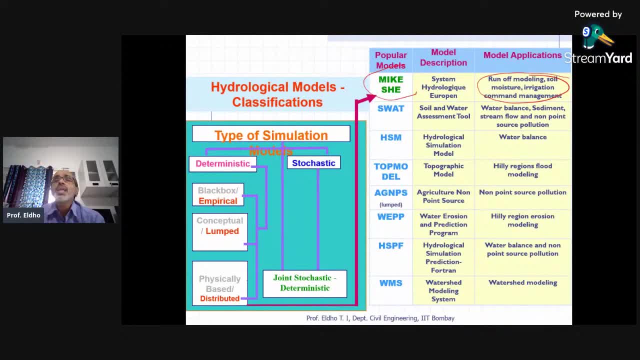 Especially a flood control model. Okay, So that is something is what we are going to study with respect to climate change impacts or whatever it is. So then we need to use Mice Sheep, But that model- Mice Sheep- is concerned, we need to pay for that. 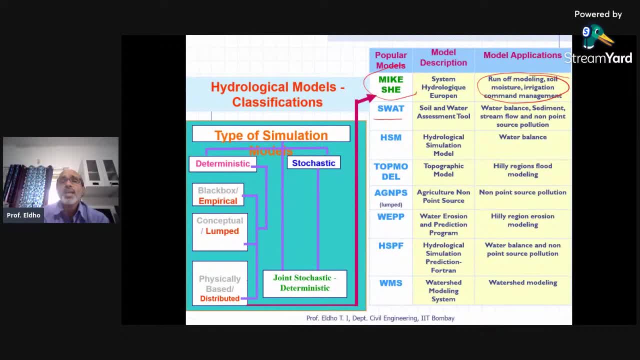 It is say we have to buy the model But open source model like a SWAT we can use. So SWAT is concerned, It is oil water assessment tool. So we will be discussing a case study using SWAT. So here we can get water balance, sediment, then stream flow and non-boiling source pollution. 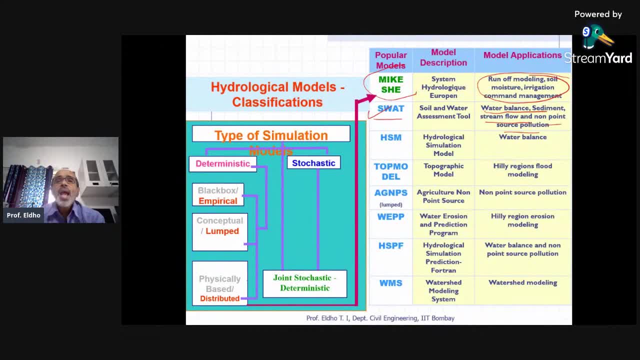 All those aspects we can get through the SWAT model. And then we have other models like hydraulic simulation model, topographic model, agriculture, non-boiling source model, then watershed monitoring systems, So like that. So say we need to decide what are our objectives. 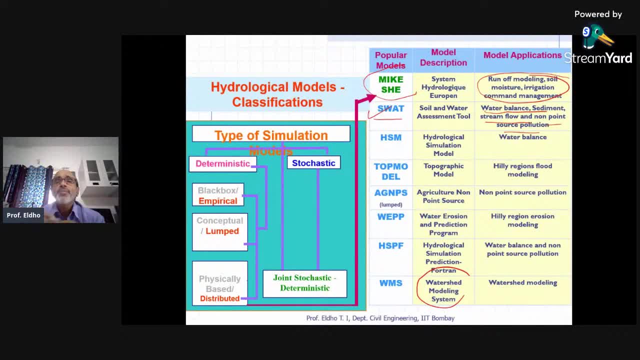 So, accordingly, we need to choose appropriate model. So, for example, if you want to only assess the surface runoff and then its related aspects, then model like SWAT is good enough, Or then we need to go, Or then we need to go for further various aspects for the various components, like irrigation, command management. 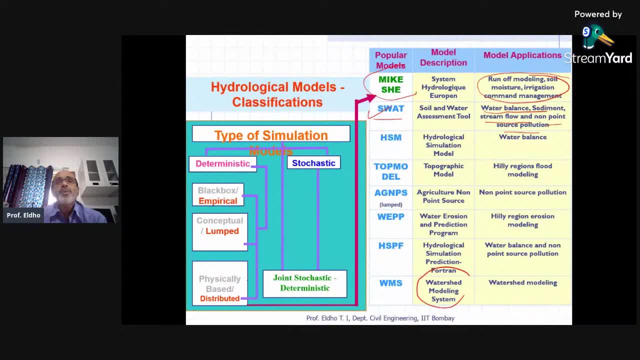 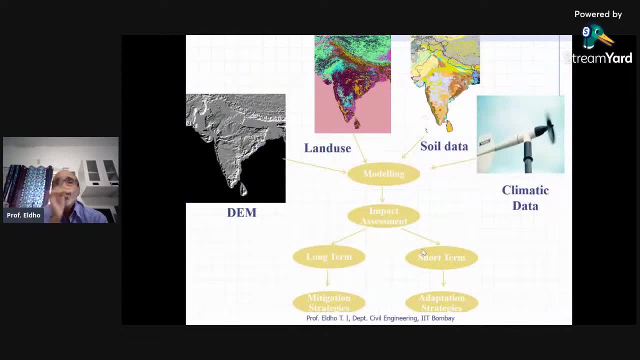 Then all those aspects, Then maybe Mike Shee. So, depending upon the objectives of your study, we need to see a particular model. a hydraulic model is concerned. So, as I mentioned, for any hydraulic model, since we are dealing with a large scale area, so we need to have an appropriate medium. 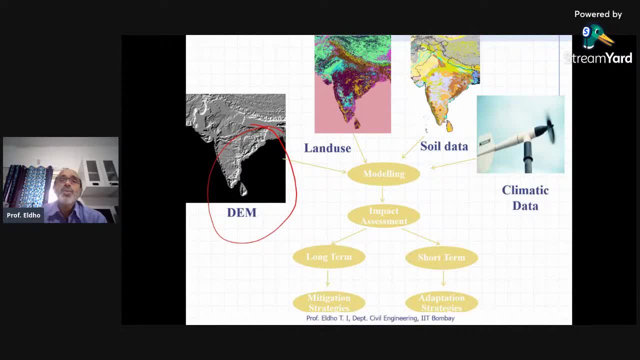 So like this deep elevation model is concerned, So deep elevation model is very important nowadays in all these kinds of modeling. And then, since hydrology depends upon the land use, land flow pattern also, so the land use pattern- we need to get that data is required. 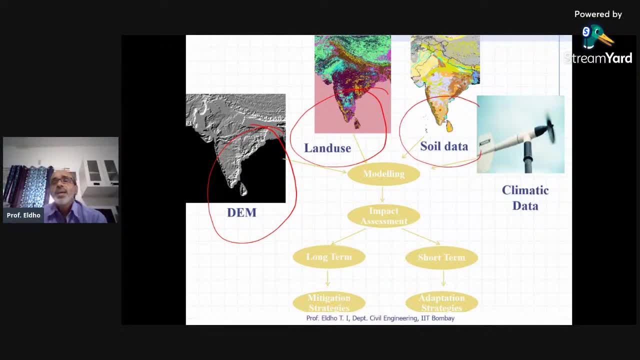 And then, since, say, the hydrology is concerned, precipitation, once it happens it can be evapotranspiration, then the infiltration, all this process takes place. So that way, soil data is very, very important, And then with the climatic data, so these all will be dealing to the, so we can develop. using all this data, a hydrological model can be developed. 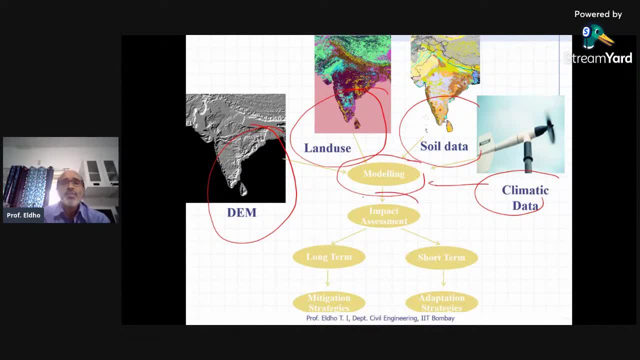 And then we can go for impact assessment: what is happening, So the impacts can be whether it is long-term impact or short-term impact, And then, accordingly, we can go for mitigation strategies for long-term, And then short-term means- immediately we need to- what kind of adaptation strategies are required? 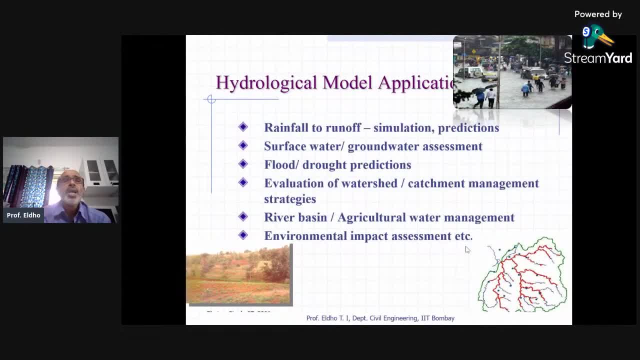 So that way we need to look into. So now coming back to hydrological model applications, So there are a number of applications, So rainfall models, like a simulation prediction, then surface water, groundwater assessment, flood-drought predictions, evaluation of watershed catchment management. 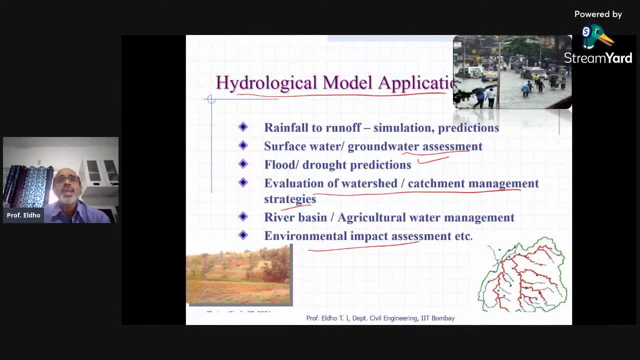 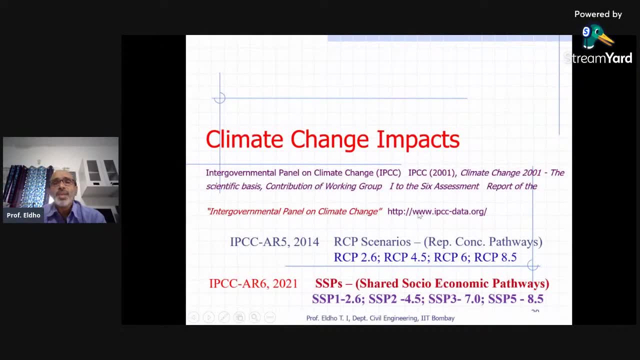 So like that, including environment impact assessments- we can do using the hydrological models. So now we are coming back, So now we are going to see how we can get to the climate change impacts, say as far as the hydrological models. 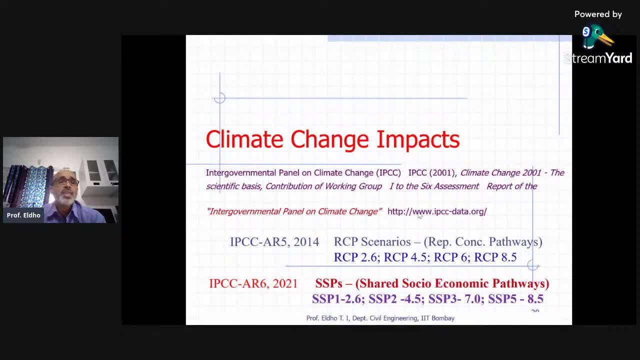 As far as the hydrological models is concerned, especially on a river basin scale. that is the main topic which we are going to demonstrate today. So here, as I already mentioned, so the present study, we will use theardiocnery, especially in the study at RCC 4.5 and RCC 8.5,. 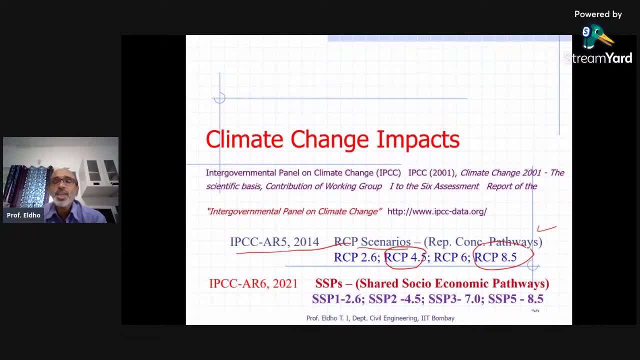 will be the assessment, the scenario of what we will be doing. But, as I mentioned, currently that Robuna IN Ana series report 2021.. So here tried the socio-economic pathways. So you will expect this in RCC this year. 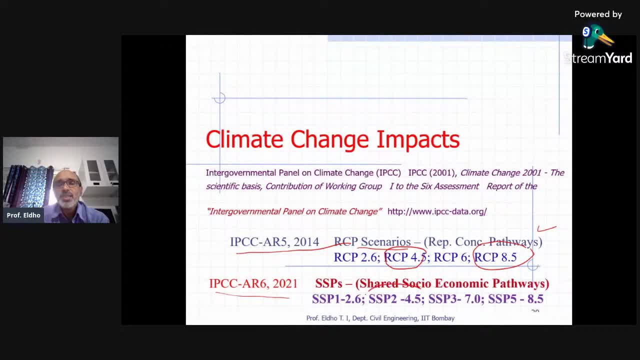 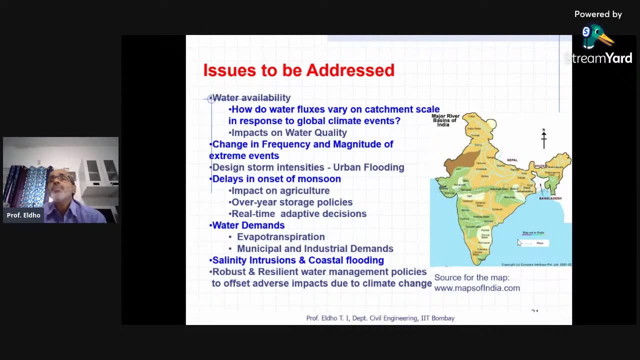 economic pathways. So here correspondingly we can say that this is this and then this. So that way the changes are taking place, but still we are using these RCP scenarios. So when we look into, say, for example, in a country like India, so what are the issues? 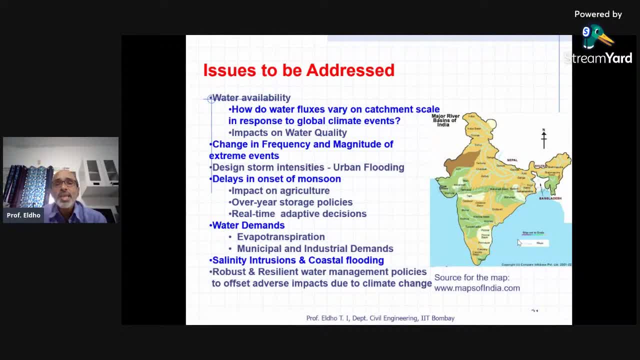 to be addressed. So that is, as a researcher, as a student, as a professional. you may ask: what are the issues? So here are some of the issues I have listed. So we need to see what are the issues. so how the water fluxes vary on catchment scales, especially with respect. 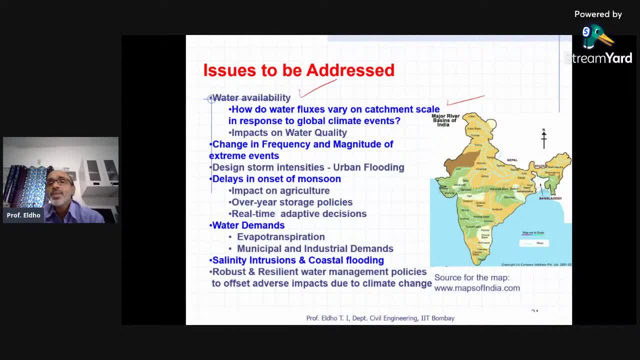 to climate change, what can happen, And then say whether sufficient water will be available on river basin scale so we can see that river basin scale map here. So then we will be observing water quality issues and then say change of frequency or magnitude of extreme events. 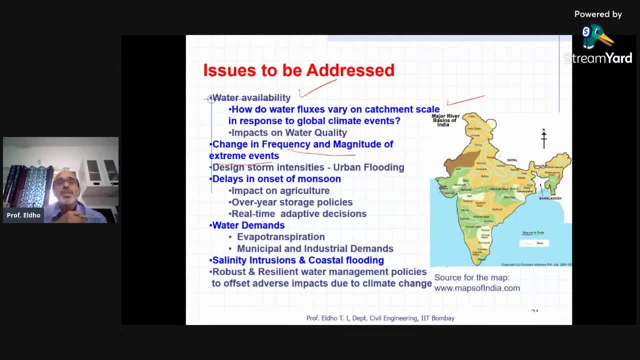 So, as I mentioned the floods and droughts, so what will be the impact as far as the floods and droughts are concerned? And then decisions. You may have a struggle with these kinds of questions, but I'm sure you can get some. 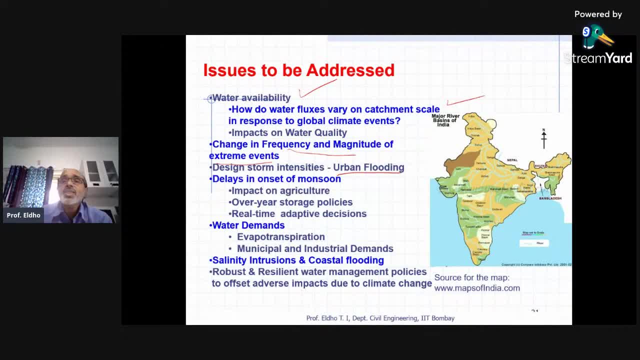 input on what are the challenges. So I would say, if you want to take this into consideration, storm intensities, like urban flooding, especially urban areas, is concerned. so we have to use a very sophisticated model, so we need a high resolution model, so that a small area, what can happen? so 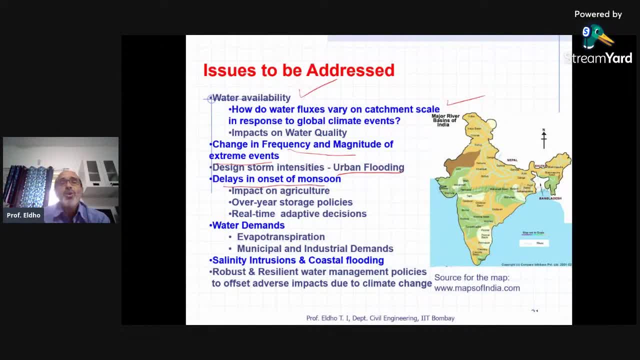 that also we need to study. and then, uh, delays of onset, monsoon, so hydrology is concerned. as you can see, a country like india, or more than 60 or 65 percent farmers, depends upon the monsoon, so we need to see what are the impacts on agriculture. so, uh, so the monsoon say whether. 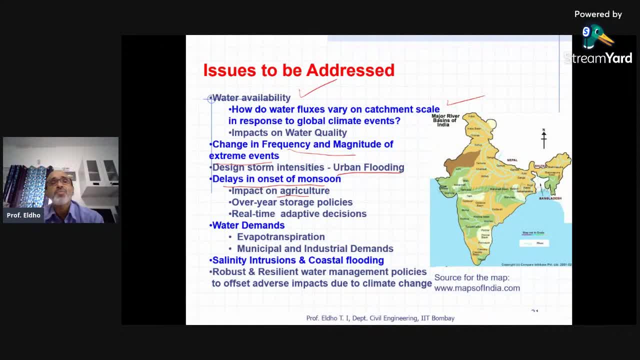 it is starting the onset of monsoon, whether it happens especially june 1st week or whether it is delaying. what will be the impact? and over uh, your storage policies, then real-time adaptive decisions and then, um, the other issues are like water demand. so you know, on a watershed scale, on, 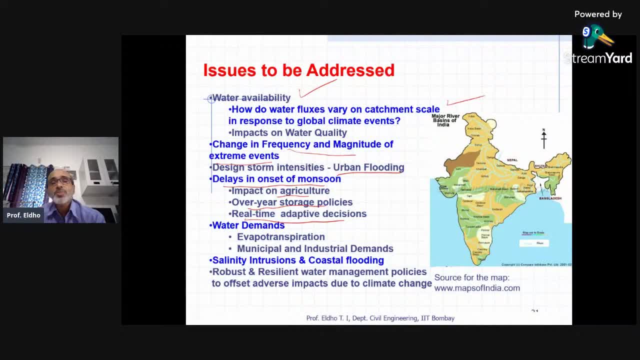 a river basin scale. uh, so you can see that. then evapotranspiration, then municipal and your demands, all the and the any regression demands, all those things we need to meet. and then especially, uh, we have got a very long cost region, so that may. we need to see the salinity. 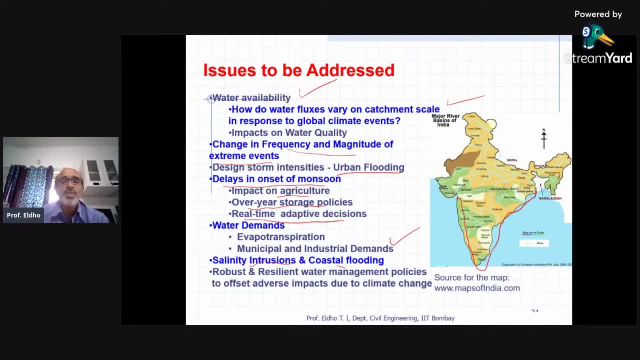 inclusion or cost of flooding. what are the possibilities? so that we need to see and then, so that way the hydraulic impact studies are concerned, we need to have robust and resilience waterman. so so all these studies can lead to robust and resilience water management policies to offset adverse impacts due to the 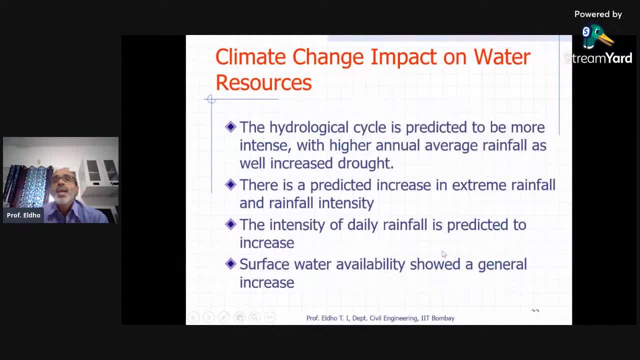 climate change. so that way climate change impact on water resource or hydrology is concerned. so the hydrological. so, as i already mentioned, both the air 5 and air 6 reports indicates, especially in a country like india, the hydraulic cycle is predicted to be more intense, with higher annual 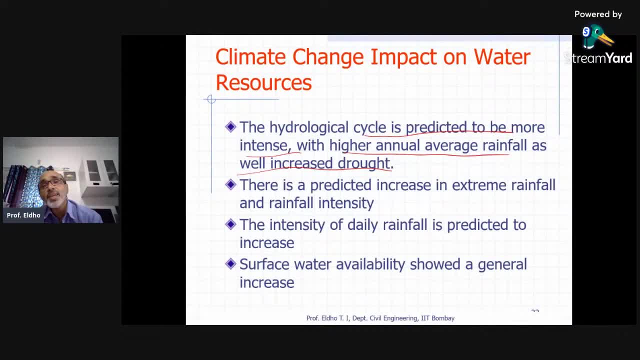 average rainfall as well as increased drought. so, as i mentioned, when rain happens, precipitation happens. it will be high, intense rainfall happens and then afterwards there will be, will not be any. uh, there's a possibility of increased drought also. so there is a predicted increase in extreme rainfall and rainfall intensity and intensity of rainfall is predicted to increase. of that way, 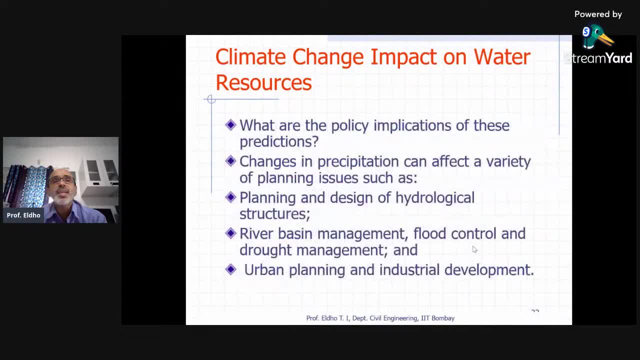 and then surface water availability showed a general increase and then that way, uh, what are the, the, the policies of consent? what are the policy implications of this? all these projections or predictions, the changes in precipitation can affect a variety of planning issues, such as planning and design hydraulic structures, if you have got a dam. 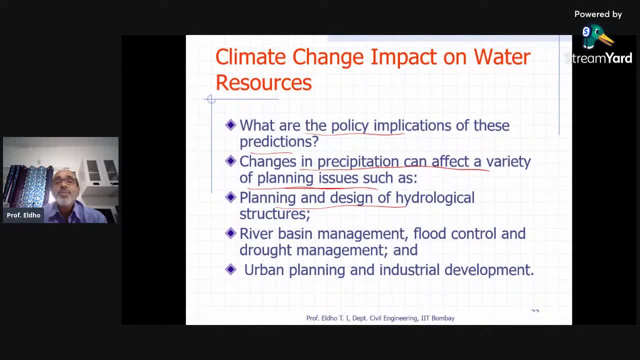 where there is no water then there is no meaning, so but if it is there and heavy rain stage space, it is filling uh so fast and then we cannot use for a long time. then we need to release the water from the reservoir, so that kind of issues, so that the river basin management is very essential for 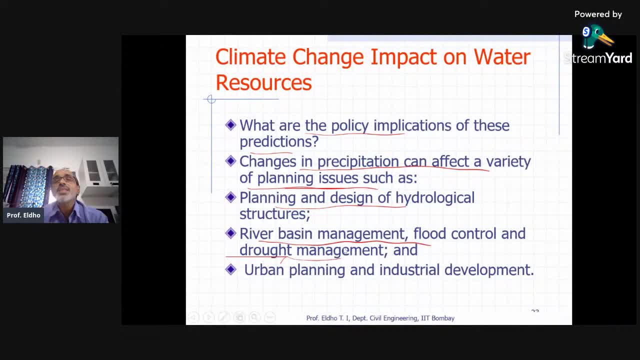 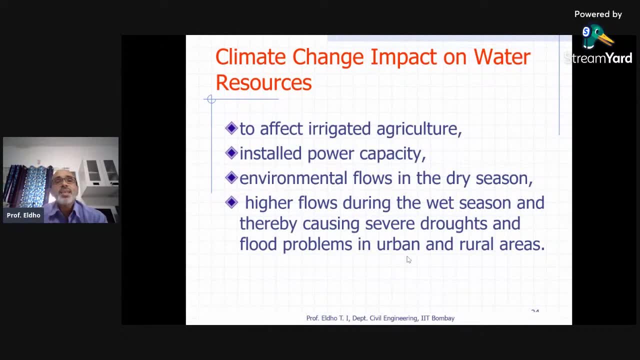 flood control and drought management, and then urban areas concerned. we need to see, and before for urban planning and management is concerned, so we need to see, within this contest, uh the uh also, what will the impact on related agriculture then? uh say, if uh say around 15 percent? uh, in india we produce hydropower, so what will be installed? 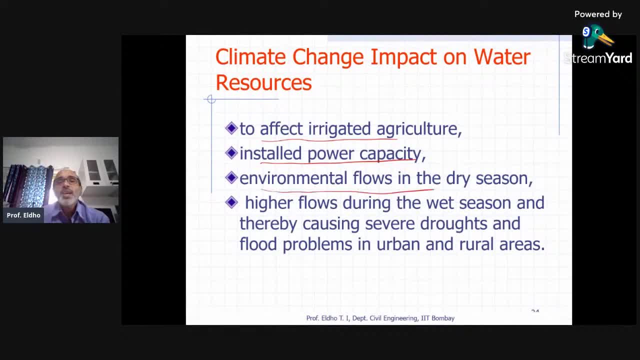 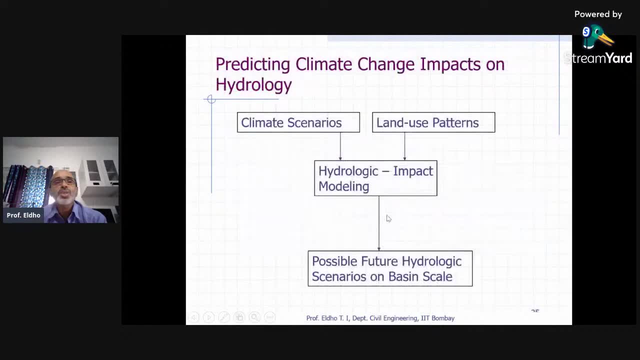 power capacity. what kind of changes can take place then? uh, the environmental flows in the dry season, how it is going to affect then higher flows during the wet season. so that that also we need to study, so that way when we look into the predicting the climate change impacts on hydrology. so we 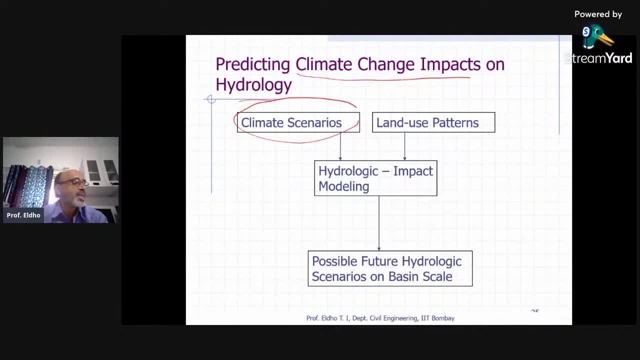 need to see the climate scenarios. as i mentioned, it can be rcp or ssp, whatever we are looking then. uh, then of course, as i mentioned, we are building the land, the, the watershed or a river basin. so what are the changes that can happen? land use pattern? and then we do the hydraulic ring batch. 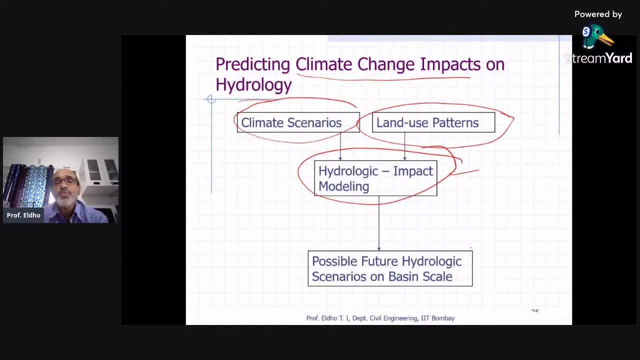 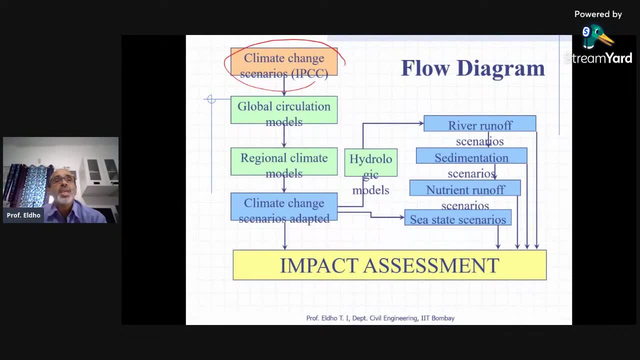 modeling and then from there we get the projections, possible future hydraulic scenarios on a basin scale. so we start with the climate change, with the gcm's, global surface models that we can use it. uh, as you can see here and from there we need to go for, since most of these gcms are 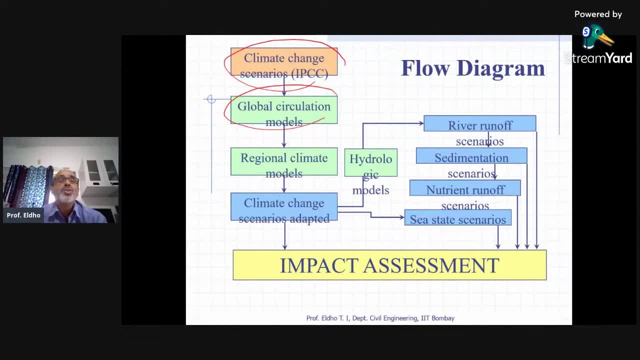 say, 2.5 degree or above resolution, so we need to get to higher resolutions like 0.25 or 0.1 degree uh resolution. we need, especially for your basis scale analysis consent, so we need to go for regional climate models and then climate change scenarios- uh, we can get it, and then uh, as i 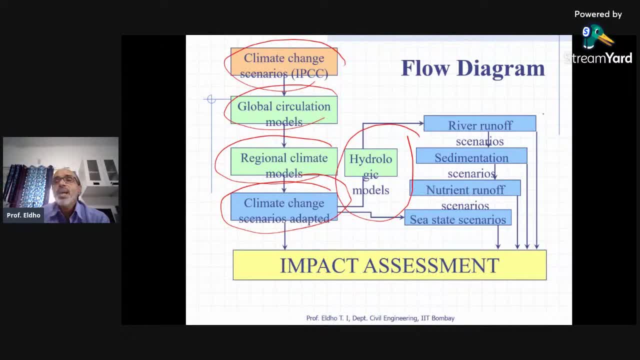 mentioned, we go for hydrological models, so it can be for river runoff scenarios or sedimentation or nutrient runoff or sea state scenarios, all those things we can do. and then we can do the impact assessments. uh, we can do it. so the climate change impact on water? 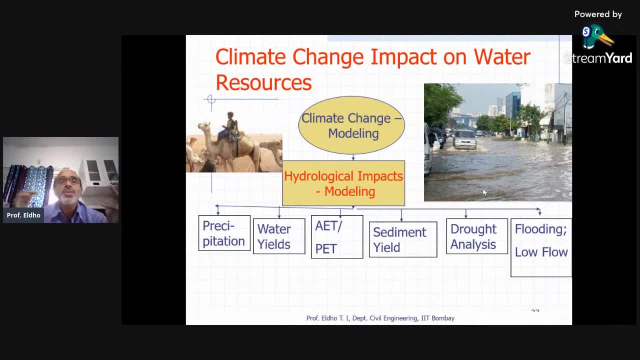 resource, as i mentioned. so we we get all the data and then do the corresponding assessments and then the hydraulic impact modeling. so generally we'll be looking for precipitation, water yields, the changes in the actual evapotranspiration, then sediment deal, drought analysis and then, of course, uh, city level or urban areas for flooding or what will be happening, uh, so 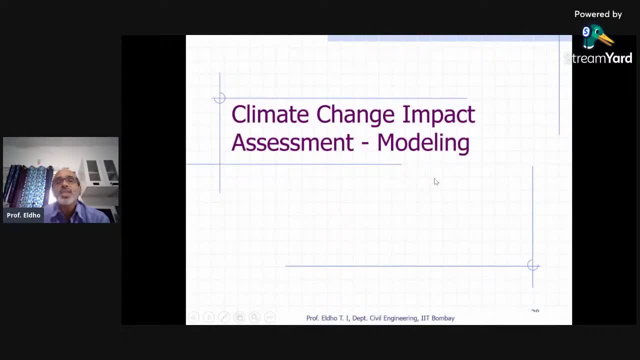 now we are going to discuss further the climate change impact assessment modeling. so, as i mentioned, so am i audible and everything is fine. uh, isaria, yes, sir, yeah, okay, so now. yeah, so now we are going to discuss the climate change impact assessment, so how we use the gcms general. 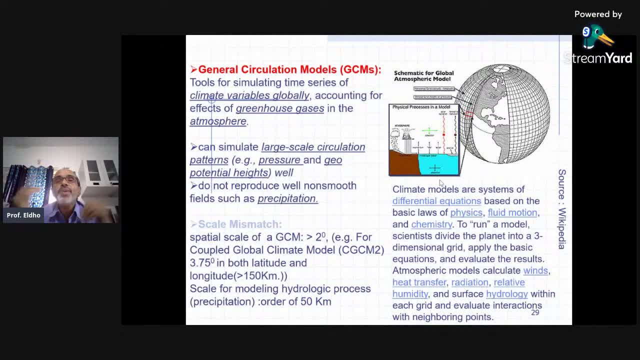 circulation models. so the this is the the best tool we can use for especially the climate change impact as far as uh future is concerned, how it is going to impact. so uh, here, this, uh this, this gcm's. what is developed is accounting for greenhouse gases in the atmosphere that can simulate large scale saturation patterns. you can see a total. 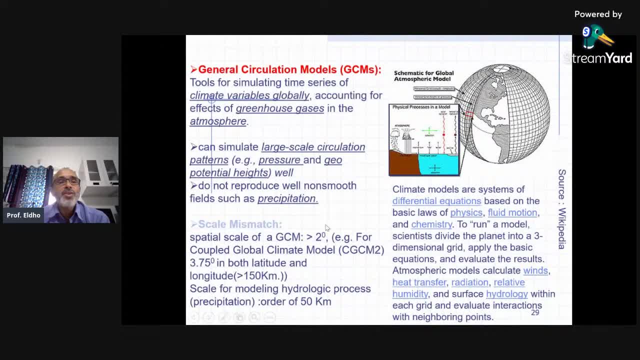 grid device. it can get, so it is. do not produce well non-smooth fields such as precipitation. so there is, as i already mentioned, there is- a scale mismatch. so most of the gcms are more than two degree or above. uh, but um, with hydrologic constraints, we need to come to further. we need a downscale. so climate models: 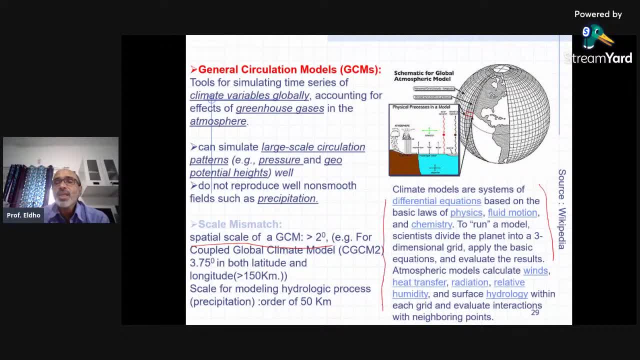 are systems of differential cancel. this anyway, uh, i'm not going to discuss. you can see that the gcms, uh, uh consider all kinds of details like the um, loss of physics, fluid motion, chemistry, and uh, then the bins, heat transfer, radiation. all the aspects are considered. so now uh say, for example, uh, as for air, for report, climate change. 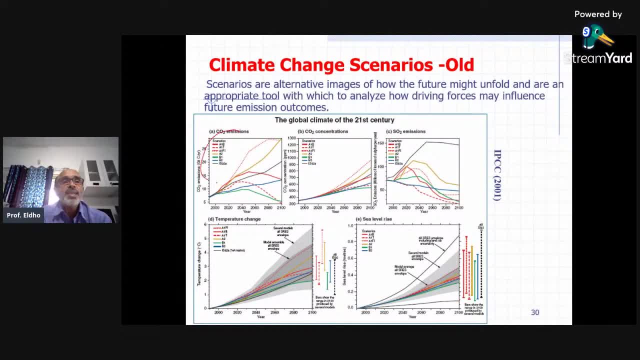 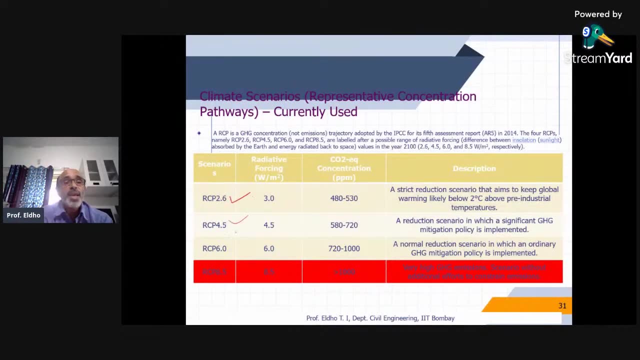 so many of you may be knowing, it was a yeah, when we haven't um, feel like that. they had to be one of these kinds of scenarios. uh, were there as per ipcc 2001 reports. then came the rcp scenario, as i mentioned earlier. so here: 2.6, 4.5, 6, 8.5, so correspondingly description. so here, as i mentioned, 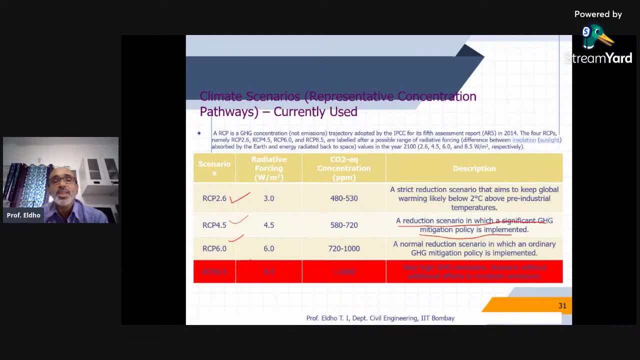 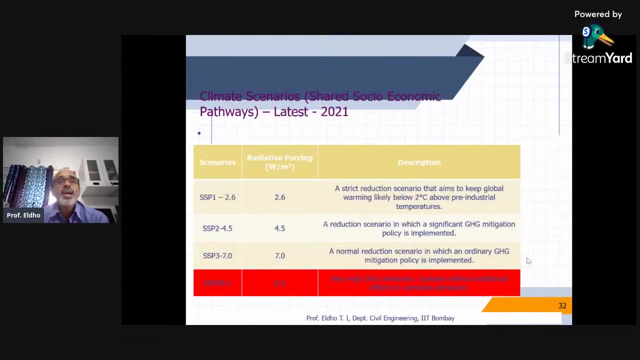 the reduction scenario in the significant gh integration policies implemented, like paris agreement. what has happened in 2018? if we can go to that level, then rcp 4.5 will be valued, but extreme condition is a rcp 8.5, a very high emission scenario. so correspondingly, we have 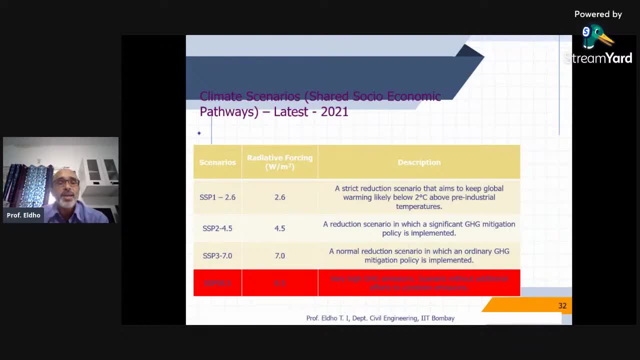 already discussed some. the latest 2021, uh, the the scenarios are with respect to shared socio-economic pathways. so here, say, rcp 4.5, almost very similar to for ssp2, or 4.5 and ssp 8.5. so we will be discussing with respect to rcp 4.5 and 8.5. so now coming to hydraulic impact. 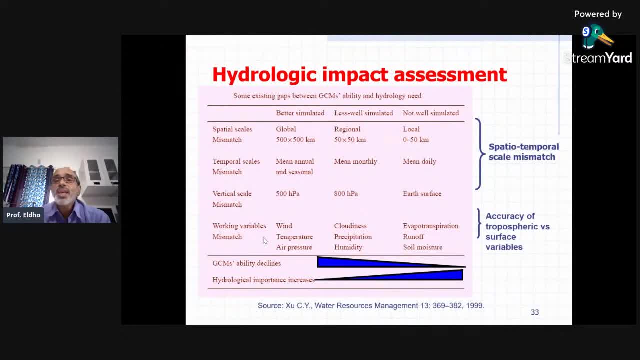 assessment. as i mentioned, scale is always an issue. so here the these gcms are concerned, large scale models are there, so here, but the the gcm's ability declines when he's coming to small scales. so now the hydrological studies are concerned. we need a same 0 to 50 kilometer. 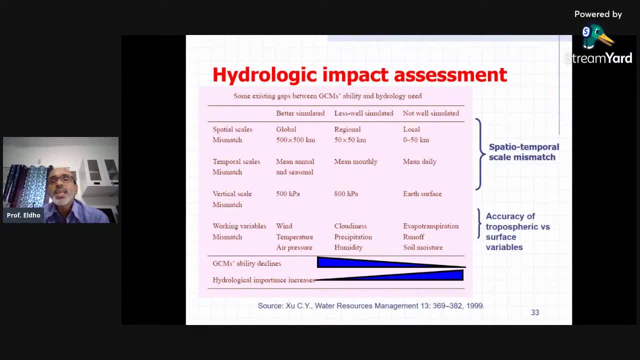 like kind of studies or 0.1 that kind of studies. so that way we need to down scale the data. so gcm savings declines when small areas are concerned, but hydraulic importance highly increase as far as the, the small areas are concerned. so that way we need to go for downscaling. so downscaling, you can see that what can happen is 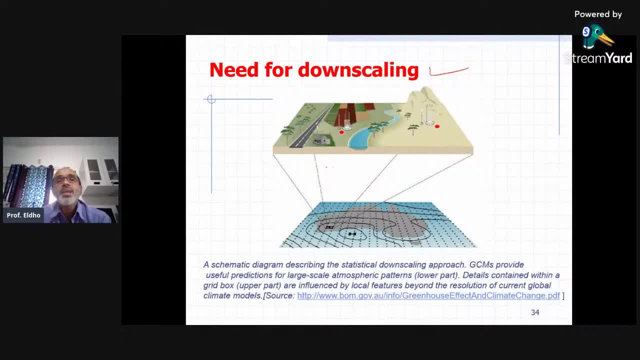 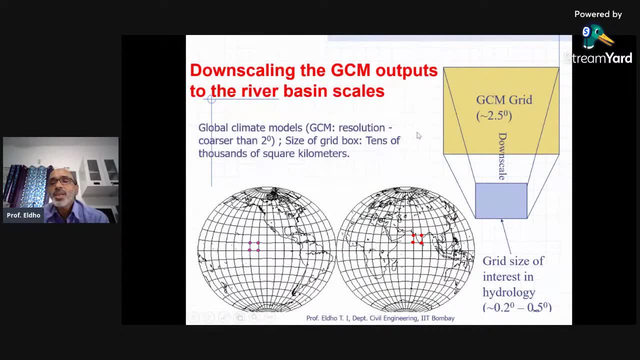 with respect to this grid, we project to the, the area, whichever we are looking for- and the down scaling to the discounting scale. so that means that we are more likely to be low scale. so we can see. So here you can see the grid size: from 2.5 degree to 0.2 degree or 0.1 degree, we have 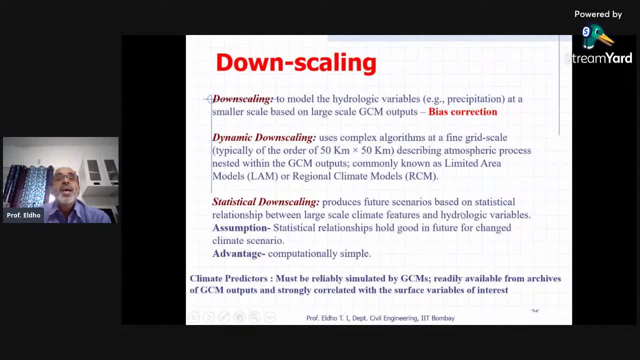 to downscale and then we have to utilize that data. So downscaling is considered. it can be two kinds of downscaling. generally we use one is dynamic downscaling. second one is a statistical downscaling. So what do we do In dynamic downscaling? we use complex final grid and, like regional scale, climate models. 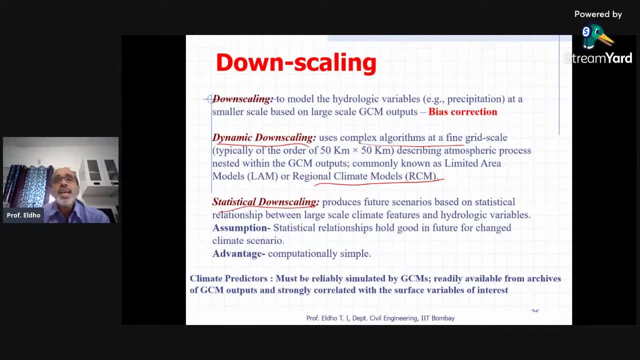 we can make from the GCMs and then we can directly use that data. Statistical downscaling: we are using the past data produced future scenarios based on statistical relationship between large scale climate features and hydrological variables. So your assumption is: statistical relationship holds good in future for change of climate. 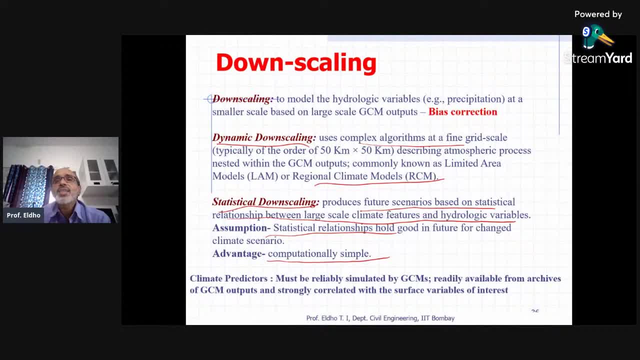 scenario. So here, advantage is that it is computation symbol, but we need a bias correction. So that is very important, since, with respect to past data, So that way important climate predictors. This must be reliably simulated by GCMs readily available from archives. 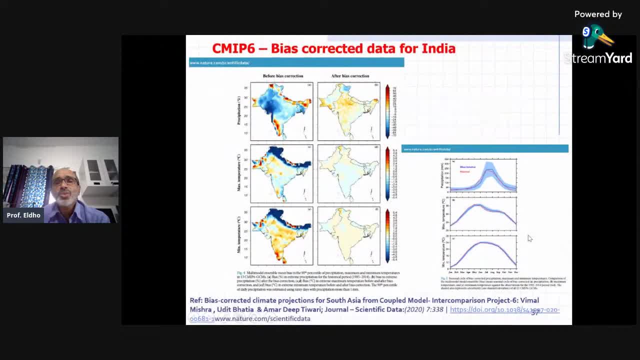 So we can do this downscaling and then we can use it. So now say, for example, as I mentioned, I am going to present a case study with by using the CME-5 RCP scenario, but the CME-6- what can happen? a study published by Professor. 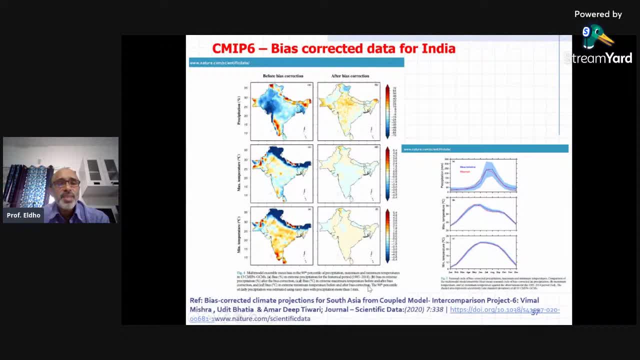 Vimal Mishra and his team. in the journal scientific data you can see what is can happen Before bias correction. So this is what is why bias correction is important. So here, before bias correction, you can see how the precipitation maximum or minimum demolition 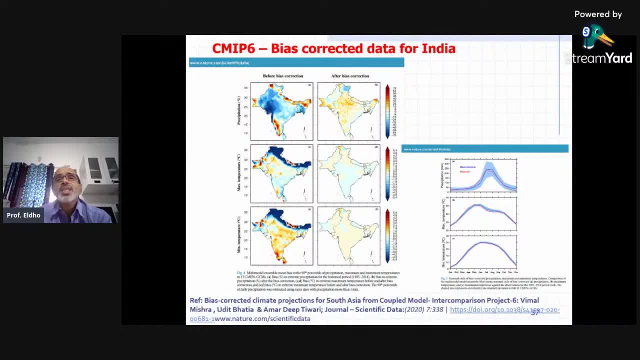 and then, after bias correction, what is the reality? So bias correction is very, very important in as far as the climate change impact assessment is concerned. So we will be generally using the. as far as hydrological model, we need to use the bias. 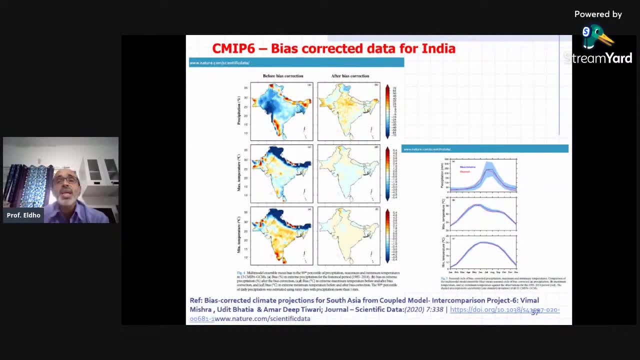 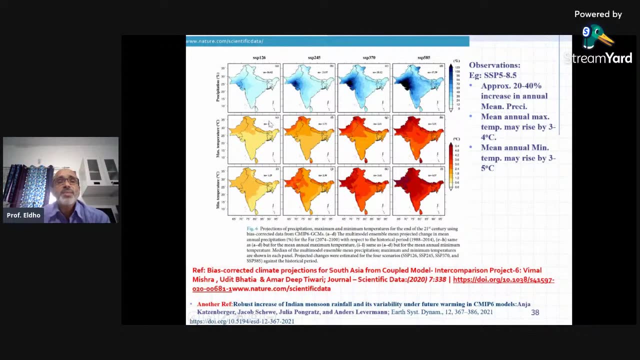 corrected data so that we check for last 20 or 30 years, that we use it and then we get a Reasonable good match and then we can use that GCM data for further hydrological modeling and studies. So here say for example this: what is happened with respect to these studies? there are two. 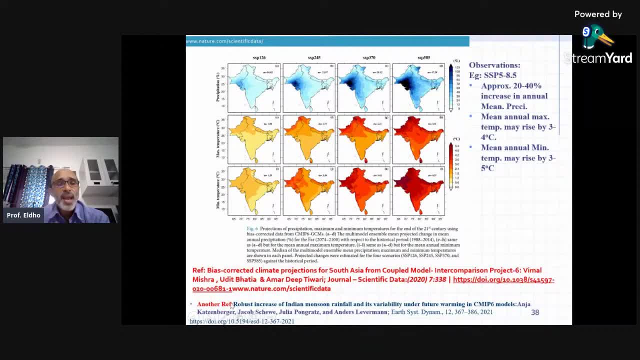 studies which I have just seen recently. one is another Professor Mishra's studies and another one is published in, say, Earth System Dynamics: So robust increase of Indian Mountstone rainfall. So here you can see that SSP 4.5 to SSP 8.5.. 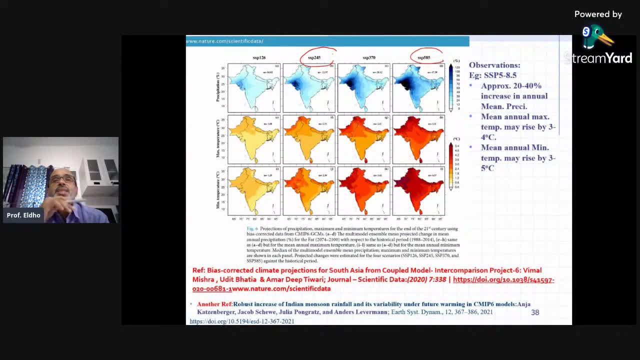 So in all those things we can see that say what is, what is? the latest? prediction also shows approximate 20 to 40% increase in rainfall, mean annual precipitation and increase with respect to, say, for example, 1901, and then similarly the precipitation, the annual maximum temperature. 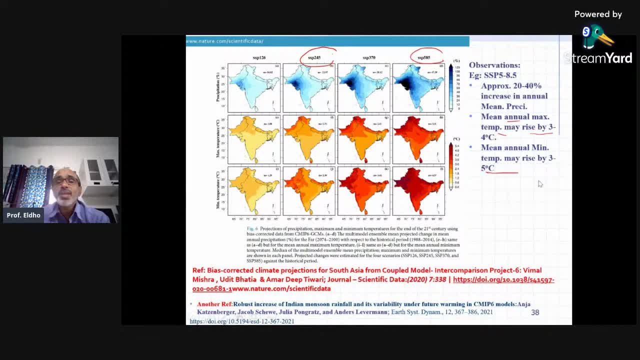 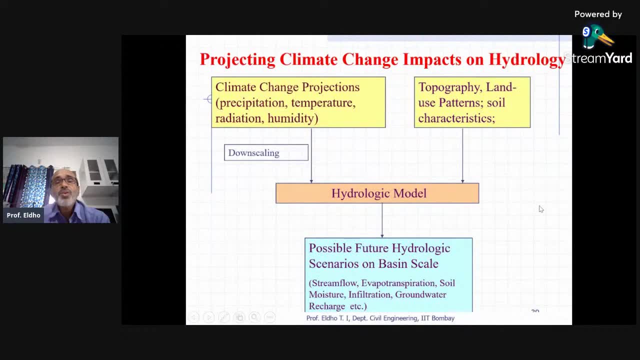 also there is increase and then, similarly, minimum temperature also. So those who are interested, please go through this category. So we should use more detail, but we are going to use the RCP 4.5, 8.5 scenario, whatever the case studies which we are going to discuss now. 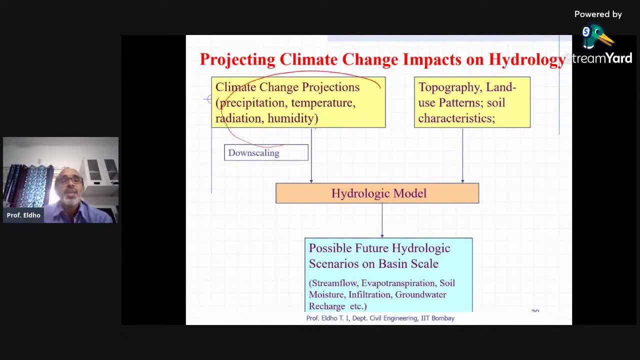 So here are projecting the climate change impact. So here, what do we get after the downscaling? So we are, by using the topography and land use pattern and soil characteristics, We run the hydrological model and then we go for possible future hydraulic scenarios. 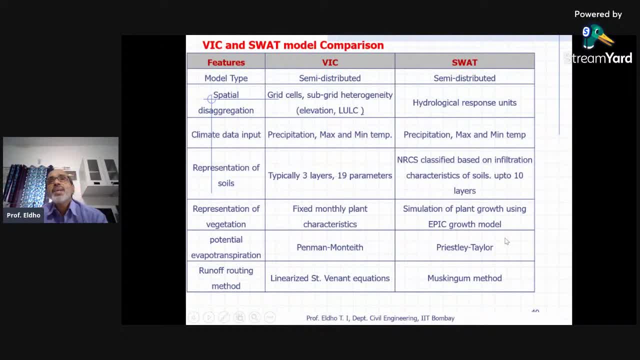 or basin scale. So here, As I mentioned, a number of models are available. So if you are going for a way of the river basin scale studies, then soil water assessment tool will be very useful and very commonly used. And then, if you're going for a grid based scale or a region scale or a for India country, 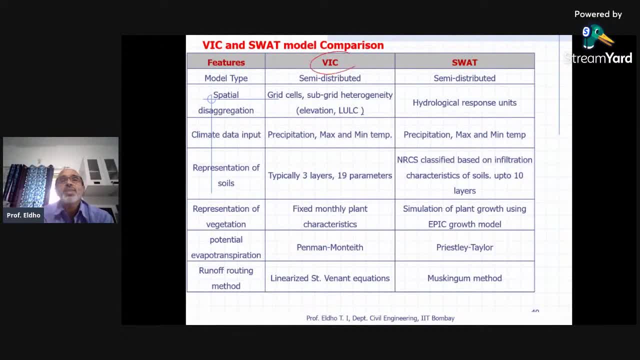 or global scale. we can go for a variable integration capacity model. A comparison is given here, actually as part of a sponsor project from Jalasekti Ministry, Government of India, And we are doing a study for Tadri to Kanyakumar. 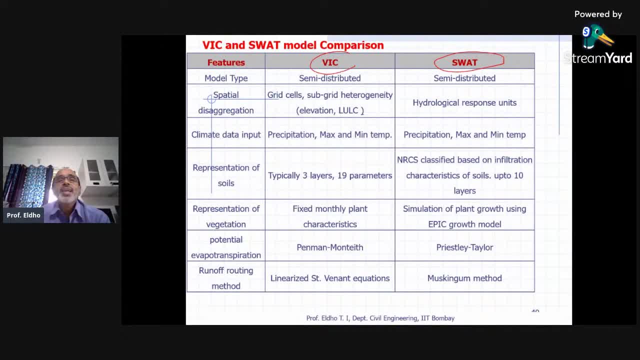 And we are doing a study for Tadri to Kanyakumar, And we are doing a study for Tadri to Kanyakumar Until we get the descent for Tadri or Jalasekti from Beheами or Say esse. the climate change. 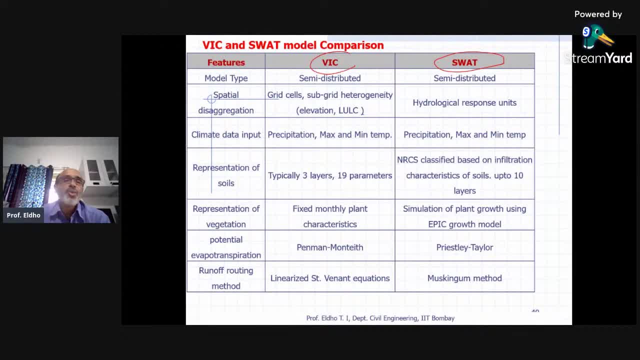 impact. So we are using both these models, BIC model and SWAT model. So I am going to present the results from the SWAT model study for river basin in the West Angles region, southern India. So here Here, These two models are both semy. 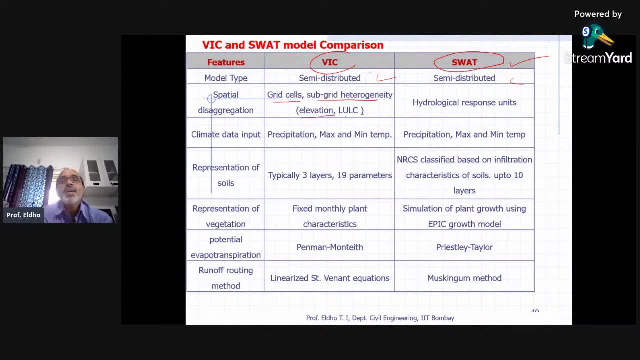 And the spatial disagree Crinyation. here good sense, sub grid heterogeneity or elevationation, NLC data directly can come from the grid. And here what is concerned? we use hydrological response unit- Okay, may respect critical point- and frying low shallow over field, over sea, Sycamore. 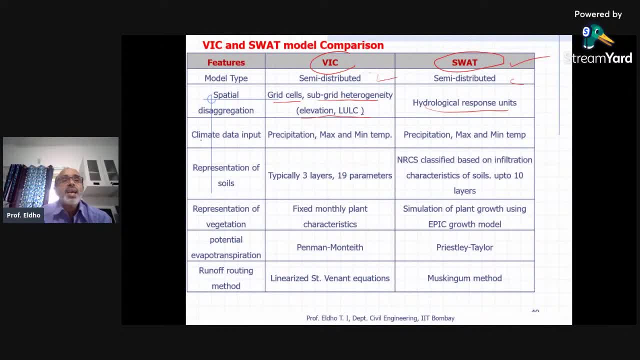 von what Ip? what are you coming here? sources for a ET model- What are you talking about units? and then climate data input is concerned, here for EIC model: precipitation, maximum, minimum temperature, etc. here also very similarly So. here a representation of soil, typically three layers of soil. we use SWAT, we can go. 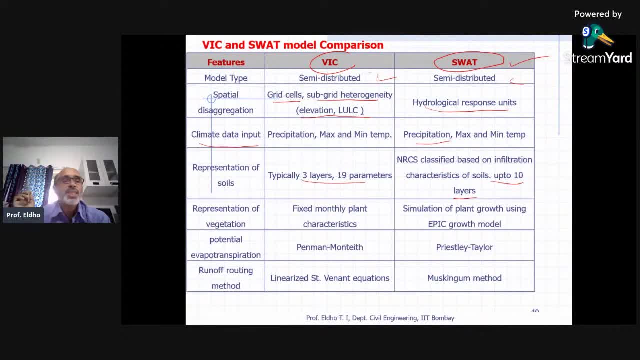 up to 10 layers of soil data so that all infiltration details can be taken care And a representation of vegetation fixed monthly plant characteristics can be taken care in EIC, In SWAT, the simulation of plant growth using EPIC growth model will be used, and here a. 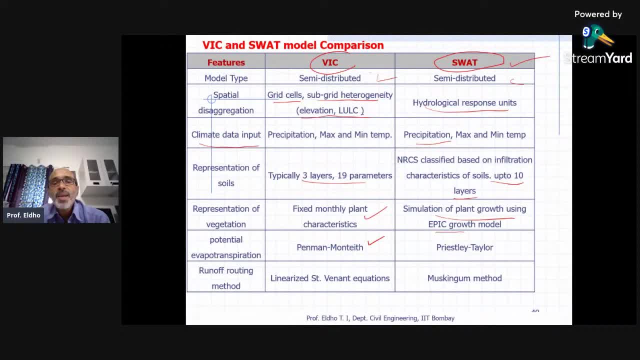 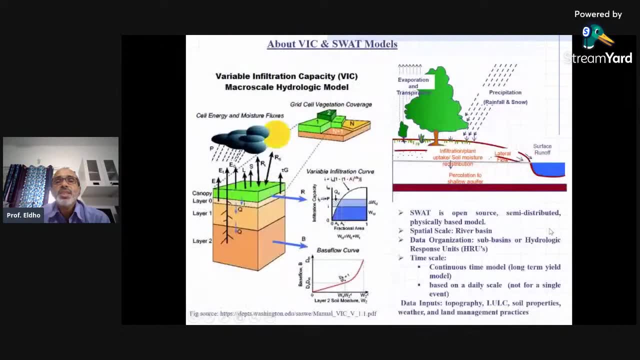 potential evaporation. in EIC they use a Penman-Mondeleev model, here a Presley-Taylor model, So like that. various option you can see here. So this is the overall sketch of EIC model and SWAT model. So EIC is concerned, we can say grid, like this, and then, with respect to this, three soil: 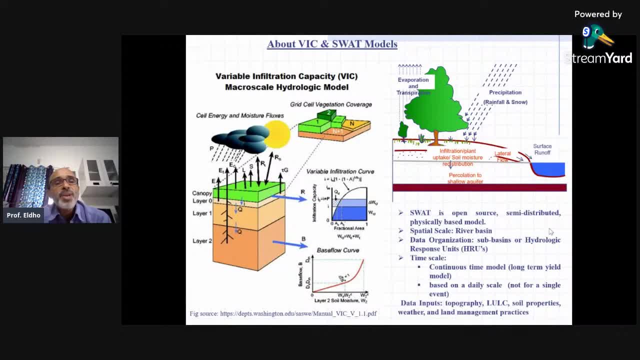 layer and with respect to precipitation, how the evapotranspiration, all those things are studied In details. you can see, I am not going to details of the model, but this is freely available, so you can download both models and then you can use it. 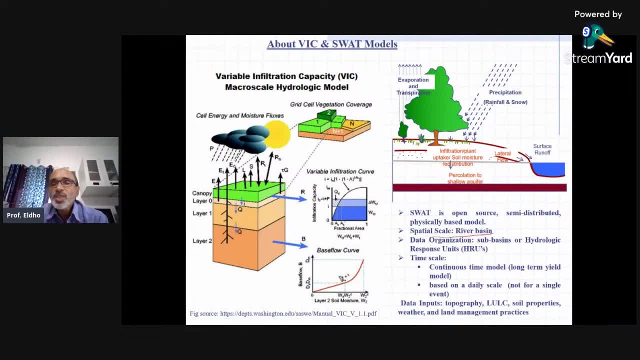 So SWAT is an open source, semi-distributed physical model, semi-spatial scale river basin, so that sub basin or hydraulic response unit, The time scale it can be continuous time scale model and based on a daily scale also we can run. So input required is topography, LULC, soil properties, weather and land management practices. 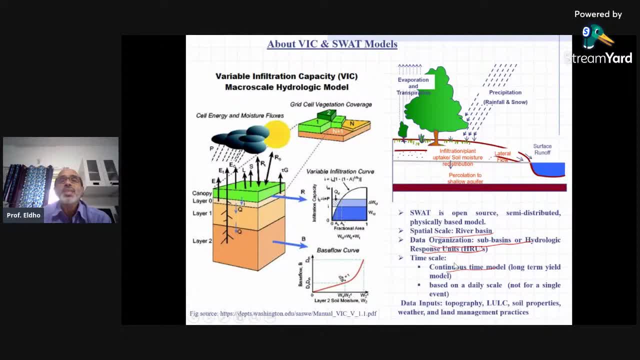 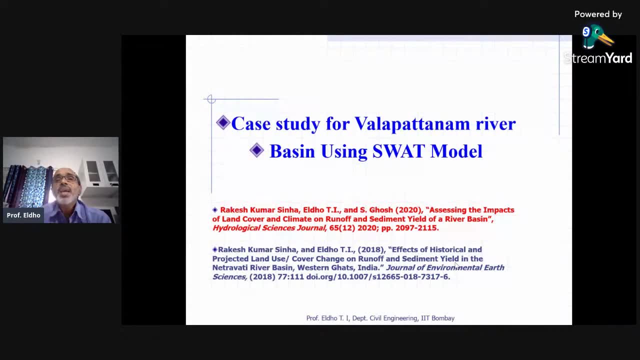 So both these models We are used for our studies, but here I am going to present the SWAT model for a river basin scale study is concerned. So now we are going to have a discussion on a case study. So here the case study is taken from the West Angle River Basin in South India, which is 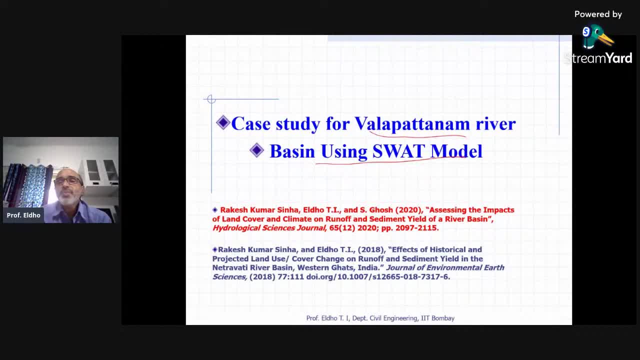 called the Vallabhatna River Basin using the SWAT model. So those who are interested, you can refer to this paper so which we have already published, this journal, Hydraulic Science Journal, And then also another paper in Natravadi Basin. this is another journal, the paper which we 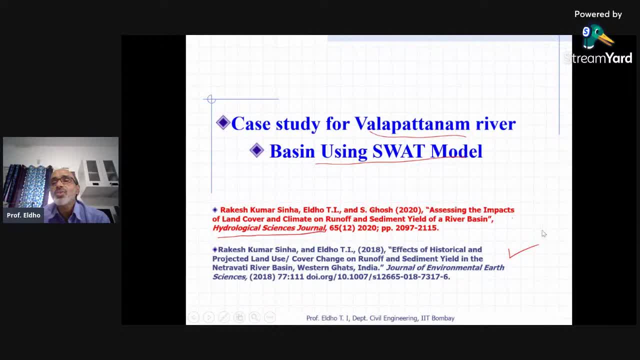 have published, So those who are interested you can go through this- how these kinds of studies are undertaken. So now this case study. we are going to discuss in detail how we conduct such studies and then what kind of inputs are needed and what kinds of outputs are needed. 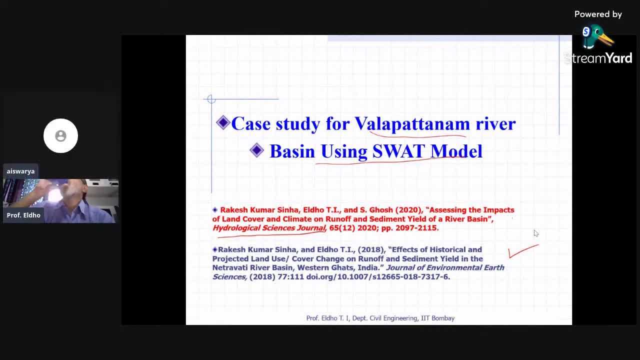 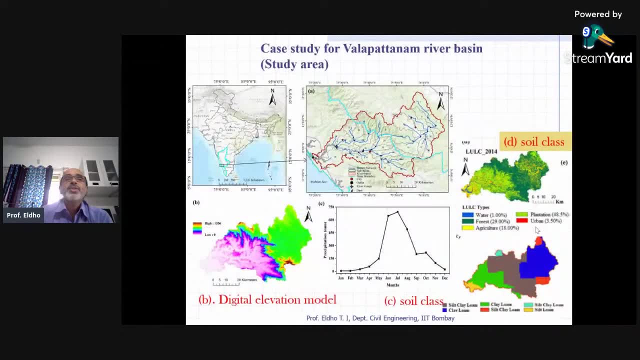 So, Aishwarya, am I audible and everything is fine? Yes, sir, you are audible. Yes, sir, Okay, So this case study is Vallabhatna River Basin. You can see here. This is the. This is the location map. 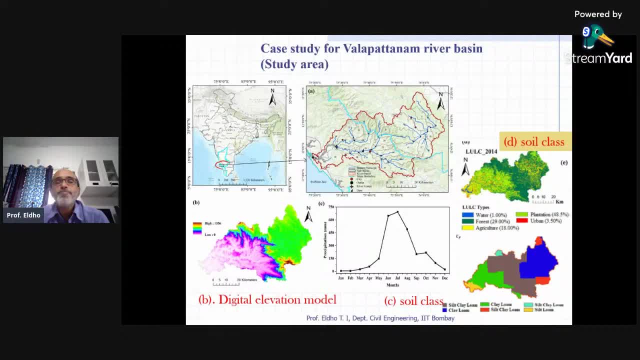 So here this is the boundaries of the river basin and correspondingly you can see the land use, land cover, say, for example, 2014, and then the elevation model. the elevation varies from zero to, since it joins the sea. so here, zero to 1556, and here so the monsoon. 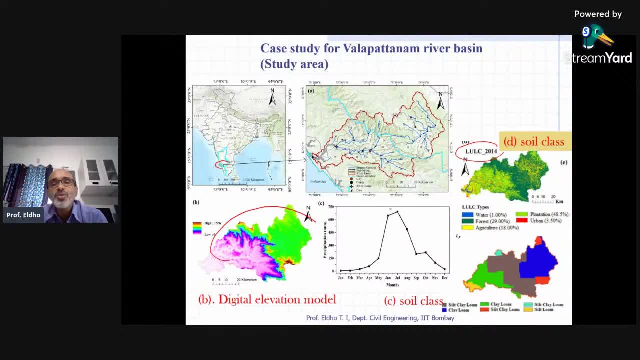 pattern, say. here the rainfall pattern is mainly the monsoon rain, starting from June to October, And then, of course, the retreating monsoon. also, 7% happens in this area, And this we are using NBS soil data. This is the details available. 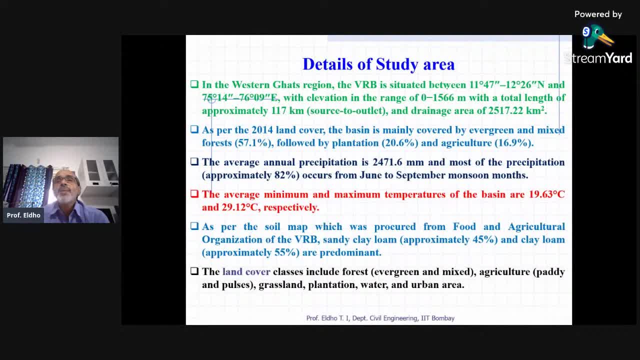 So here the details of the steady area. So this is latitude and longitude is given here. So the river length is approximately 117 kilometer and the drainage area is around 2500 square kilometer. So here, as per 2014 land use, land cover basin is mainly covered. 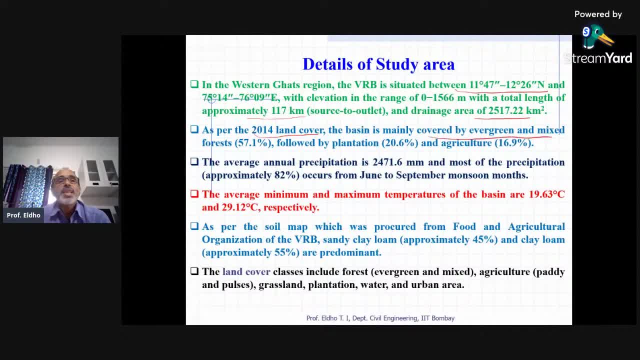 So this is the drainage area. So this is the drainage area. So this is the drainage area And scheme is provided by above and sulphurous plus about some percents, And then all the plantation and agriculture, So that kind of variations are observed everywhere. that allows per inflation. 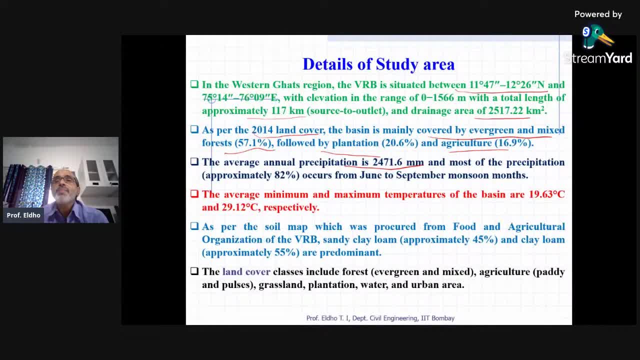 The Gegenscheider is about two thousand five millimeters and must specific and most 82 percentage between September must. So the average minimum maximum rain isência ninety six to nine point three, when that means to be sunny, nine point one degrees centigrade. 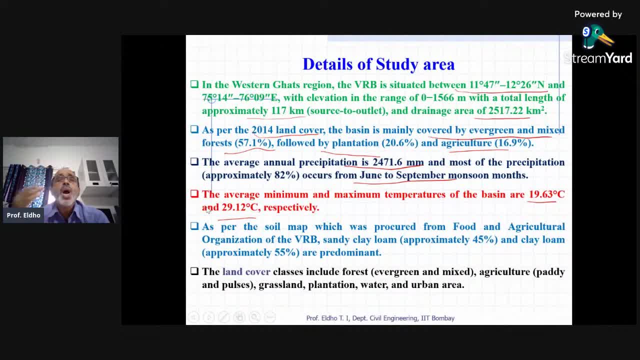 So this systematically show you how you can collect all these, Can collect, and you can collect all this data and do a hydrological impact studies with respect to climate change, and then what kind of data are required and then what kind of output you can get. 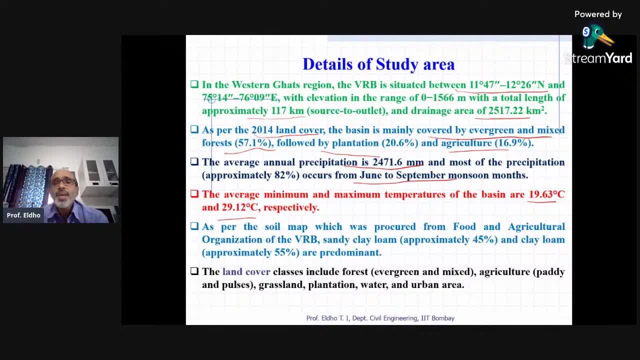 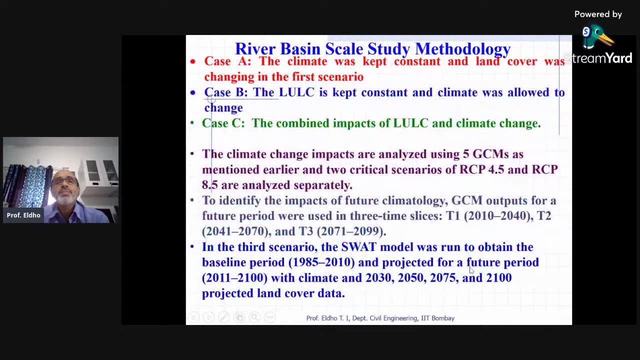 so, as per the soil map, we are you so here, mainly agricultural. the the soil is sandy, clay loam and the clay loam, so that is the soil data. and the land cover classes include forest, evergreen. it's an agricultural kind of land use landlord. so here the studies. whatever we are doing is three. 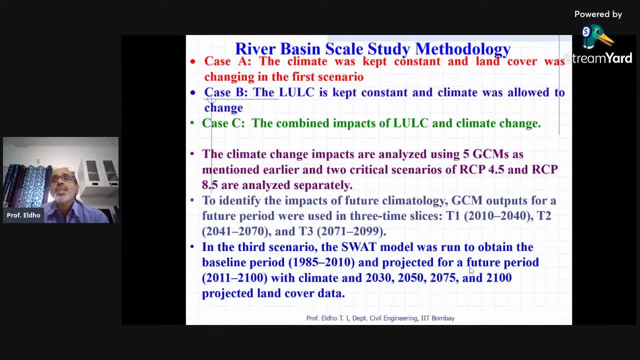 types of studies we are doing. one is the climate was kept constant. as i mentioned, land use, land cover change is a major issue. and then what are we its impact as far as the climate change is concerned, so that we need to study separately? and then if lulc- land use land cover is kept constant. 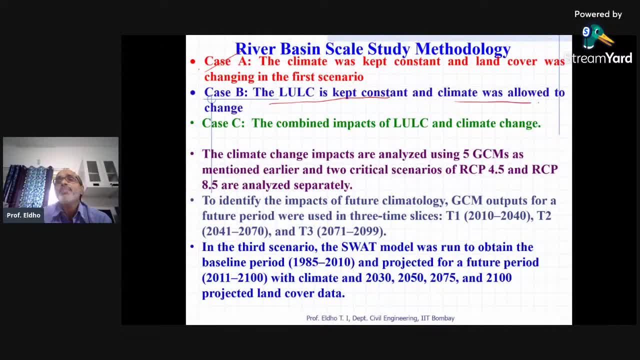 so that is the first study and second studies. failures is kept constant and climate was allowed to change. so, whatever the data that that we are getting from gcms, then we are running the model and then we are getting the. what are the impacts? the climate, only climate, is concerned. and then, finally, what is reality is the combined 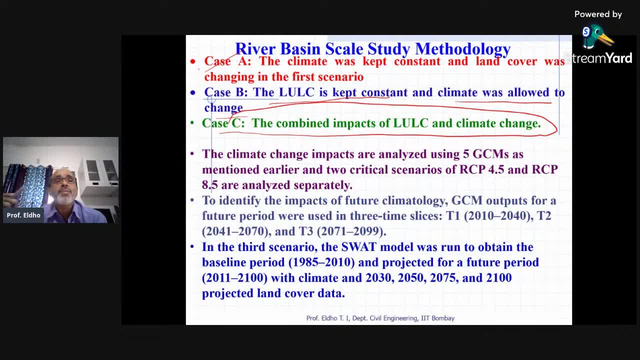 impact of land use, land cover and climate change. so that is the final rate. but we need to see uh, since the the land use land growth changes um happening drastically in many of these areas. so we need to assess that also so that we can um show: yes, if the land use, land core change is happening like this, then 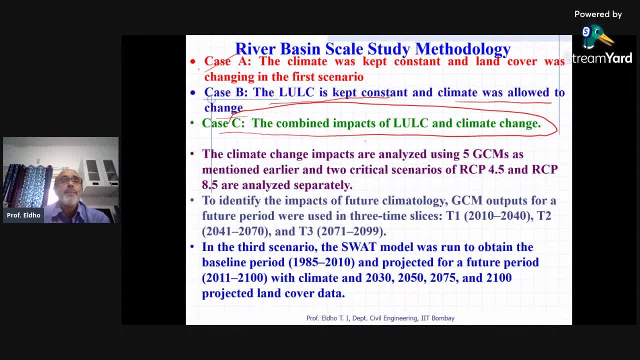 impacts and then, of course, climate change, case b, and then come back. so climate change impacts are analyzed using five gcms, as mentioned as part of this project. uh, so here two critical scenarios, rcp 4.5 and 8.5, are analyzed separately. so rcp 4.5, as i mentioned, the current trend goes, uh, that: 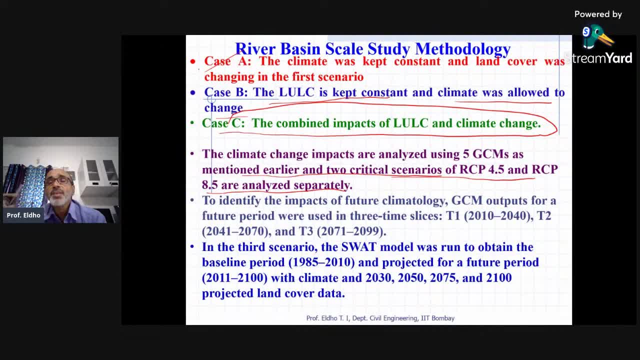 means it is uh and the gas emissions or or the carbon dioxide there is a only small rise is there, but rcp 8.5, the extreme case. so the medium case and their extreme case. that is what we used in this study to identify the impacts of future climate: all the gcm outputs for a future periods. 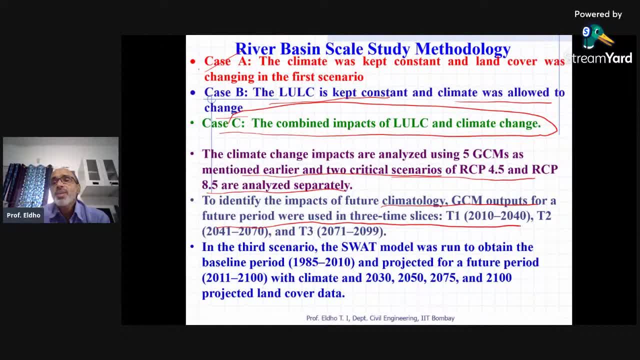 were used in three time slices, so 2010 to 40, then 41 to 70 and 71 to 2100. so the third scenario, sat model, was run to obtain the baseline periods, say by taking 1985, 2010 and projected for future period. 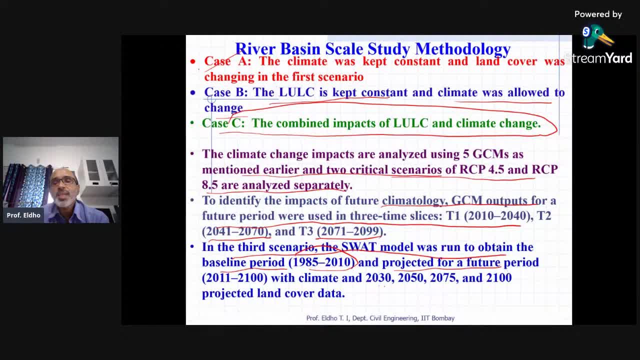 up to 2100 and with the climate of 2030, 50, 75, 2100. with this, this land cover data correspondingly 2030, 50, 75 and 2100, uh kind of land data. so this flowchart, so you can see these details in our published 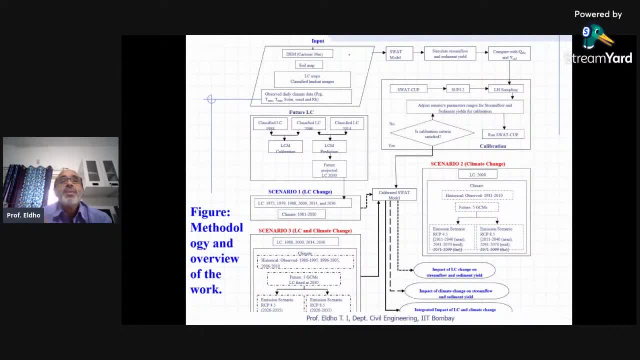 papers, also the methodology and the overview of the work. so here, uh, we needed the data, like dm and data, soil map, land use and core map observed the, the climate and other precipitation temperature- all data- and then swag model so similar to streamflow and sediment yield. so i am presenting only this. 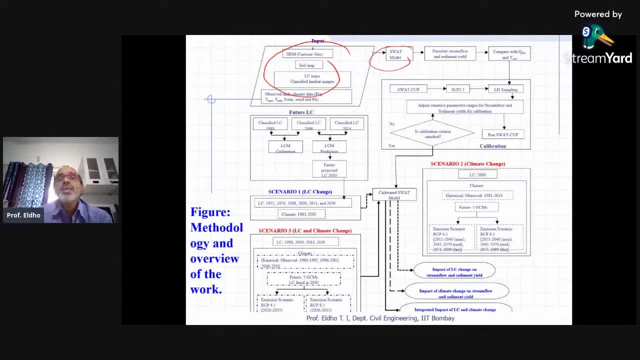 the runoff here and then compare, then, uh so we the swag model, we need to do a lot of calibration, so we use that cup model, so we add the sensitive parameters, then calibration quite is satisfied, then our model is ready and then scenarios are concerned. as i mentioned, the only land 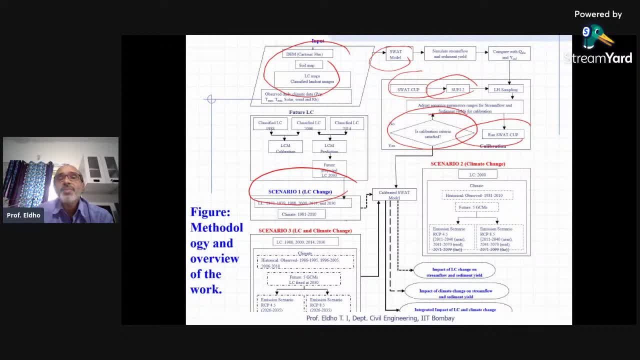 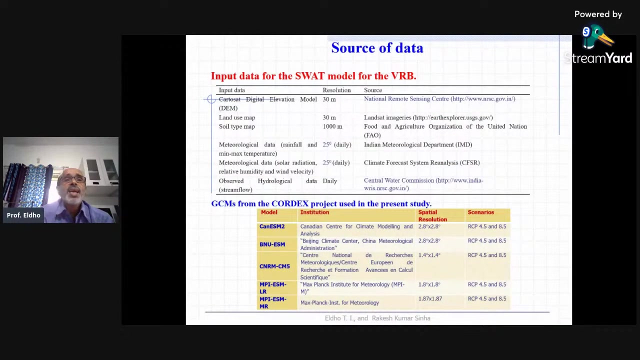 land cover change- case a. and then we do a up to 2100 and case b, only climate change. uh, by using a land use land core constant, and then, finally, we do the assessment with respect to the combined impact of land, land use and core change and climate change. so that is the way for rcp 4.5 and 8.5. so the source of data here i have. 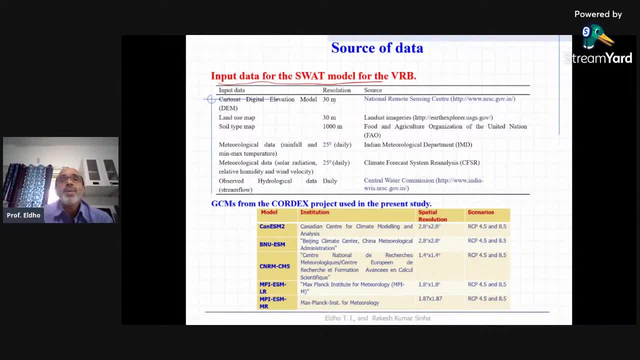 listed input data for sat model. so here we use the 30 meter resolution dm land use map map we get from from landsat imageries with respect to 30 meter and soil type map is around 1000 meter. and then the material data. so we are using the 2.5 degree scale and the observed hydrological 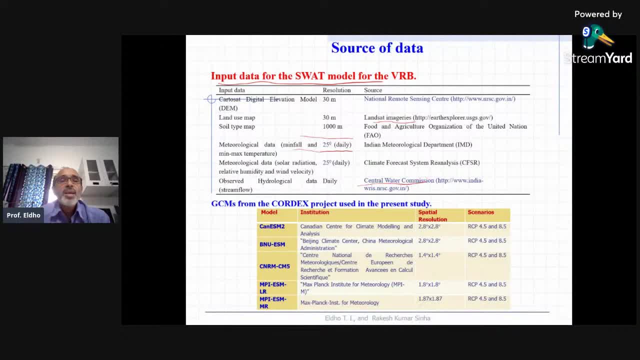 data, daily data. we are using a grid scale, so here we use the. this is not product project, sorry, here we are using this: five, five gcms, so here this is. this is what we are using. this is not cortex project. sorry, this is wrong. the gcms from the five canadian gcms then. 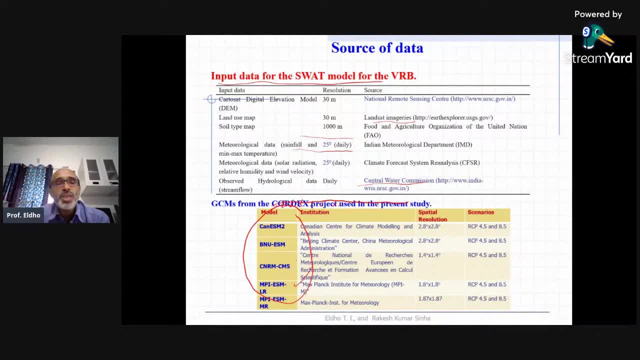 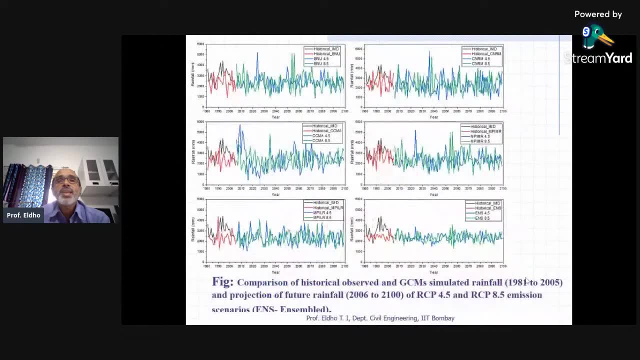 beijing climate center gcm. these are the five gcm which we are using in this study, and corresponding spatial resolution is given here and corresponding scenarios are also given here. so first we need to see what is happening with respect to this whenever we are downscaling, and then 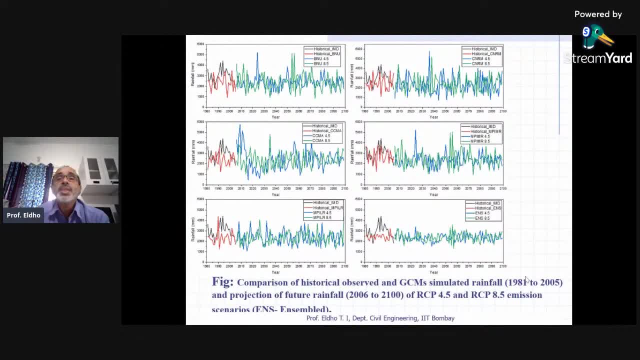 so the statistical downscale products available we are, we are using here and then we need to do you. and then the comparison of historical option, gcm simulator, rainfall 1981, 2005 and protection for up to 2100. you can see here. so here, with respect to imd data, directly what is? uh, it is. 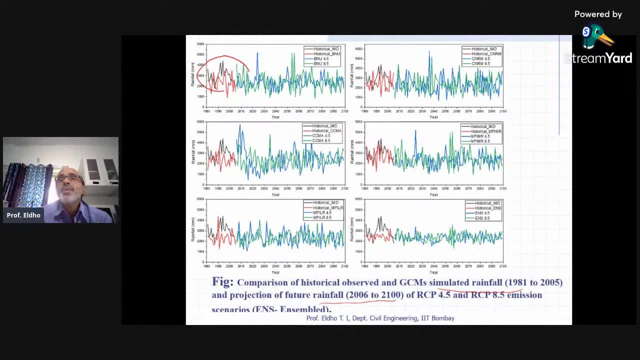 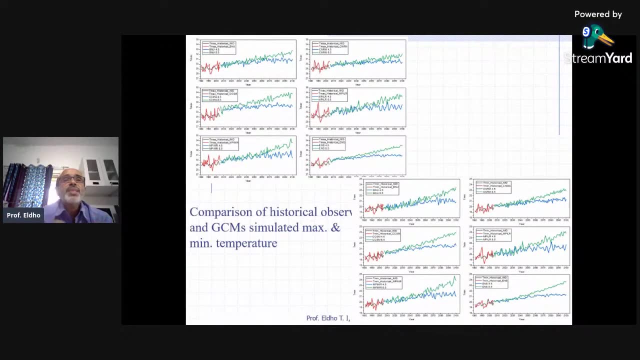 that we are getting reasonable uh match and then only we are going for using various uh five gcms. as i mentioned, we are using here and we are getting a reasonably good match and that is right and we are using the same. so correspondingly, here you can see the, the maximum temperature. 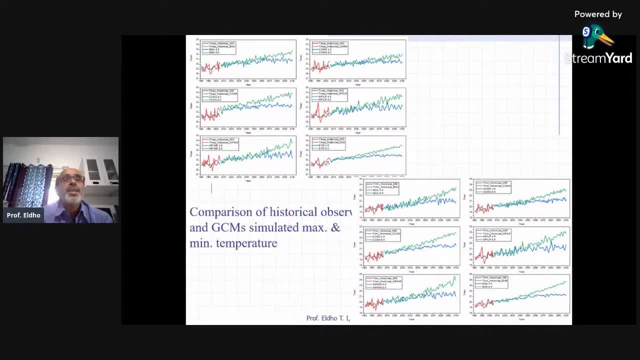 variations you can see here with respect to rcp 4.5 and 8.5. so this is the ensembled one with respect to all these 5 gcms. so here, 5gcm, what are used, already mentioned here. so correspondingly, the ensemble 1 is shown here. so, with respect to rcp 4.5 and 8.5, this is 4.5, this is 8.5 and this shows historically uh with respect to the, the minimum uh temperature left over before. that is, and this is the 8.5 and this is the combo: rcp 6.25, which means we see what rcp 6rain queda is representing here. unit rate is showing here and it is the value from rcp 4.5 this grew to current 24 hours to 8.5, which reaches feets, if that is 심ficiente. but again, here this is the environmental. 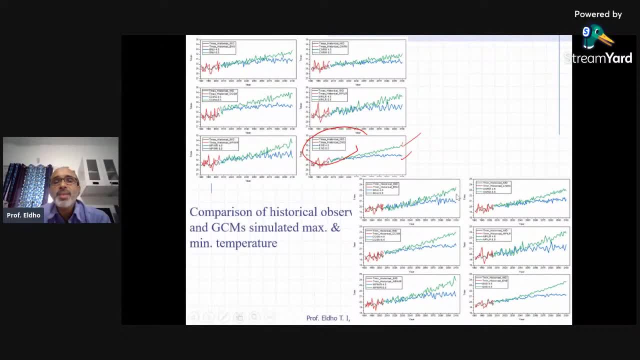 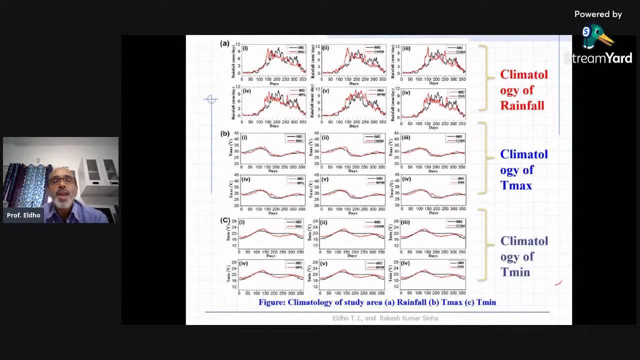 and this shows historically, with respect to the, the minimum temperature radiation. also with respect to ensemble one, this is a 8.5 and this is a 4.5. so that kind of details are obtained and here the climatology of rainfall. so with respect to say, for example, annual base, how the changes. 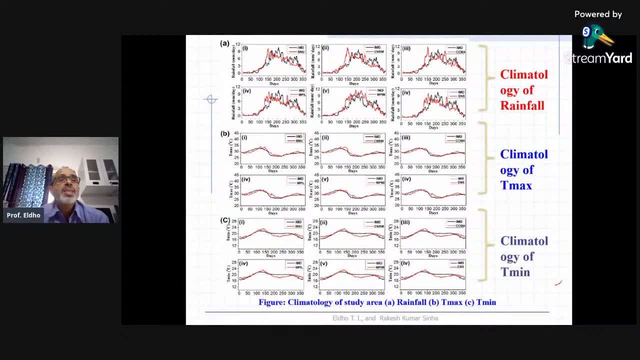 taking place with respect to the rainfall, you can see here, the rainfall and the with respect to imd data, and then we compared with respect to various gcms, and then so we, we use the ensemble data and similarly here you can see: so this ens means the, the ensemble. so this is what we are. 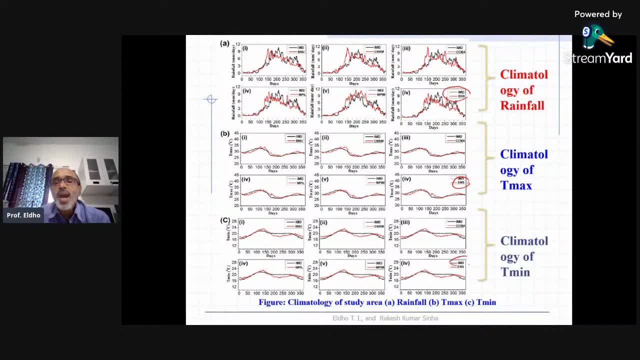 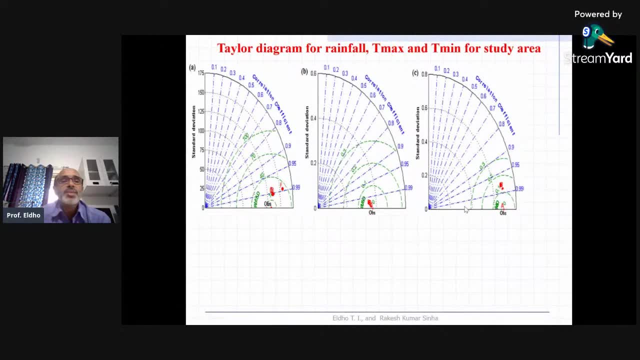 using, so that we are getting a very good match. so that way we are using this gcm data. so this shows the table diagram for rainfall: t max and t minimum for the study area. so you can see that very uh, good match we are obtaining serum point uh, the nsc values 0.8 to 0.9. we are getting so 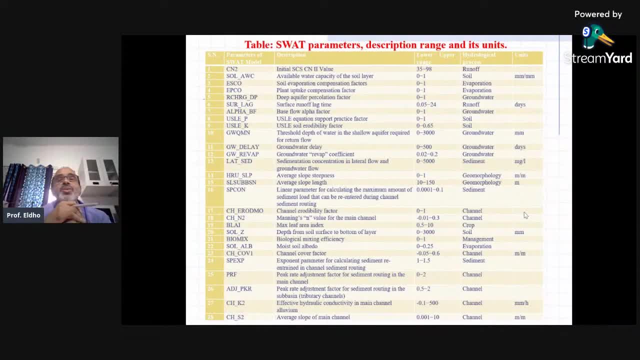 correspondingly and that is why, and these gcms we have chosen, and then these are used for the, the, the river scale, river basin scale assessment. so here a swat model is concerned, there is a large number of parameters are there, like here? i have listed 32 parameters. so many parameters. 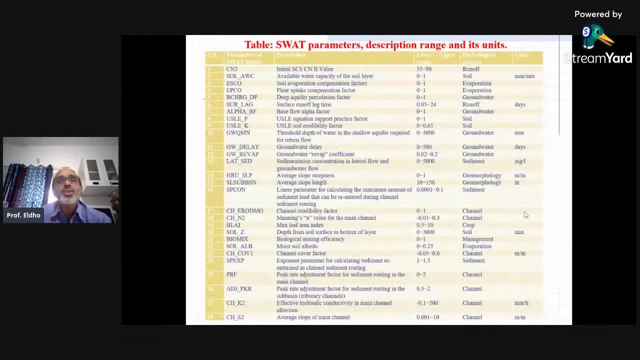 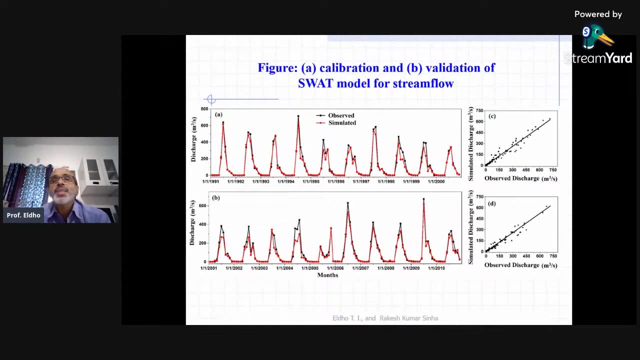 are there. so we need to calibrate the parameters also from this. we have chosen about around 15 parameters which are found to be very relevant as far as these kinds of studies are concerned. we have calibrated it and then this shows the calibrate calibration and validation of the sat model for stream flow. so you can see that. 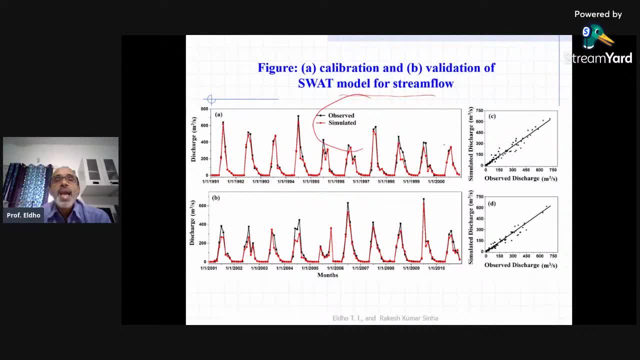 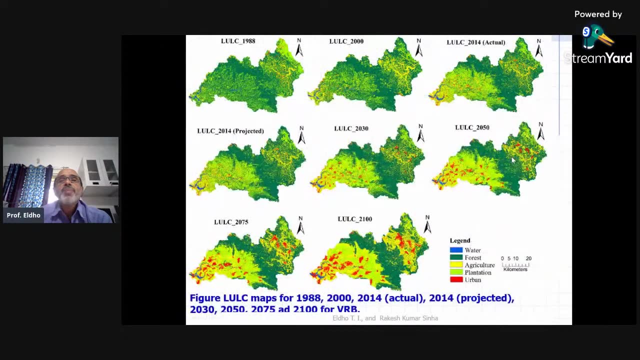 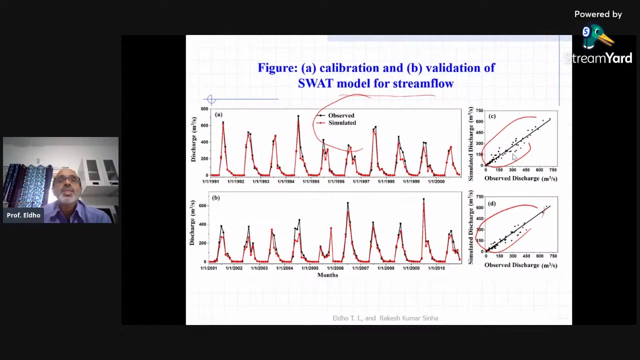 starting from 1991 to 2000 data is used for calibration and from 2001 to 2010 is used for validation. so you can see that very good match after the calibration is obtained with respect to various swat parameters. so that way we have observed that swat can give up to the very good results as far as this river basin scale. 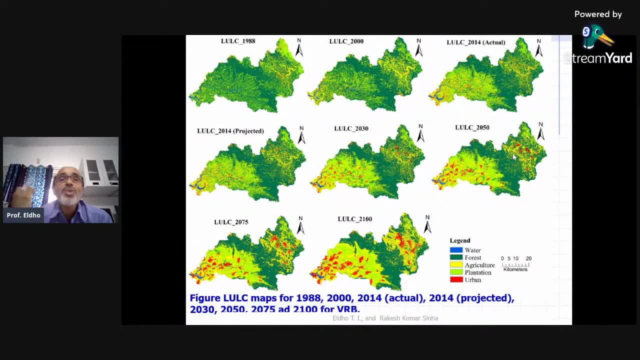 modeling is concerned. so then, another question is, as i mentioned, land use, land cover changes. so land use, land cover changes. so it is not only the climate change, land use, land cover change is also very important. so you can see here: uh, so we used what we did, there, we, we. 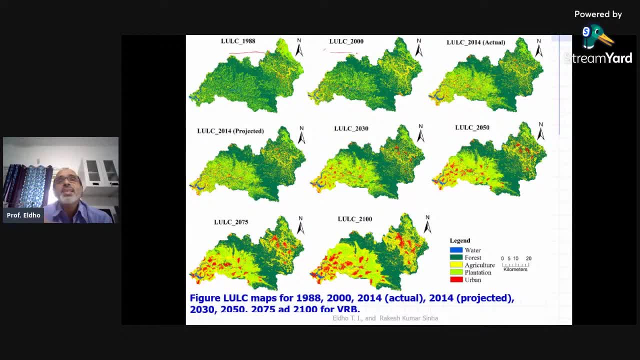 we got the from the landsat data. we got 1988, 2000, 2014. all these data are obtained and then we use air dash models for the projection, for the land use, land plot projections. so here this shows the actual 2014 and projected. it is compared, so we got a very good correlation. 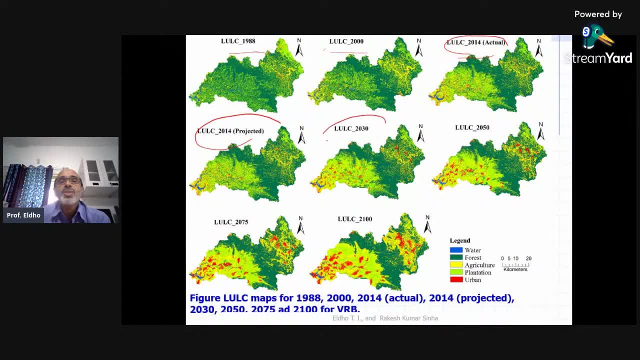 and then, based upon that, we further projected the land use landlord for 2030, 2050, 75 and only 100, and data were used. So here this river basin scale is concerned, it is a say if it is a 2014, hardly five to six percent is the urbanization, so it will be increasing around to 14 percent by 2100. 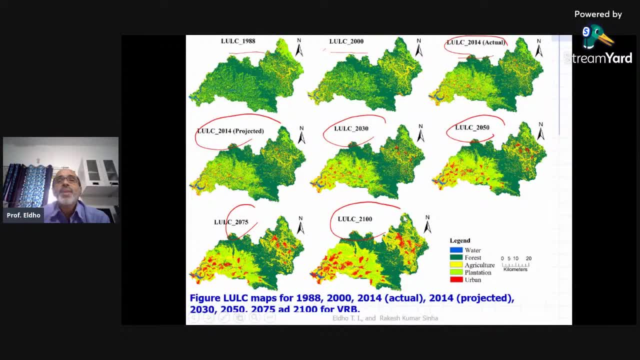 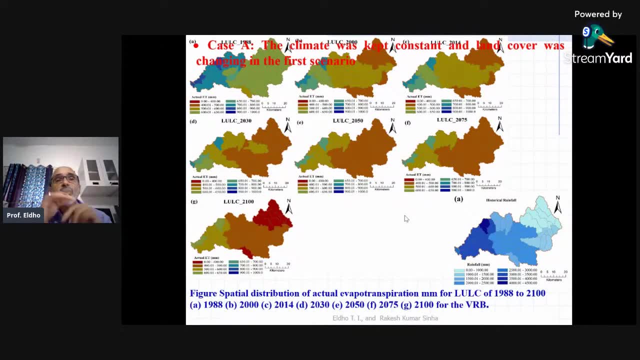 so that is so, this, this data, which is a projected land use land cover data, is also used. So, as I mentioned, three kinds of scenarios we are simulated here. so what is the impact of the land use, land cover change only? and second one is: what is the impact of climate change only by keeping LULC? 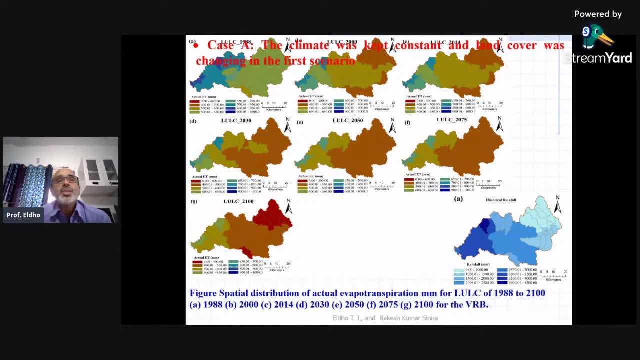 constant and then the combined impact. So here this shows the spatial distribution of actually evapotranspiration with respect to: so this is the rainfall and the historical rainfall which we used for this assessment. so year 2030,, 50,, 75,, 2100- how the variations are taking place. so start this is. 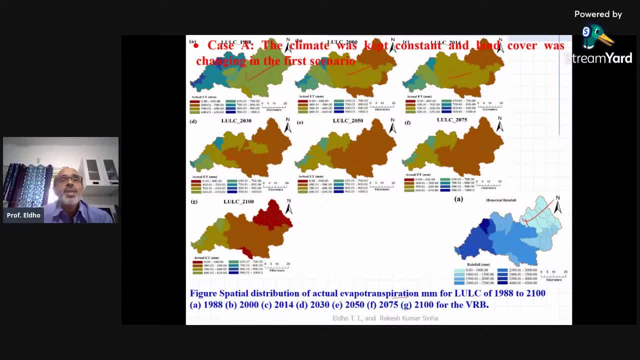 88,, 2000,. 2014, then 30,, 50,, 75. and 2100. so you can see that the climate compared to climate change, the land use, planetary change impact is not that much, but still a lot of changes you can observe since, as I mentioned here, you can 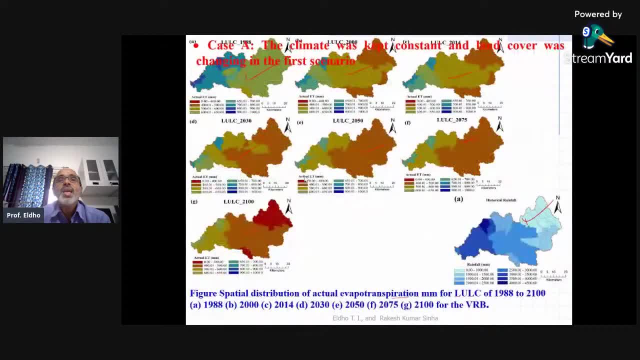 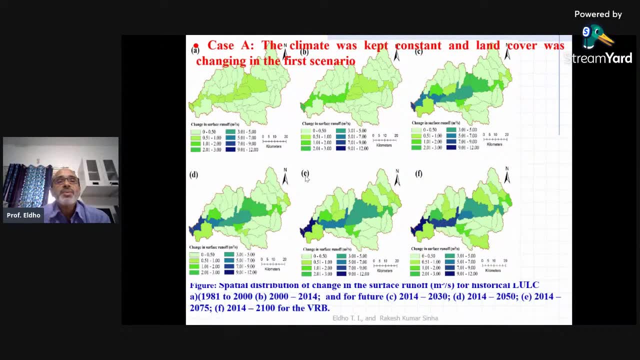 observe here a lot of land use, land core changes taking place accordingly, evapotranspiration, spatial distribution, evapotranspiration changes and then this shows the climate was so the the the impact on the spatial distribution of a surface runoff. so with respect to 1981 to 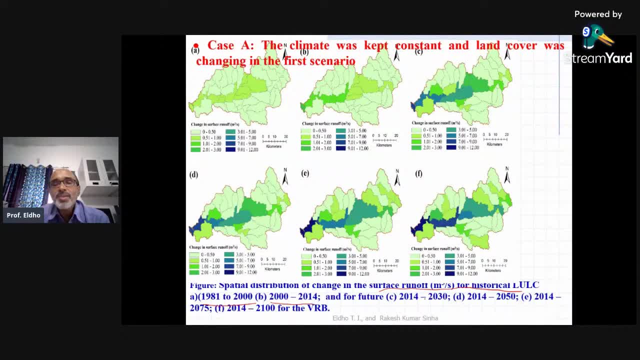 2100, so 2000 and 2014. so what is the changes taking place? figure a: this is with respect 81 to 2000 and then at 2000 to 2014. then that is the difference, this is only the difference is: 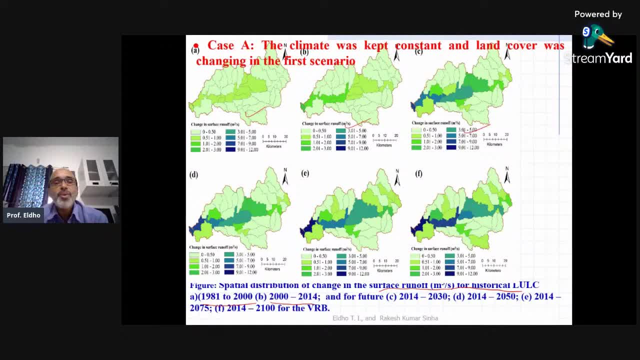 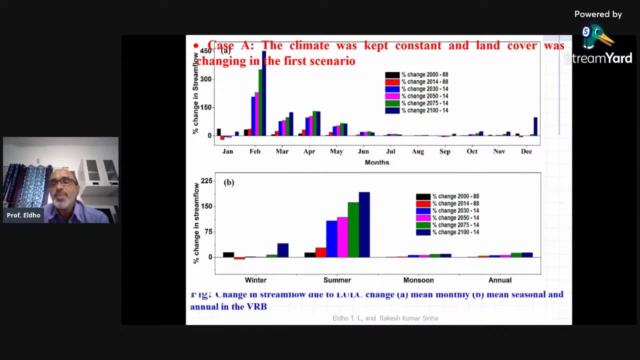 plotted here, and 14 to 2030, then 14 to 50 and 14 to 75 and so up to 2100. so how the with respect to agency changes? what is happening? what are the impacts? so this shows the. the impacts changes in stream flow due to luc. changes mean monthly, means seasonal and annual in the 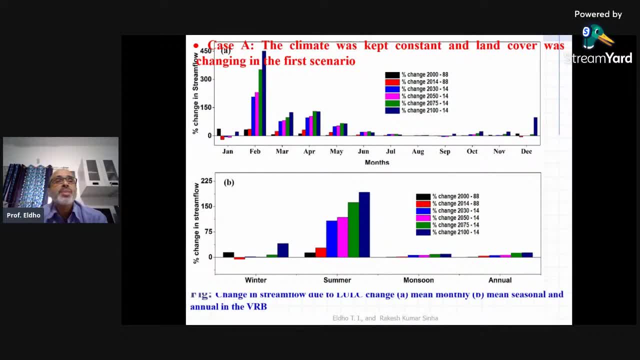 wallabata river basin. so how much percentage changes taking place so you can see the changes in stream flow? so here, especially summer rainfall is here observed and then the big changes observed as per the summer is concerned, but months on season there is not that much change, is not. 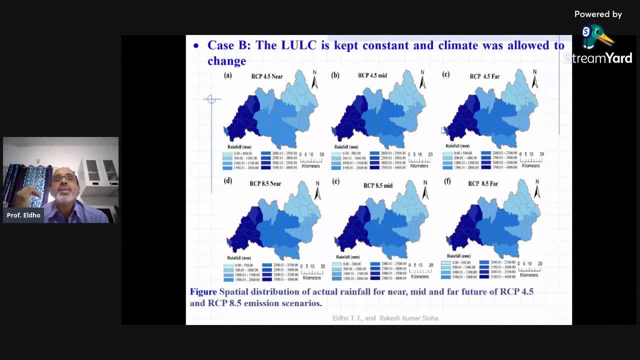 observed. and then case b. second case is land use. land cover is kept constant, say by taking 2000 and 14, whatever that is used as a base, and then we use the, the, the special distribution, actual rainfall for this river basin obtained from that, five gcm's. so here, rcp 4.5 near near 2030. 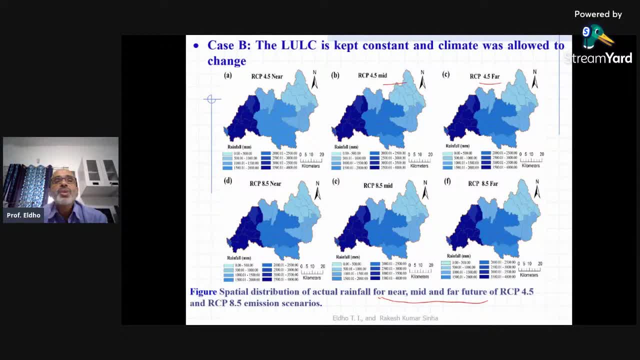 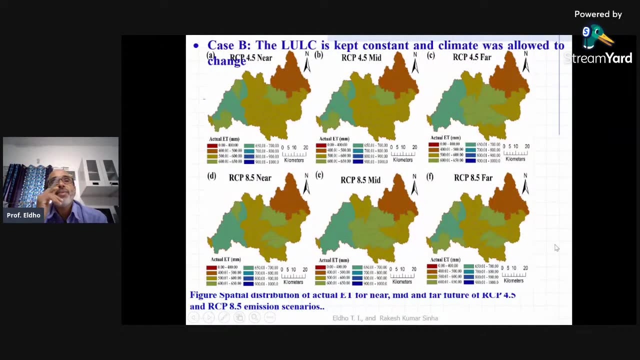 70, then power distance, so 2001 to 40, and 40 to 70, 72 to 2100, so correspondingly 8.5. scenario: the rainfall is put into the river basin, the special distribution is obtained, rainfall, and, and then we- we kept the ну sequence and run the more than so. here we saw the special distribution. 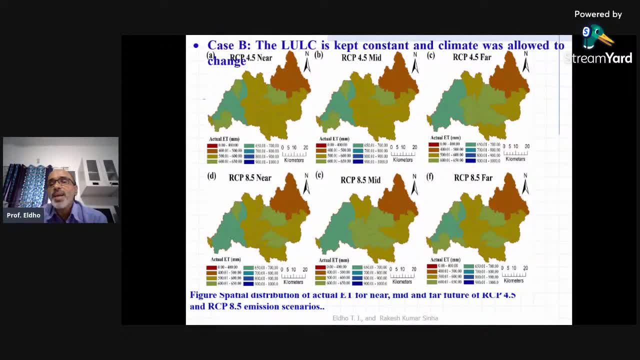 actually evapotranspiration for near mid future and power future, how the system will be, how the changes will be taking. so you can see here also compared to land use, downtown change, here the changes are more things that more not this river basin. what we analyze showed. 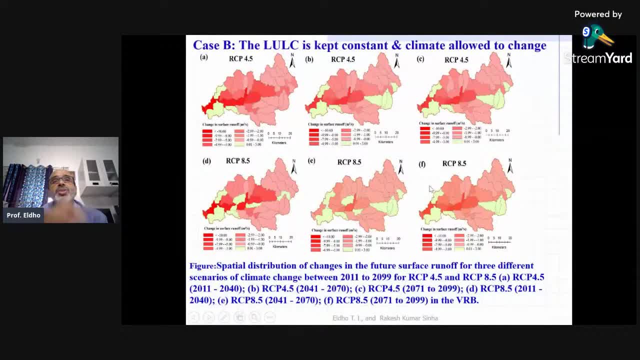 that the climate change in fact is more severe and this shows the lucs kept constant and climate is allowed to change. the suspicion distribution change in future. so another two surface runoff of three different scenarios how the variation is taking place for rcp 4.5. 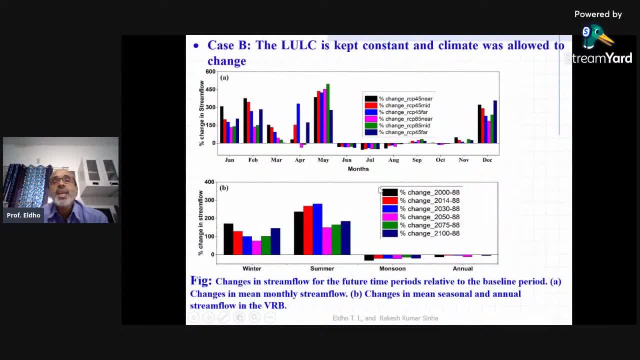 and 8.5, so that is shown in this video. so then again, monthly variation, seasonal scale, all the changes you can see here, this area, summer rainfall is this river basin, and there is an increases observed, and then monsoon, there is a small decreases observed. so like that, that kind of 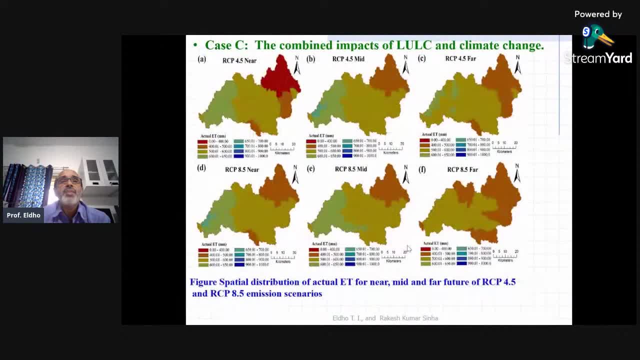 variation, monthly basis and also seasonal basis we can obtain and then finally we analyze the combined impact of land use and for change and climate change. so that is shown here. special distribution of actual evapotranspiration here: midland rcp 4.5, 8.5. emission scenarios you can. 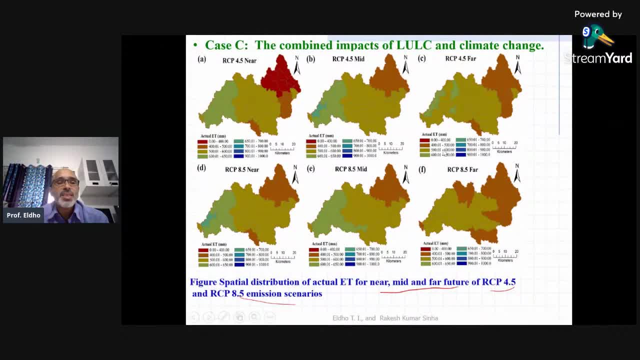 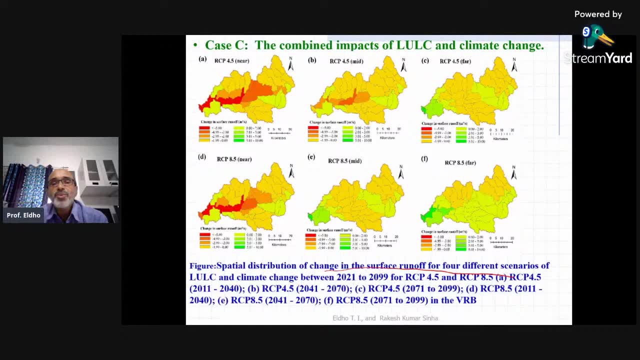 see here. so the combined with respect to land use and land cover change. so here evapotranspiration changes, then special distributional changes and surface, and now for different scenarios, up to 20 to 2100, so for 4.5 and 8.5, so that for the near width and far heater. so you can see that. 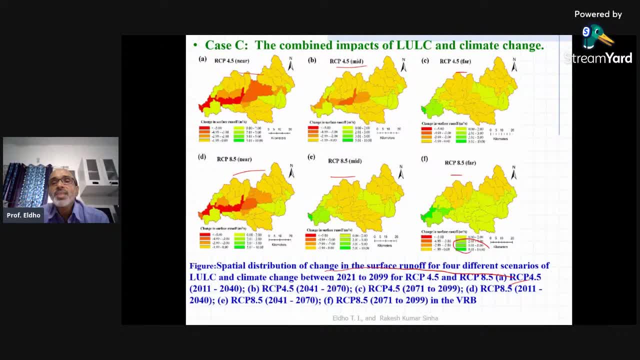 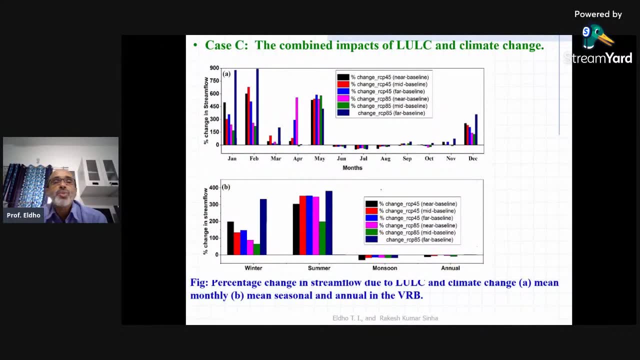 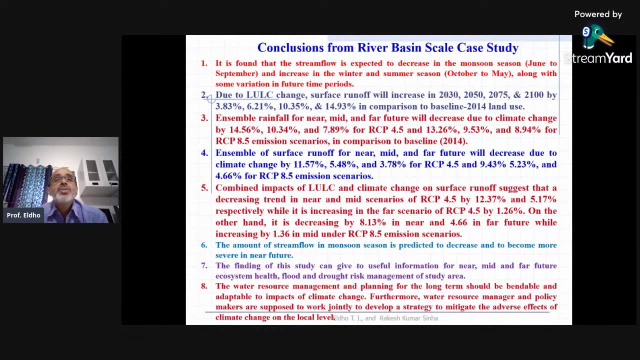 severe impacts, especially rcp 8.5. you can see labs. yeah, large impacts are visible. so then the combined impacts with respect to the monthly base. also we have obtained, and corresponding season wise also. so finally, the conversion from river basin scale study. so it is found that stream flow is expected to decrease. 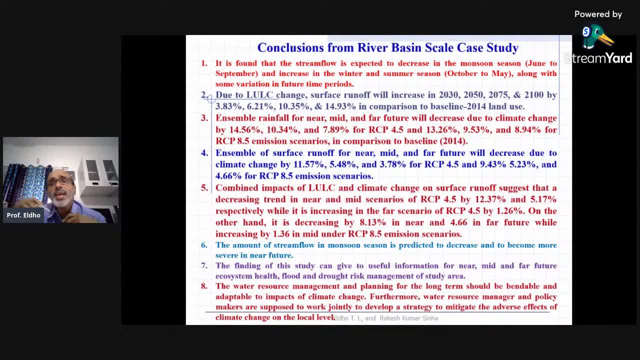 in the monsoon, So that, though the projections are for a- yeah, India or various parts are referring, but small scales, which is coming to river basin scale. the changes can be different, so that is what is observed here. here the standard streamfluous has focused in the monsoon season. 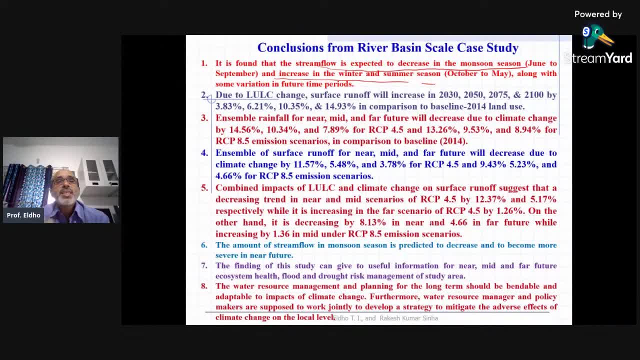 and increasing the winter and summer season, along with some variation, future change due to lluc change. surface are not going to increase in 2030: 50, 75, 2100 by uh- this much person, 3.83, like that. it is increasing and then ensemble rainfall near mid far, which will decrease due to climate change. 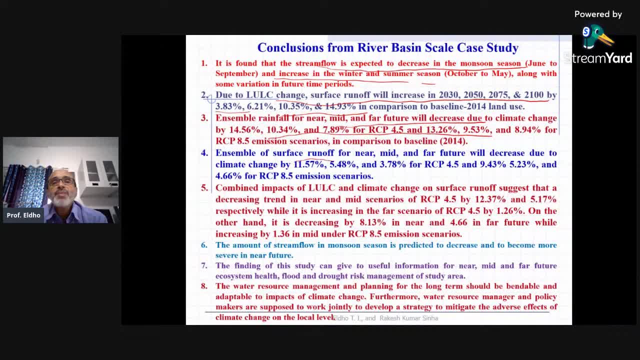 so that is uh. what is this? person issues and ensemble surface are now for near mid and will decrease due to, uh, climate change. so this is a decrease, especially this river basis is concerned. so then, combined impact of aliens and climate change shows so suggest that a decreasing trend. 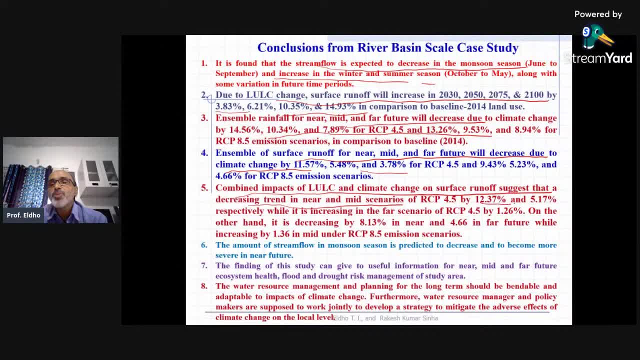 in near and mid scenarios for rcp 4.5 with respect to 0.37 or 5.17 respectively, and then, on the other hand, it is decreasing by 8.13 year and 4.66 um in the some some time slices show is increasing. 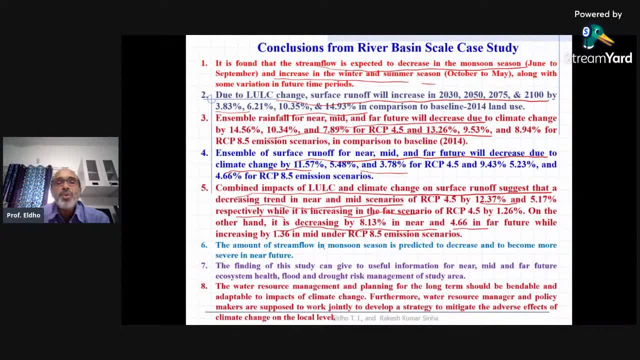 sometimes, as it is decreasing, 20. so so the amount of stream flow is, in monsoon seasons, predicted decrease and become more severe in near future. the finding of this? so then, summer rainfall, i mean during february to may, so that is recently in this region. it is upset, rainfall is increasing and that impacts will be further. 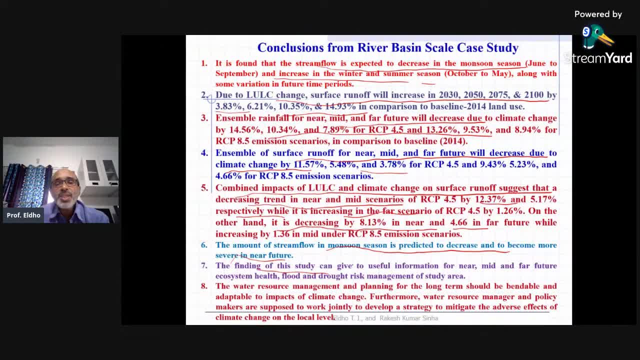 carried over to the monsoon time also, so the finding of the study can give useful information for near, mid and far future. ecosystem health and plant and risk assessment and the water resource management and planning for long time should be um. so we can go for the very various various 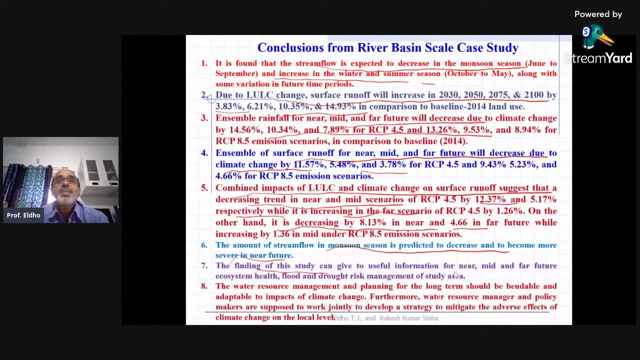 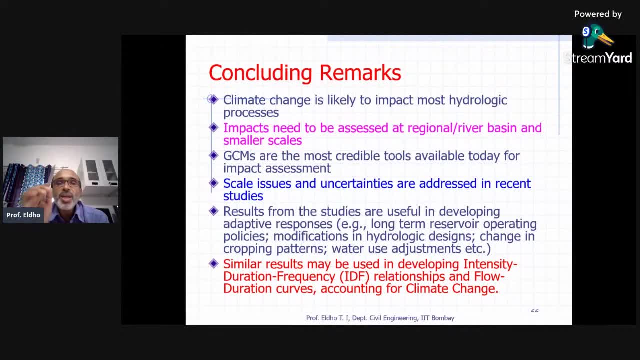 mitigation measures and adaptations as far as these details are concerned. so, finally, to conclude with the information that these are a couple of micro-weapons that we have heard so far that were the한 state which, as we already said, will be prepared for future water, single on water, not only, and 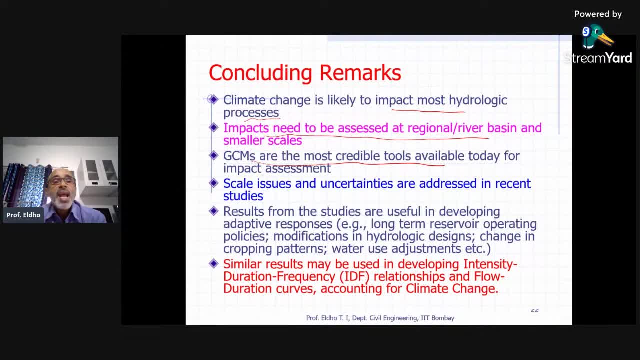 the other one is that a people- humans- can produce the water and fish. they are able to use the water nutrient's. they can help the environment. they can help the environment or else they don't. they can also everyone can do it in out. in the future you can see better water management. you can see better. 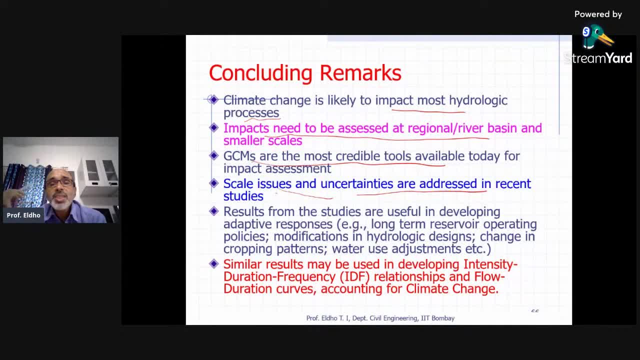 quality, water management, energy, nature, climate change is um so not likely, but it is already happening. and uncertainties so, of course, uh, the gcms. what are the gcms? uncertainty, then, the data answer: there are so many. uh, uncertainties are there. so, on a river basin scale, also, these kinds of 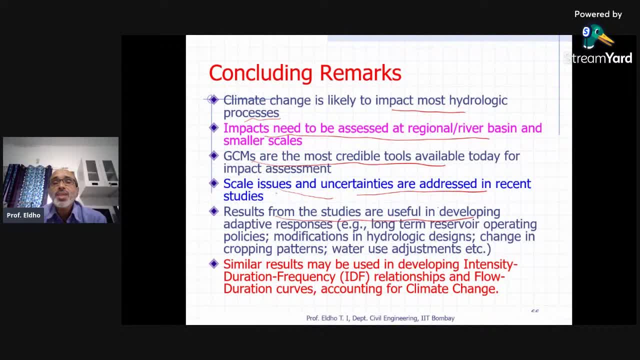 uncertainty studies we need to do and results from the studies are useful in developing adaptive responses like long-term reservoir operation policies, modification, hydraulic design, changes in cropping pattern, etc. and then we can also use similar studies in developing idf relationship and the flow and duration occurs according for climate change. so now when we discuss about the 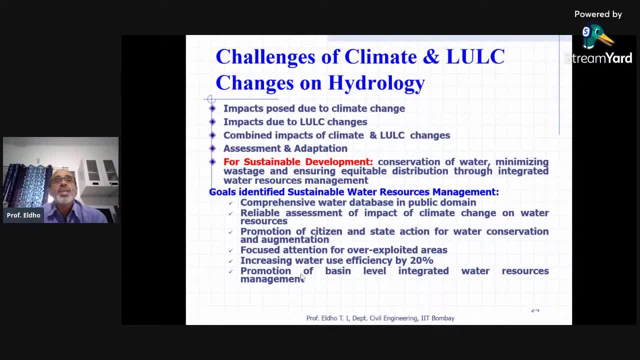 climate change. what are the major challenges with respect to hydrology? so the impacts: climate change impacts positively, so we can see so many impacts we can see with respect to the hydrology's consent. so and then, when it is a not only climate, when the land use, land cover changes also takes place? 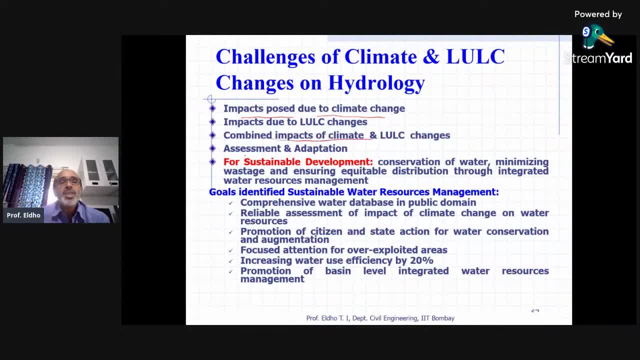 the combined impact is very crucial as far as the river basin scale is concerned, so that we need to assess this kind of impact by considering all the uncertainties also, and then we have to go for further assessment and adaptation, so for sustainable development, conservation of water, minimizing waste. 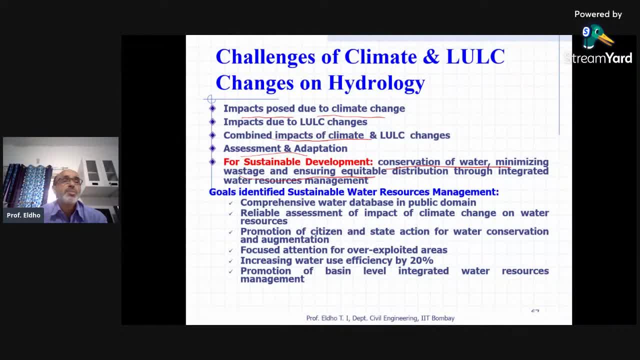 wastage. ensuring equitable distribution through integrated water source management is essential. so that way we need to put various goals for sustainable water resource management, like a comprehensive water database in public domain, then reliable assessment of impact of climate change, so that we are doing for that. we need to try to manage, undoubtedly, water. government of india, ministry of intereses for. 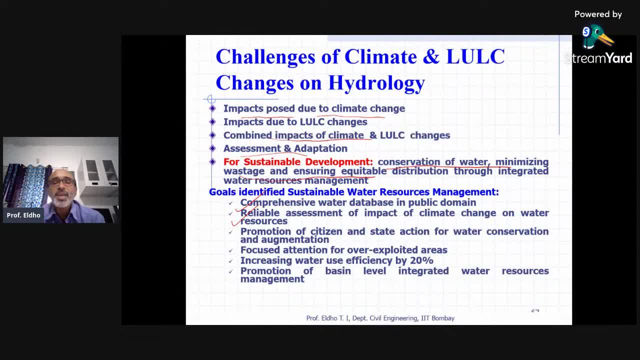 other river basin since then in a Hallke park in Abby hunter university we're. so we have a project based on, sometimes earlier caniamari is the caniamari ocean river basin. have可, then, focused attention for over exploited areas, especially groundwater in many areas are over. exploited areas, especially groundwater in many areas, are originton, so we need to look into the water resources management on a negative way and then focused attention for over persecuted areas. especially groundwater in many areas are over exploited, so we need to focus ourêmany versus many others. so 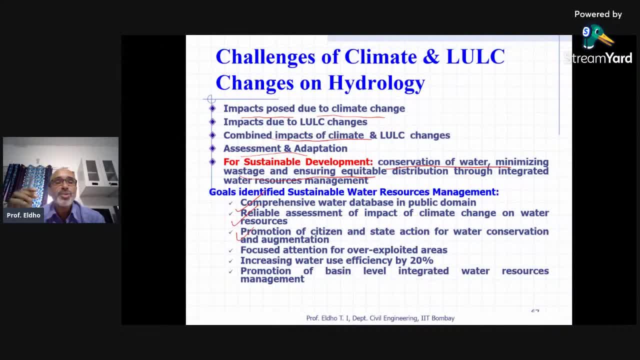 go for ground or recharge or whatever it's impartial is also to be done then. so, of course, in a country like india, the, the, the irrigation efficiency is so low, we need to use the. how further we increase the water use efficiency so that the water scale city and all those issues. 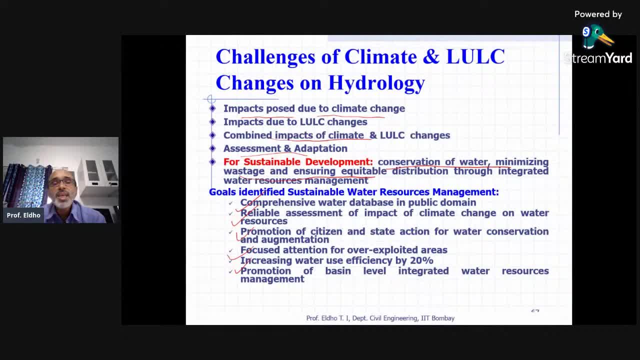 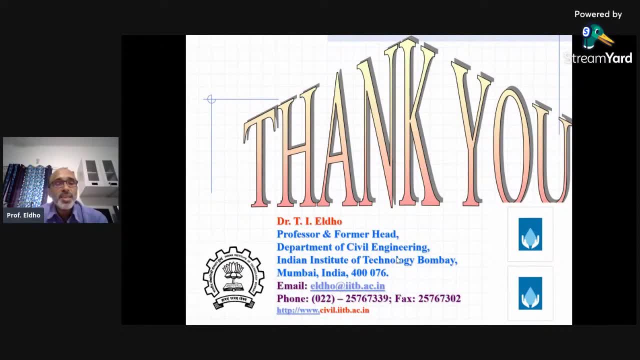 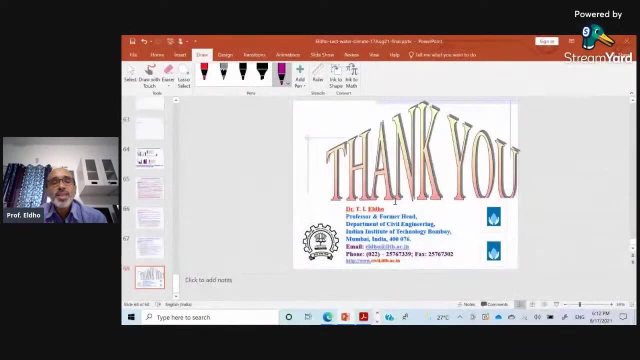 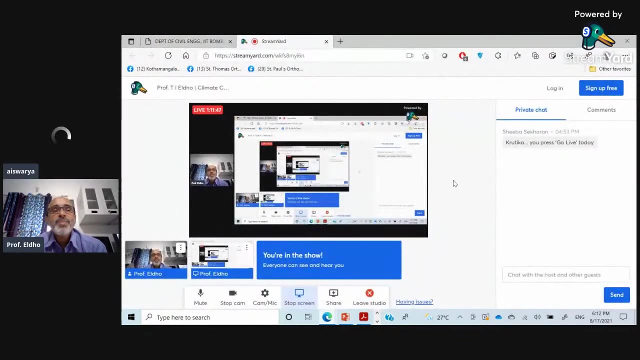 can be sought out. and then further commercial basin level indicator. water resource management is very, very essential as far as the the hydraulic is concerned, the river basin, especially river basin state studies are concerned. so with these- and i am converting this lecture so further, so i will be so happy to say answer to any of your queries, so especially the river basin scale. 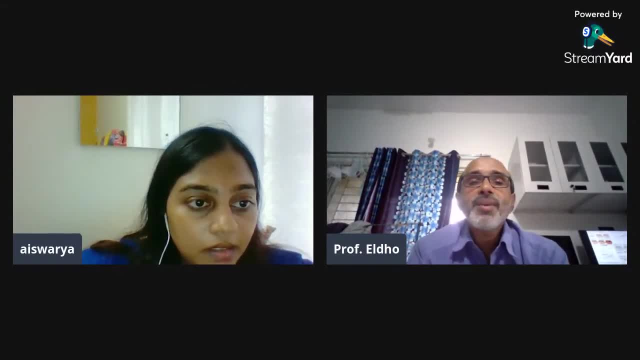 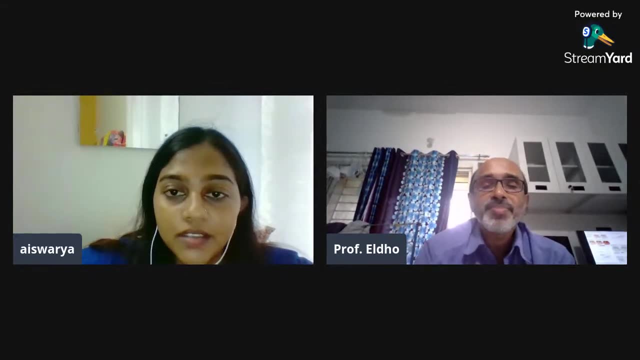 as i mentioned, so important these kinds of studies. so so i'm giving back to the organizers for further proceedings as far as the question and succession is concerned. thank you, sir, for the in-depth explanation. the field of hydrology is important now since it's dealing with one of 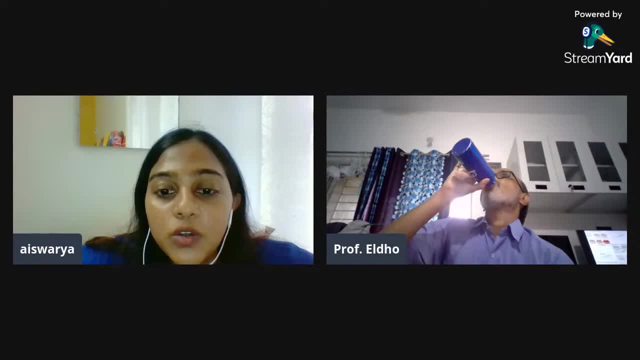 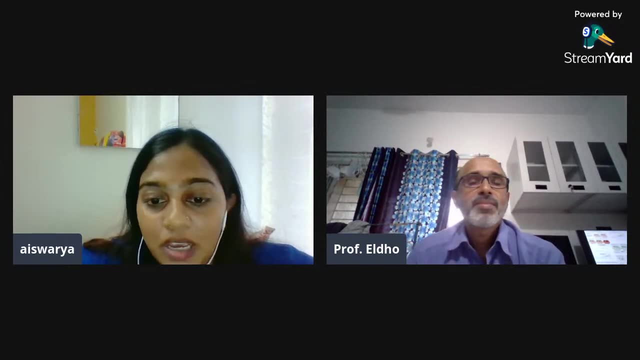 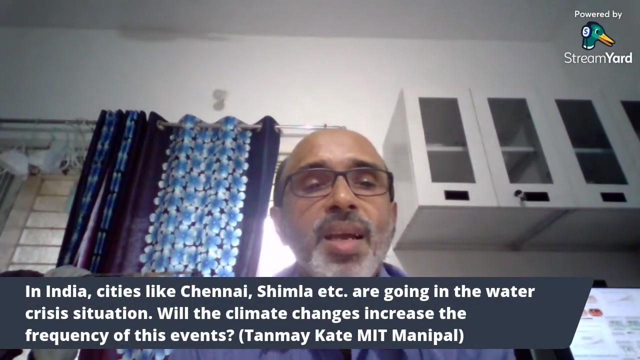 the most vulnerable resources on earth: water. thank you, sir. so participants can type your queries in the spreadsheets, which is already shared with you. sir, we have already received some questions, so can we display it, sir? yes, yes, please, okay, shiba, you can start displaying. okay, the. 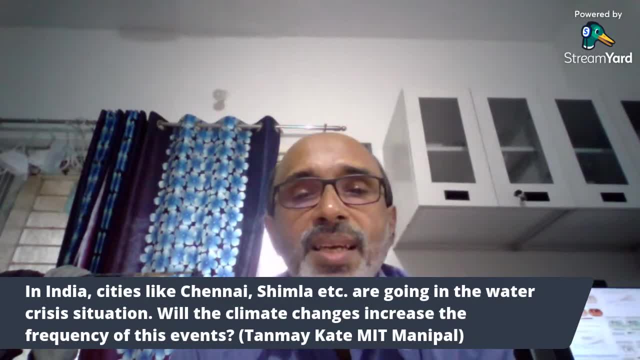 first question is: in the india cities like chennai, shimla, except, we are going in the water crisis situation. will the climate change increase the frequency of these events? so yes, as i mentioned, i can see that now the this, whatever the, like your flooding, or like say whatever the. 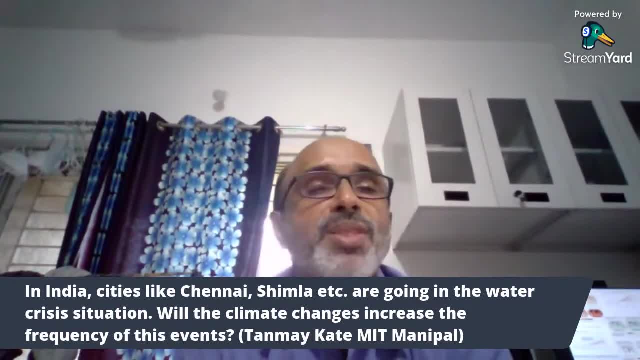 assessment. you can see that in the air 5 and air 6 all the assessment shows that the, the hydrology hydrology will be very intensive. that means the precipitation is going to be high intensive in the coming coming years. and then more events, these kinds of events like the, the flooding, then 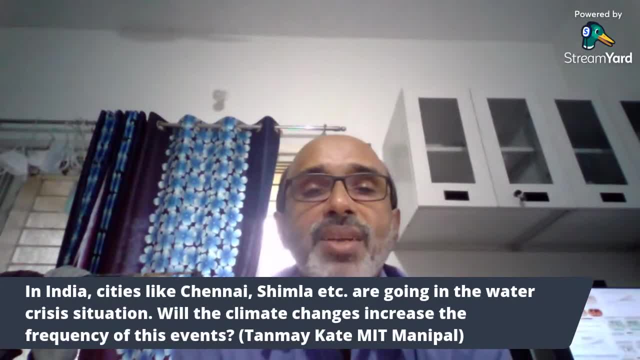 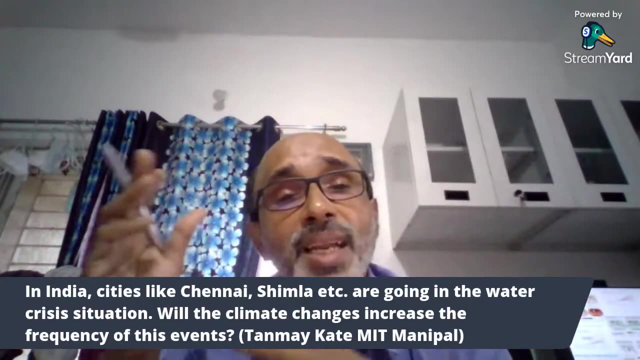 droughts and then also land safe that can. so events are going to happen and then, of course, but as i mentioned, when rainfall happens, the so flooding, mainly flooding test space, high intense rainfall for short duration, that is the cause of flooding, is concerned, but then the total rainfall will be, will be increasing many areas, but whenever it is coming, 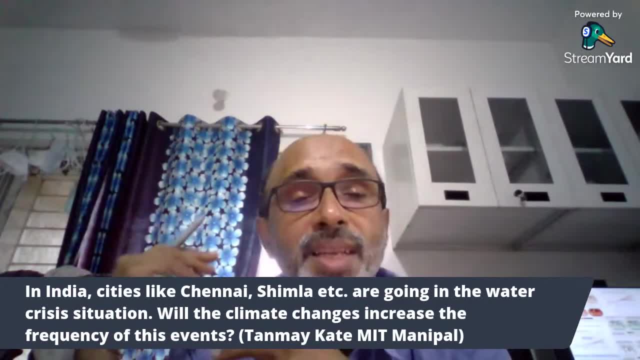 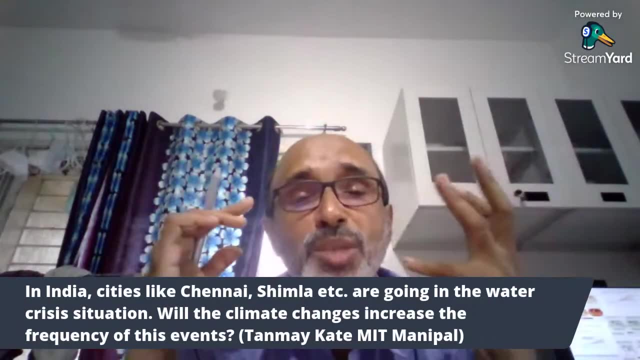 afterwards. there will not be any rainfall for the next few months or like that. so that way there is scarcity of water can also face this. so whenever a heavy rainfall test space, there is a possibility of high flooding, as you can observe in many parts of like, um major pradesh, and then 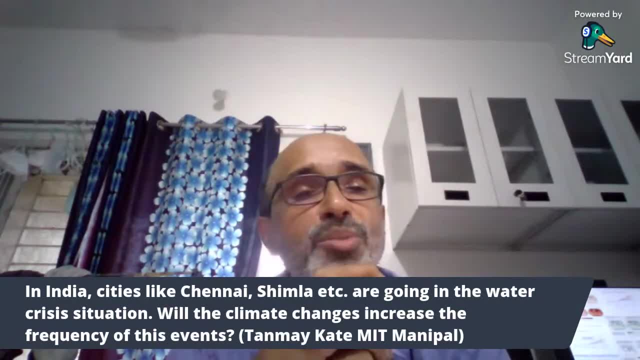 all parts of the country, so that is very much possible. so the frequency of these events are going to increase, as you can observe in this and the all the studies in ir5 or air6 and then further on, i think all the studies will be yes based on that, so i hope i answered this question. next, 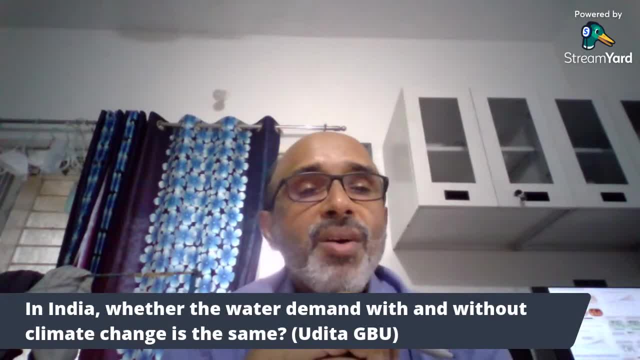 question, please. okay, the question is in india, whether the water demand with and without uh climate change is the same. so actually, it is not same. actually, you see, this is the best upon some statistics based upon 2000 and um 2002, between 2010, but, uh, that changes here as i. 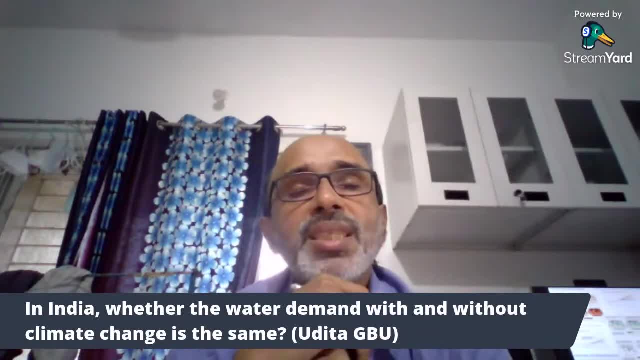 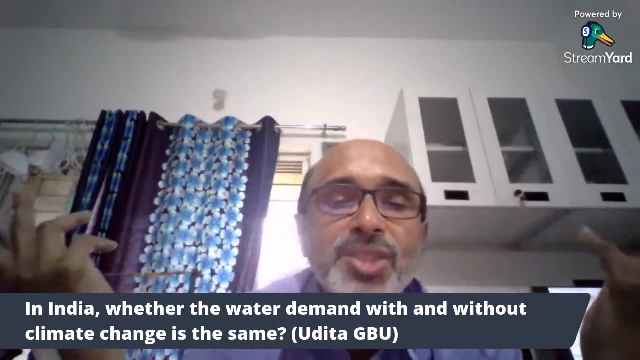 mentioned water availability. so, for example, what was there in 2000? having 2000 meter cube per person per year. then by 2050, since our population is also increasing, that will be coming down drastically. so it will be becoming around 1000 meter cube per person per. 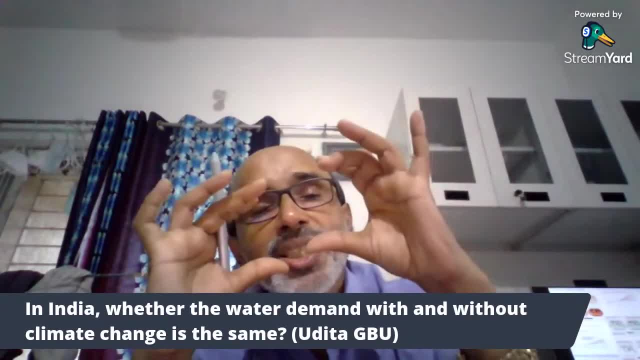 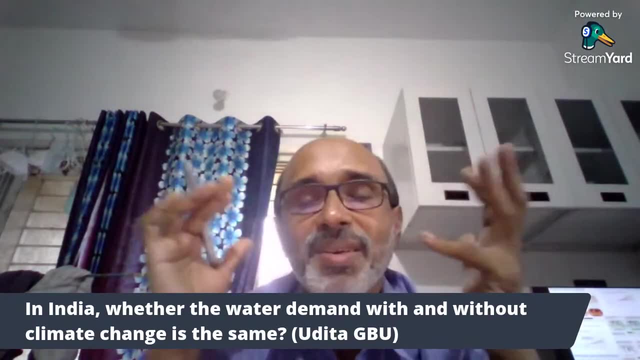 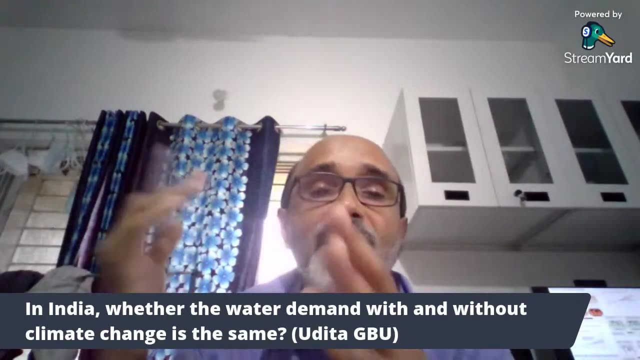 per year. so that way that changes, even though, as you can see, that plot, it is small, but that plot is per person, that is, please remember, it is per person, whatever you put it. so but that change itself since already available, there is a water scarcity. then, with respect to that, even climate, 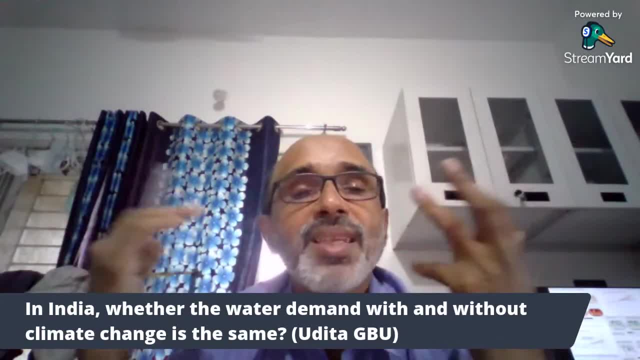 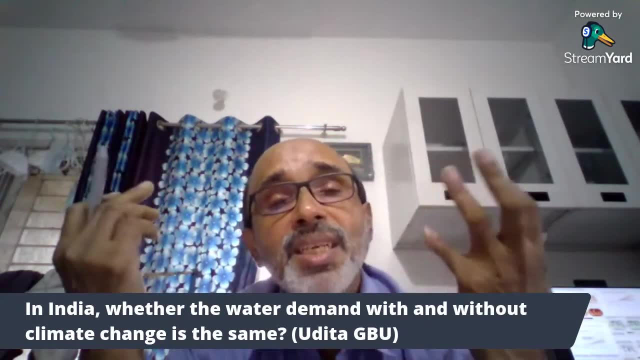 change impacts also takes place, then it is the effect will be very severe. so you can see that. what is, though? the precipitation going to increase, but whenever it happens in a in a very heavy way, it happens, then we cannot store the water in reservoir. so that is what is happening in a state. 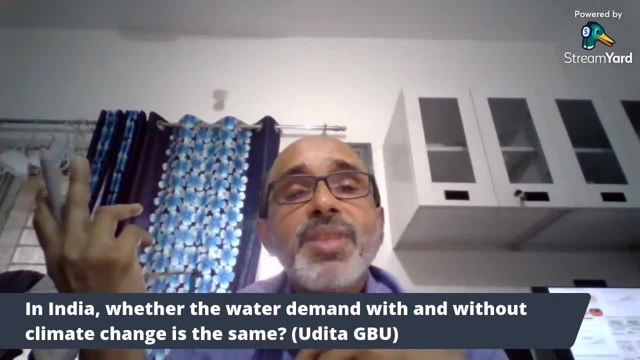 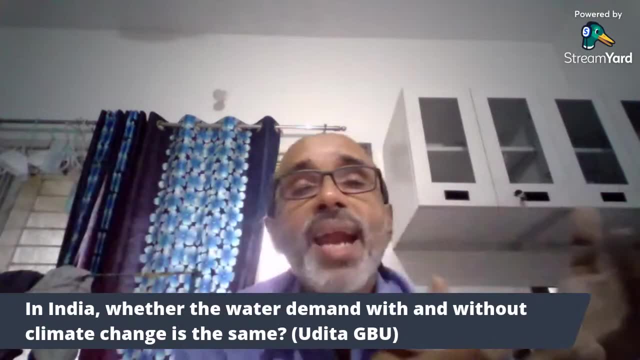 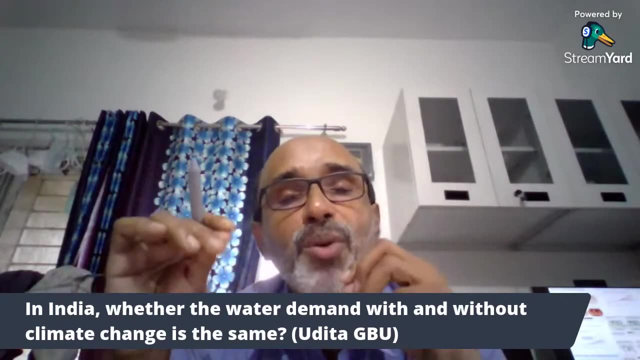 in kerala 2018. you can see many of the dams which were they kept. they kept on storing the water, but when the heavy rain takes place, they have to release everything, so that also added the flooding problems. so that way, the problem is that whenever heavy rains stay space, it is for short duration. uh, the number of events will be. 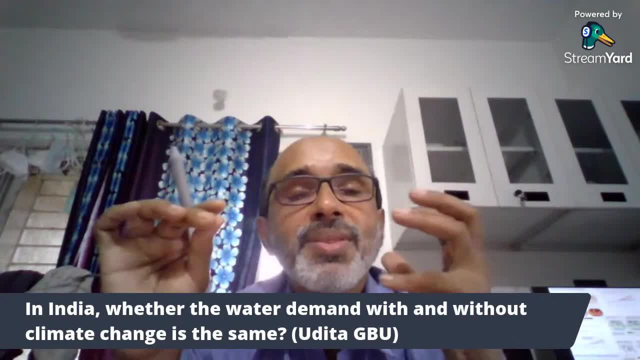 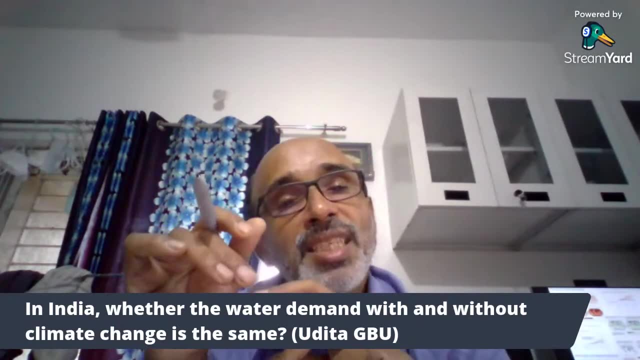 decreased and the events happens in a very, uh, severe way. so that way, the flooding will be the, the final, uh, final outcome. so that way, as i mentioned so here, a climate change impact is definitely there, uh, but the per person, whenever you put it, that that amount may be small, but that. 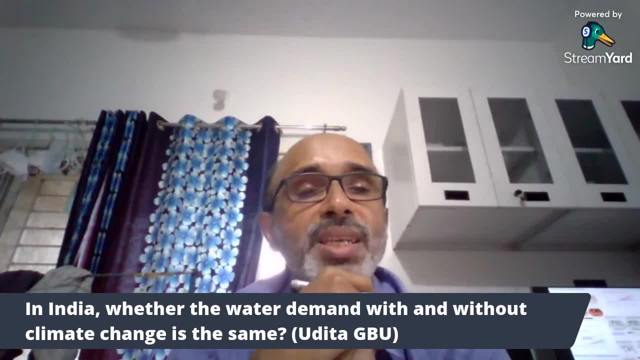 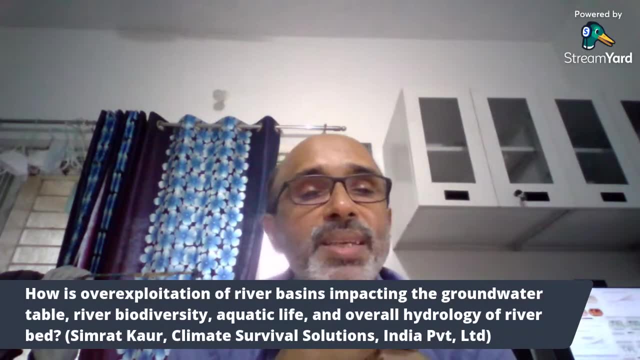 itself is too severe. okay, i hope i answered that question. next question, please, now we saw. our next question is that: how is over exploitation of river basin impacting the groundwater table, river biodiversity, aquatic life and over hydrology of river? uh, river bridge, uh, so here, uh, so here uh. 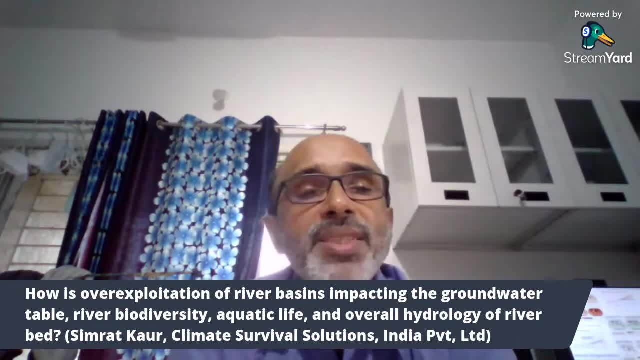 how is over exploitation? of course, as i mentioned, that many of our river basins are over exploited. say, for example, if you take uh, kaveri or godavari or krishna, all these river basins are or or or exploited. so that way, since uh, we have got a number of uh. 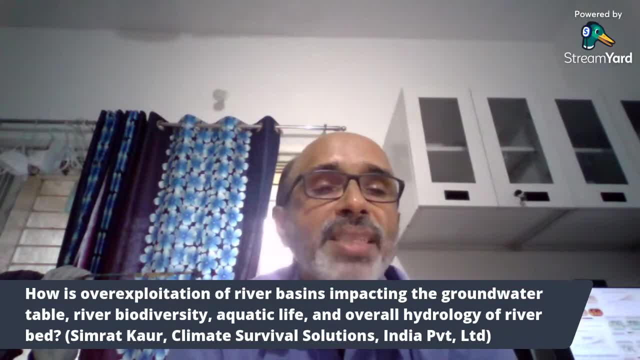 uh, so that way? uh, with respect to this climate change impacts are concerned, as i mentioned, what can happen is that: um, so, whenever the, the, the, we cannot store that much water, since the severe, intense rainfall space for few events and the total amount of rainfall may be higher. but uh, 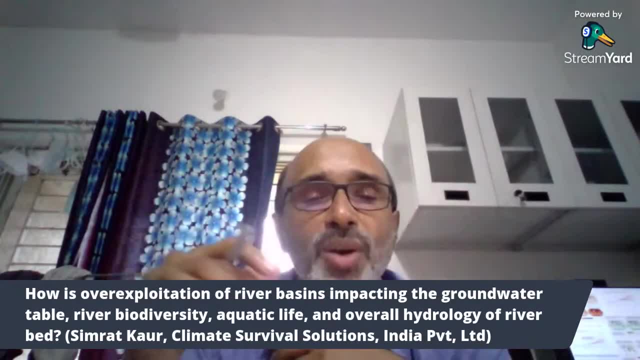 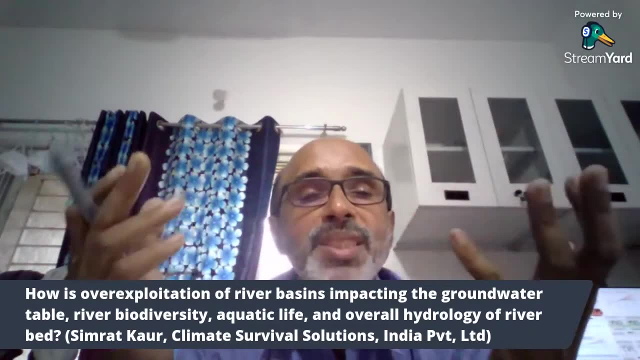 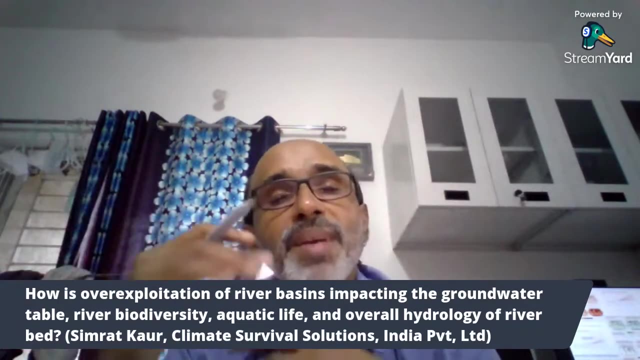 whenever it stays, facing, say, within few events, the storage possibilities. there is some limitation to the space and that way, uh this, um, uh the for the basins which are over exploited, there will be more impacts as far as the the biodiversity, since the environmental flow will be decreasing, since, uh as 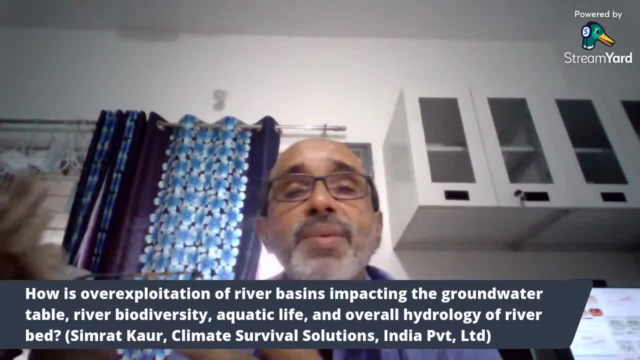 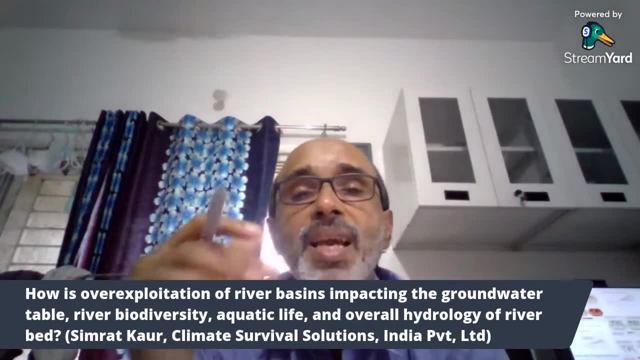 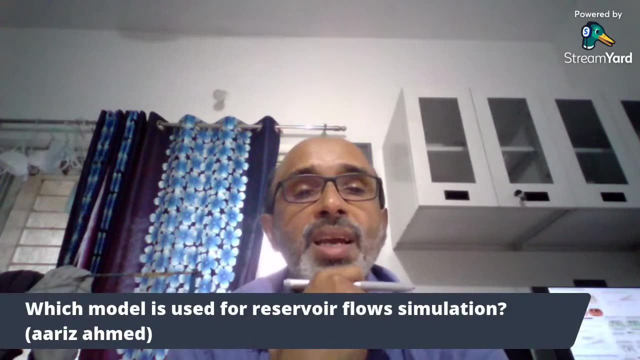 i mentioned in the climate change, that is, whenever rains happens in few events and afterwards no rain. so that means the environmental flow will be affected. so that way, biodiversity, aquatic life, everything will be affected on a river basin scale. okay, next question, please. uh, so reservoir flow simulation. we can say here, you see that reservoir flow. 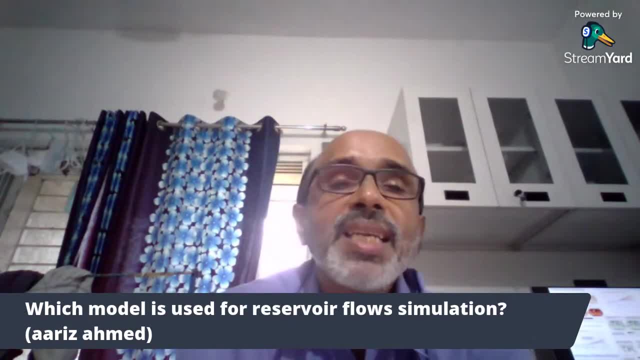 simulation is concerned, and we have, we are having. so that depends upon the areas, like as a we, we can have a number of models, like a systematic, like based upon the like, dynamic program, linear programming or in the the, the combination of all these kinds of models are possible, reservoir flows, simulation is concerned, and whatever i hope this question is for. 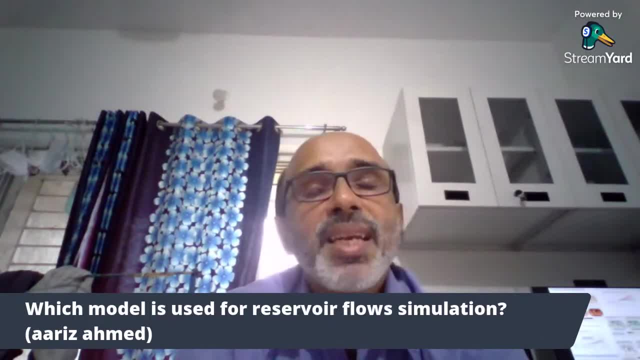 the flow coming to the reservoirs. so here are that kind of simulations we can definitely do on a river basin scale using the, the, the, um, swat model itself, and then um, of course, uh, uh, the, the vic model which i mentioned. it is a little bit more, since it is good based model, uh, so, but the sad. 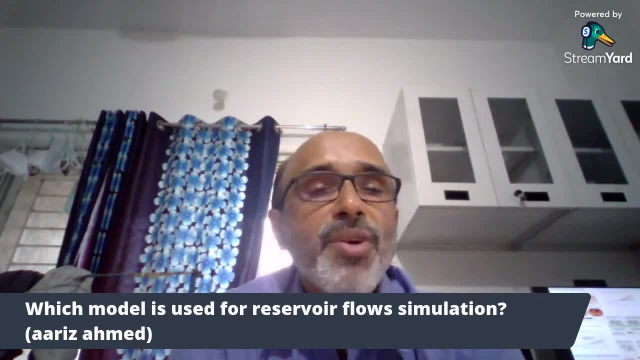 model can be for whatever the inflows are coming to reservoirs, but reservoir now the start model is and the vic models. we can also uh, incorporate the reservoir aspects also and then that the models are modified recent times and that we can put it for that kind of purposes. next question, please. 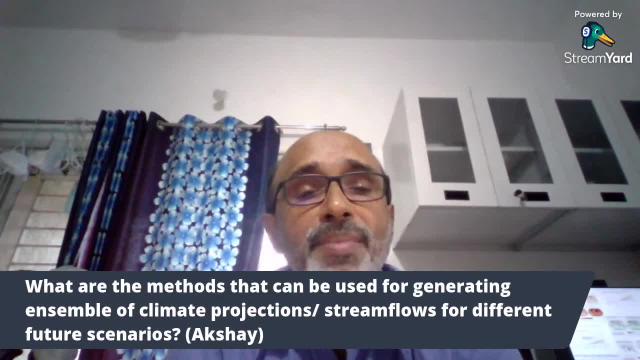 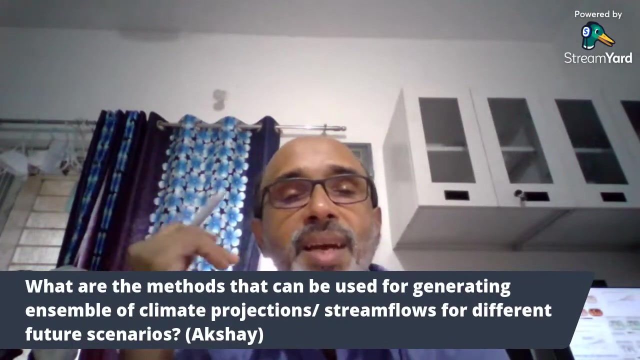 what are the methods that can be used for generating ensemble of climate projections stream flows for different future scenarios. so here um generating ensembles. so you see that we can say, as i mentioned, we need to first downscale the data and then do a bias correction and then, based upon the particular gcms, so that data the different methods of like you can give a. 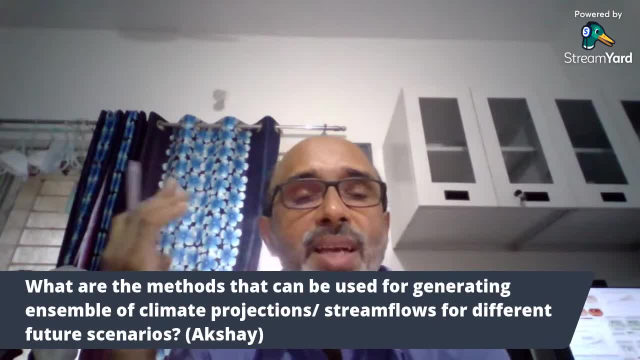 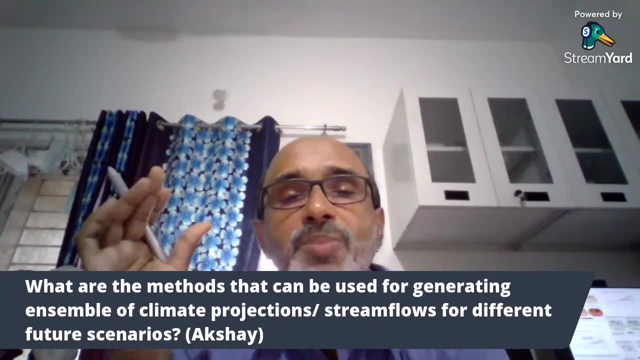 the, the impact i mean with respect to grid device. you can do. a variety of methods are possible, uh. so i think here, uh, we used, with respect to the, the averaging of whatever is happening with respect to grid scale. that is what is done. so, but, um, we need to whatever the downscale data. 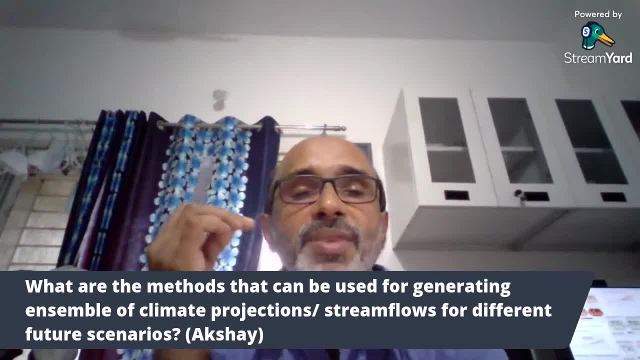 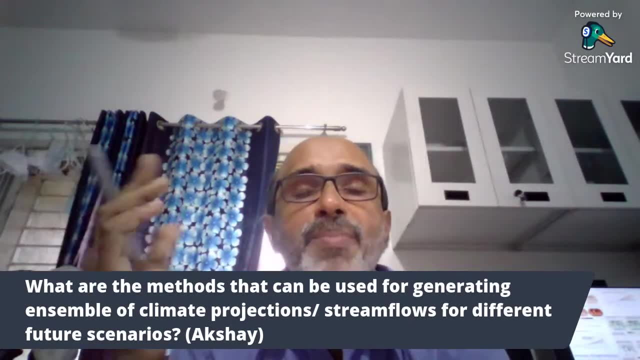 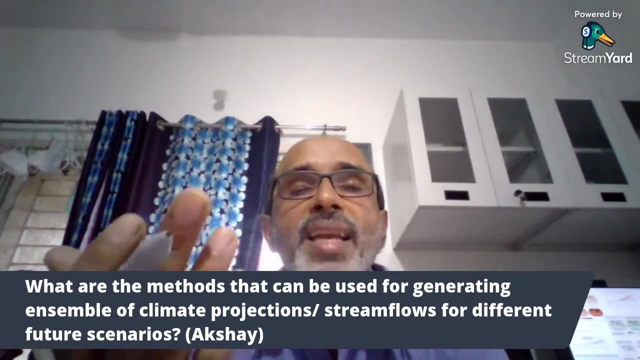 so first we need to verify, with respect to uh, each gcm with respect to past data and then, if it is coming, the trend is getting better, then only we go for the, the assembling. with respect to um, say, as i mentioned, five gcm which we have used for this river basin scale study and out of that for each basin it is. 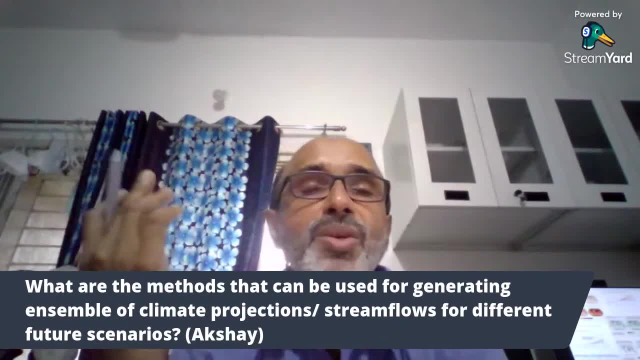 varying. so some basins it will be giving, some gcm's will be giving good results and some other basis to be different, so that we see, we observe that each gcm which we consider, how is the performance? and then we go for the, the assembling of uh with respect to that, the best, best performing gcm. 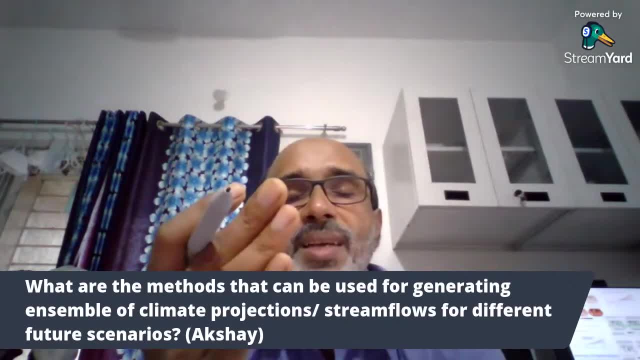 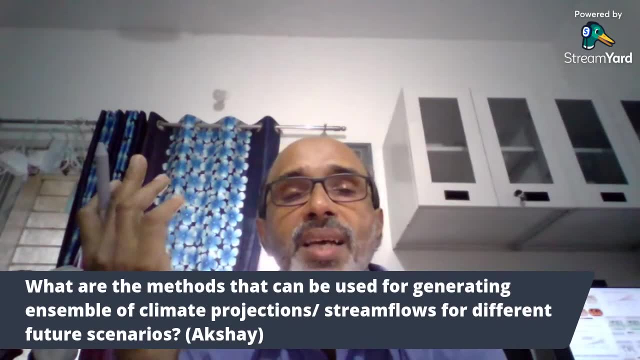 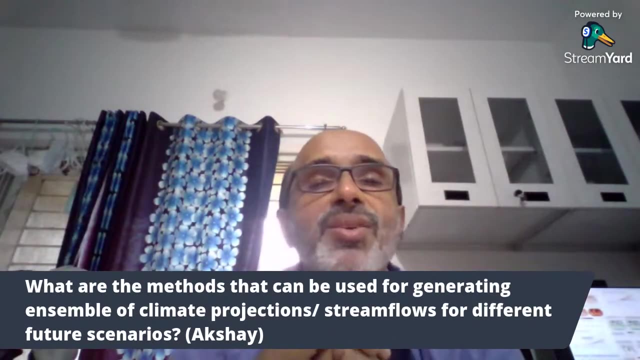 so, for example, the, the, the details shown by shown in the procedure paper area by which i are shown. so that is, they are using around 16 gcm and then another study is about 32 gcm. so a large number of to. to deal with the uncertainties related to the gcms, all guys better to use number of gcms and the. 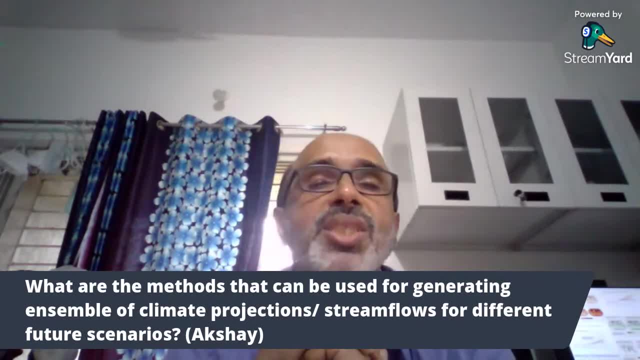 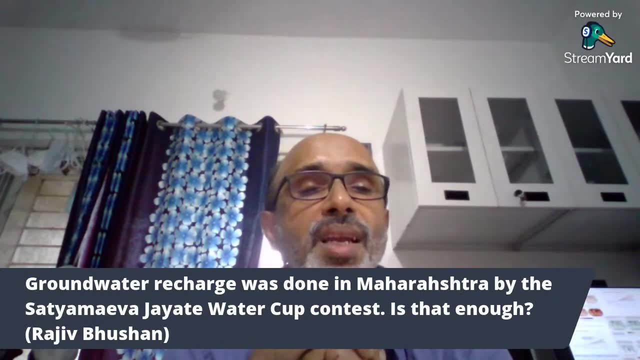 uh, identify which gcms are giving better results and then go for ensembling, ensembling uh technique. so next question, please? and groundwater recharge was done in maharashtra by the septima water. is that enough? so groundwater recharge? of course these are our small scale scale studies. 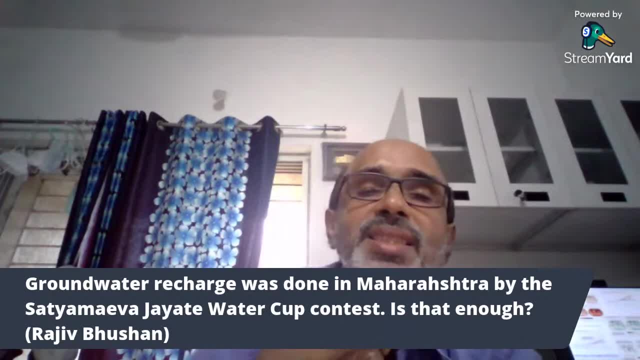 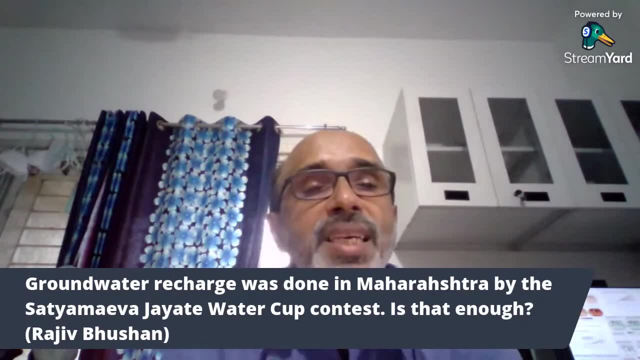 we need to see that scale studies, each river basin scale studies: how much is the surface water, groundwater availability and then, uh, whether we can increase the groundwater recharge through various schemes like, as i mentioned, watershed indicator, water resource management, which is- we are also talking about watershed management, watershed management practices to be 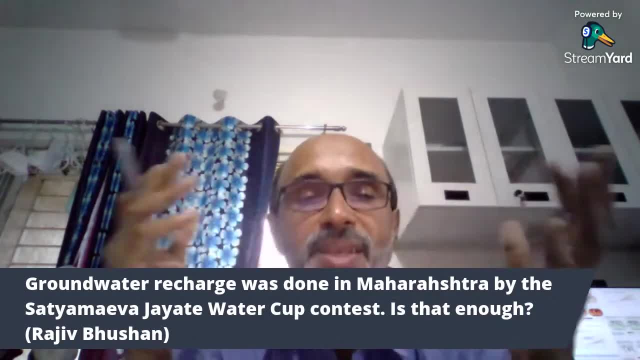 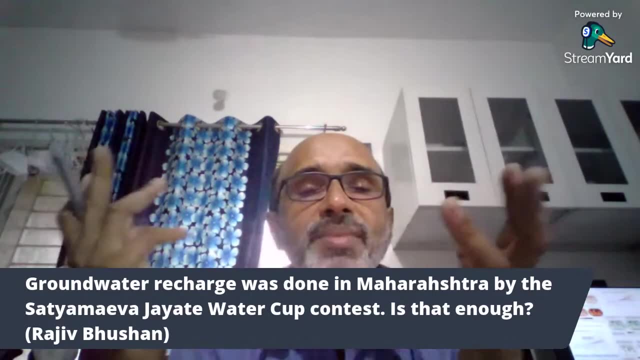 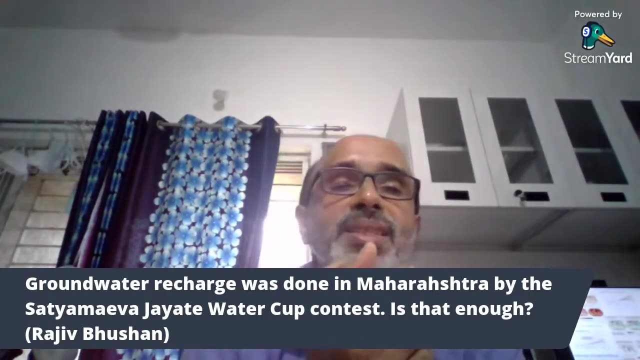 say, become universal, so i mean all areas. we need to go for that so that the good groundwater recharge can take place. and then many small, small studies are available with respect to the the impacts of watershed scale intervention as far as groundwater retard is concerned. next, next question: 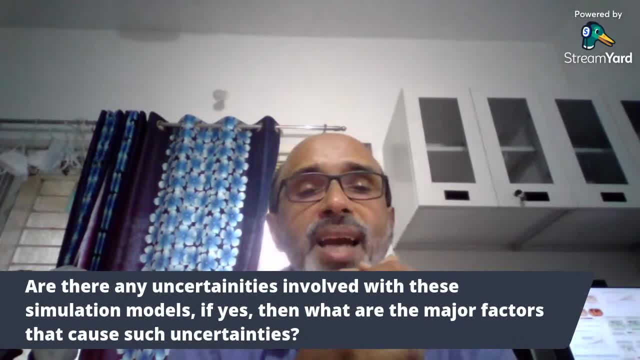 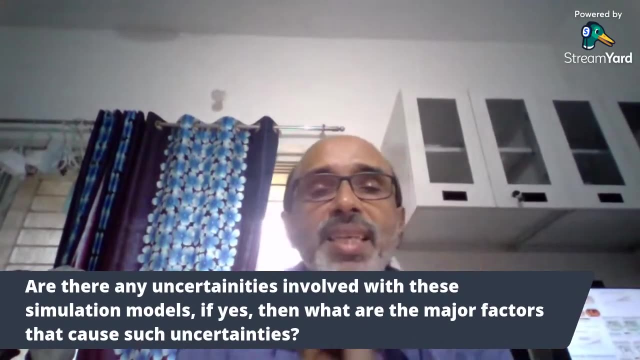 please. are there any uncertainties involved with these simulation models? if yes, then what are the major factors? of course, as i mentioned, uncertainties. there are. so many uncertainties are there with respect to the gcm uncertainty, one that is the climatic data is concerned, then the data uncertainty, whatever data we are using, and then, of course, model uncertainty is also there. 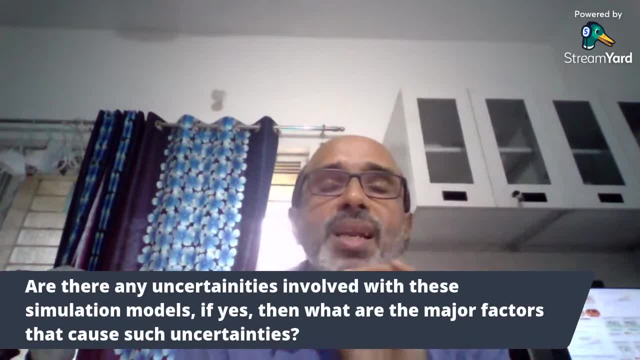 so, for example, if we are using so swat models, that model where we use number of assumptions and it is semi-distributed model, or if we are using vic model or migration model, each model has its own assumptions and that model uncertainty is also very important. so, these uncertainties, it is always 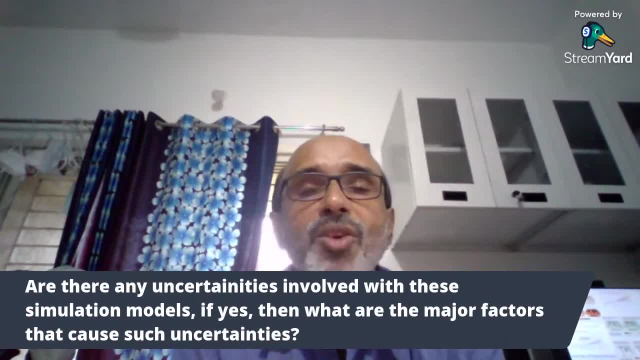 better to so. anyway, if you are doing comprehensive studies, it is better to study the model uncertainties also. so that way, whatever the the swat model use or the vic model use, there can be some differences. so that kind of uncertainty is also it is always better to take into account while while considering these kinds of river. 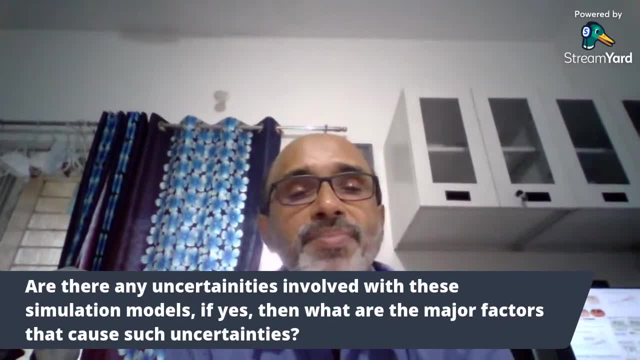 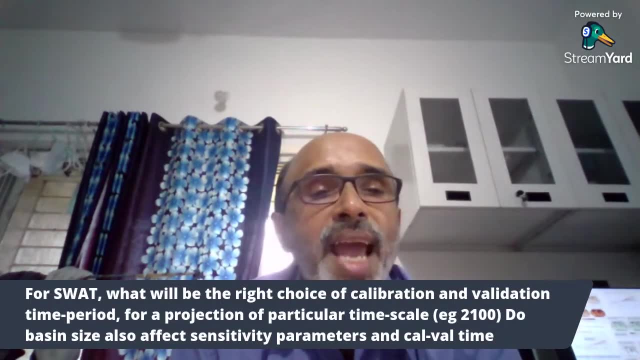 basin scale studies are concerned, yes. next question is for swatch: what will be the the right choice of calibration, validation time period for a precipitation particular, say time scale. so here, as i mentioned, say, if you are having a large data set, i mean reliable data set, so then say generally a minimum we prescribe, at least. 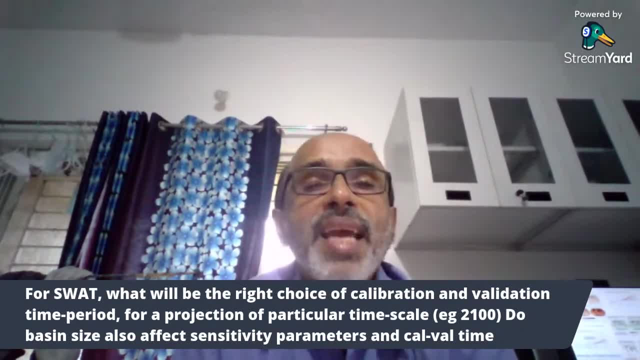 minimum, six years calibration minimum. so if you can go for 10 years, that will be generally good enough. so six years, even six to ten years, will be good enough for calibration and then, so especially, we are doing daily the scale we are using and then we can validate for another six to ten years. so 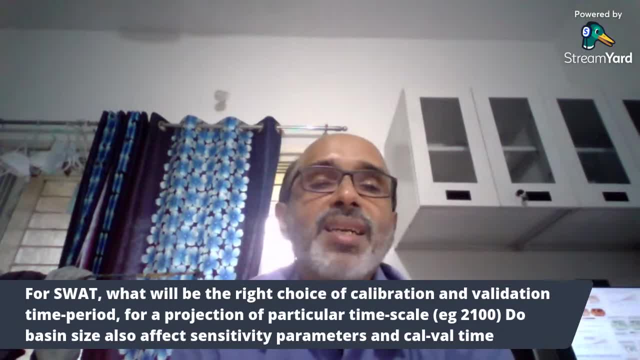 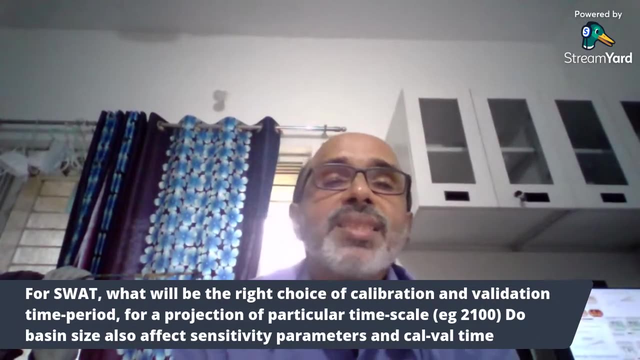 that is, the general trend is there, but the minimum five to six years is required. so that is the, the minimum requirement, and the better is going up to at least ten years. so so, since we are using this model for further, after 2100, so that is why i am saying at this time, minimum 10 years. 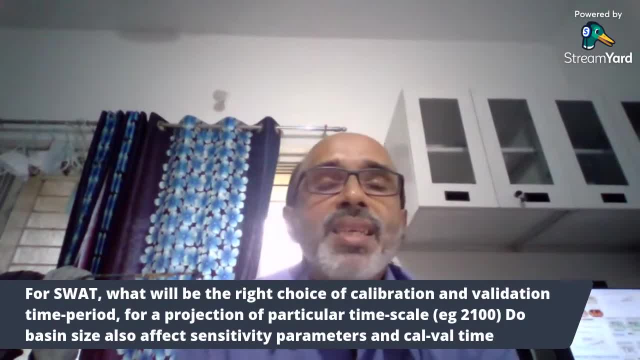 will 6 to 10 years, that for calibration and validation further. i mean 10 years for calibration and 10 years for validation. that is the best choice, and but if you are having better data, then you will take face ten yearsраз forty years for the calibration and validation, and then you will take six to ten years for the calibration. that is the best choice and but if you are having better programs, that case denken wir und hat you lu 있을betteradan ہem. LuckyData system needs to get some. 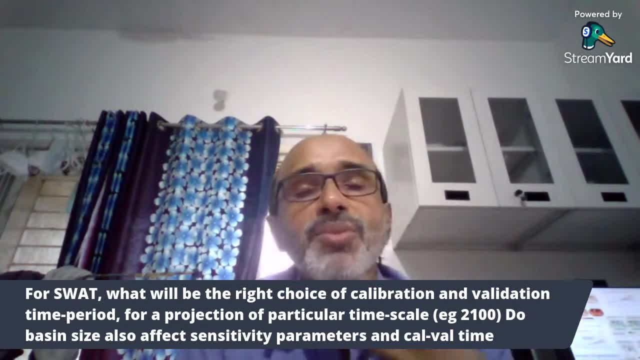 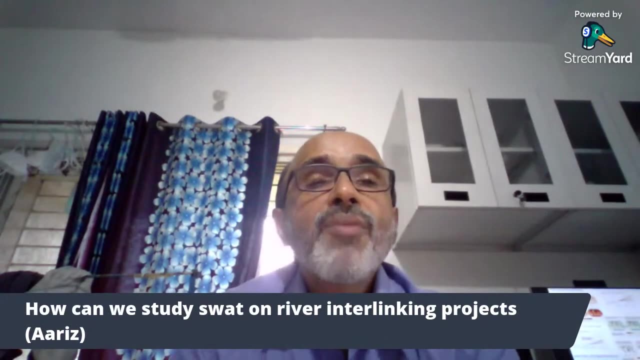 that the model confidence will be increasing so that we can use for further, maybe 10 to 15 years also, if it is available, But average say five to 10 years. data is required for calibration and validation. And next question, please, Of course, the last question part is that. 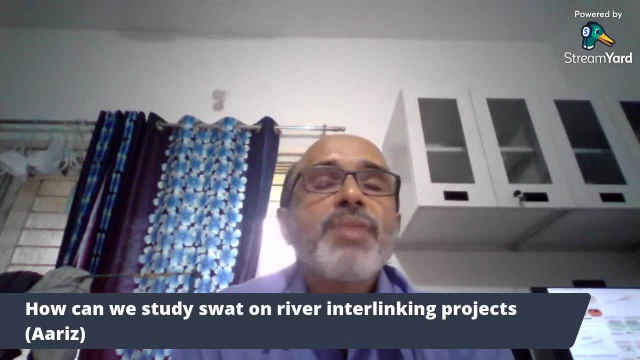 of course the river basin is also important. If it's small river basin then the data requirement will be in the calibration validation. with the data the years can be reduced, But for larger river basin it is better to go for a longer span. 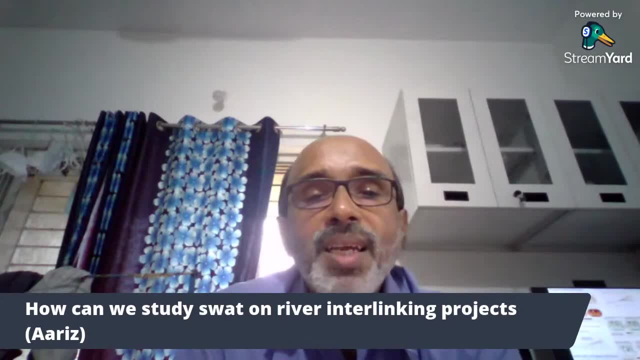 And next question is: how can we study SWAT on river interlinking projects? So river interlinking projects are concerned, of course, what we do- so as you can see that we have our plan- is to transfer the water from one basin to another basin. 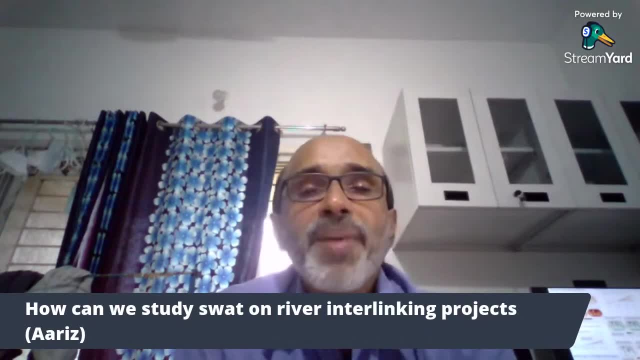 So for that we need to assess each river basin separately and then, whatever the how much water is needed, is the same water surplus is available or not? And then based upon that only we can decide. So that is the major issue. So we need to study each river basin. 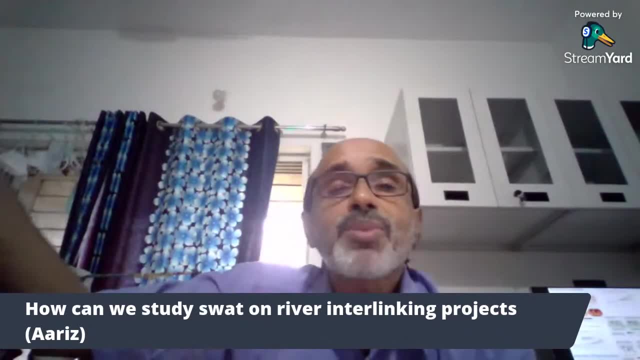 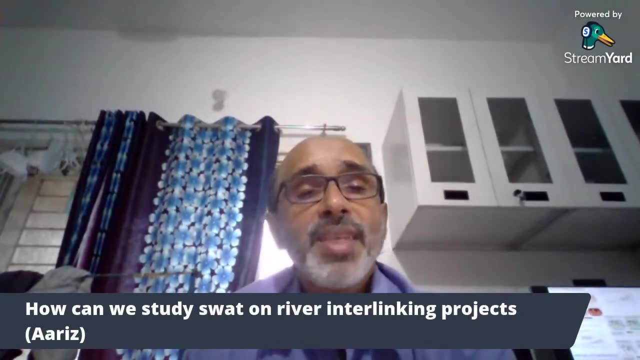 is historical past data, using past data and then projected data up to 2100. And then only we can take these kinds of studies. So each river basin scale studies is very essential for river interlinking projects, So that what is SWAT model we can utilize. 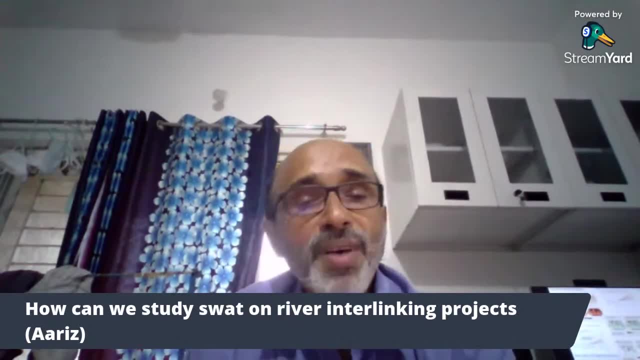 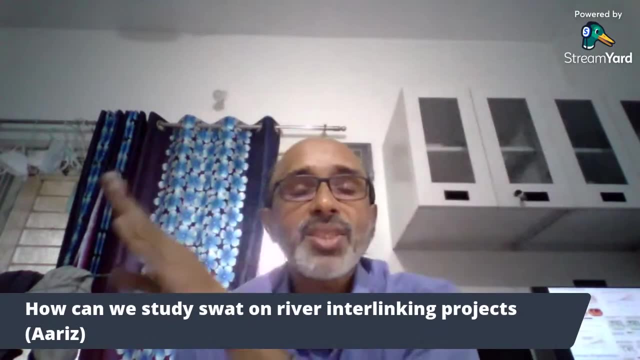 or other kinds of models also we can use for this kind of study. So first we do past in the historical data, using historical data, and then the projected data can be used and so that, whether it is consistent, trend is there or whether after a few decades- 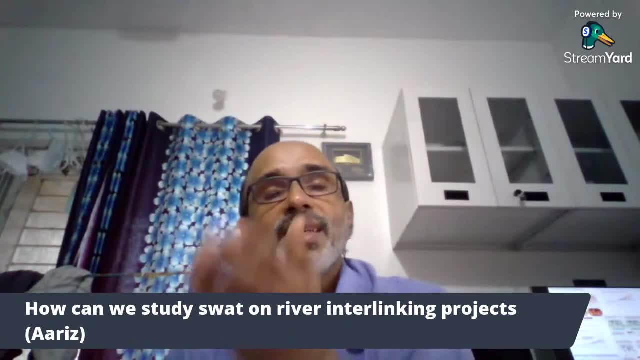 whether it is going drastically reduced, then the river interlinking may fail. So that is the issue. So we need to see, with respect to the past, historical and the future projected, And then for each river basin, the water to be interlinked, we have to study. 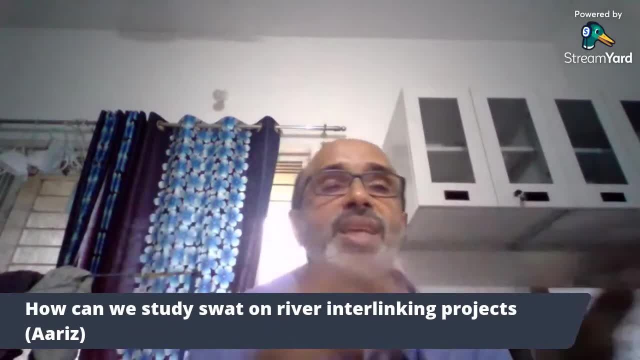 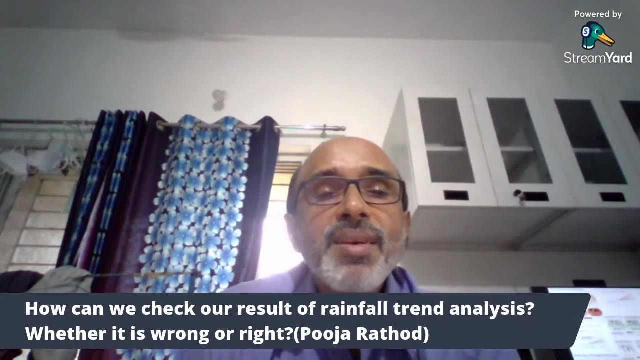 And then we can see that, whether surplus water is available or deficit, how it is, And then we can do that to be the best way to do this. Next question, please. Any other question please? Yeah, So how we can check our results of rainfall trench analysis? 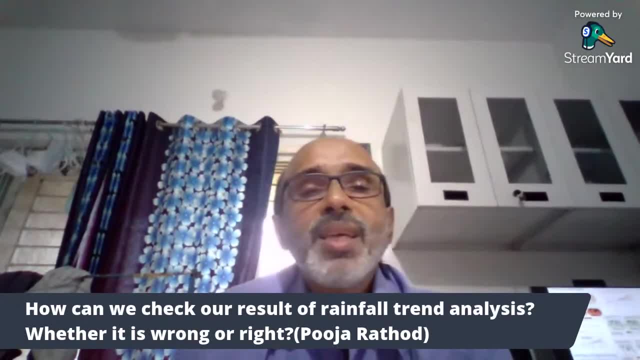 whether it is wrong or right. So what do we do? So the best way is that, so the climate change is concerned, generally, we put a time span of 30 years. So what do we do? say, for example, whatever in our analysis. 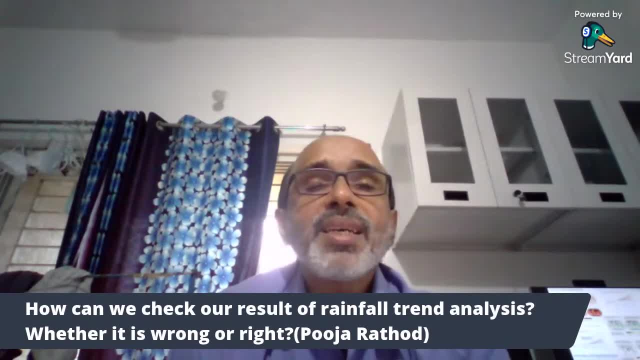 consider 1980 to 2010 data, Whatever the rainfall data, what we obtained from IMD, So that data we are used for checking whether it is getting good trend or not. So that is, as I mentioned, the GCM data. 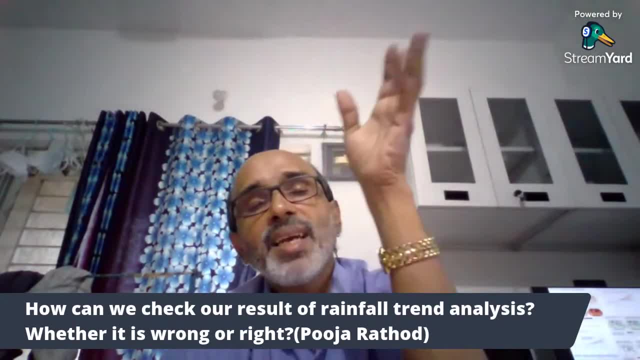 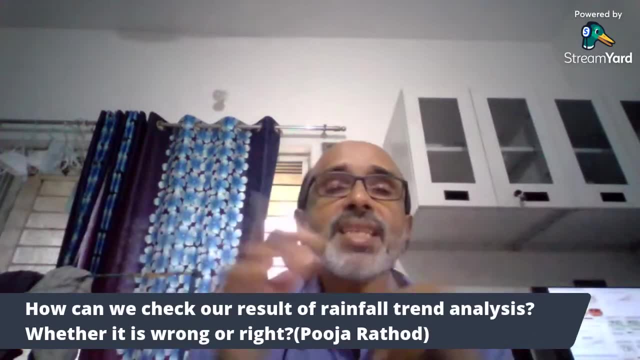 GCM data we can get from whenever the simulations start, 1980s or 90s onwards. up to 2100 data we can get it. So what do we do Generally the climate change studies are concerned? Generally we use for 30 years span. 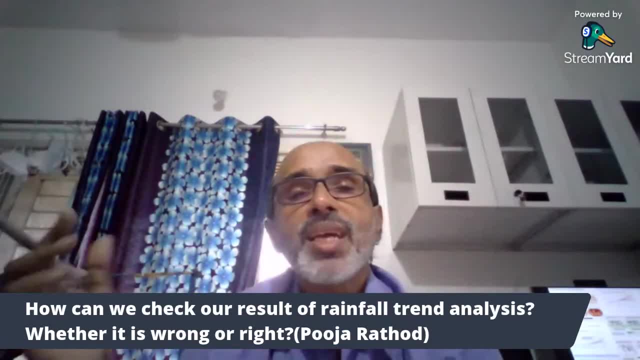 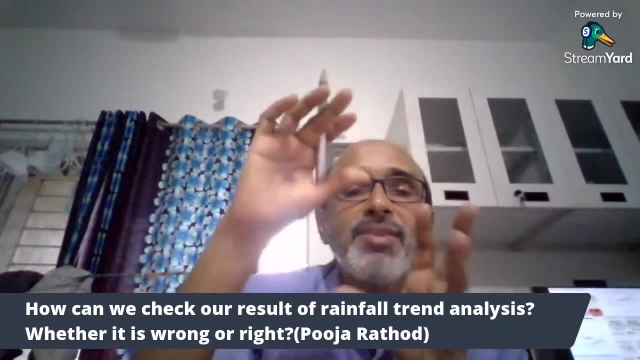 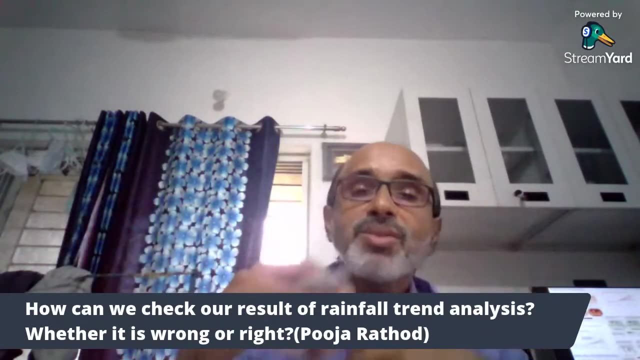 so for that 30 year span. so you can take 80 to 2010 or 90 to 2020 or whatever the retrospective data, and then we check with the- let's say, india is concerned. imd data will be using that data and then what the gcm data is getting and then we will be using whether further bias correction is needed. 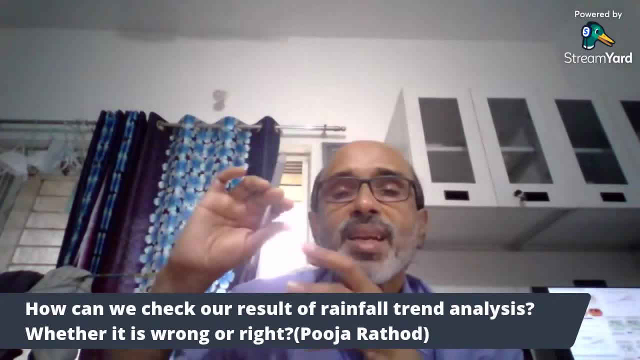 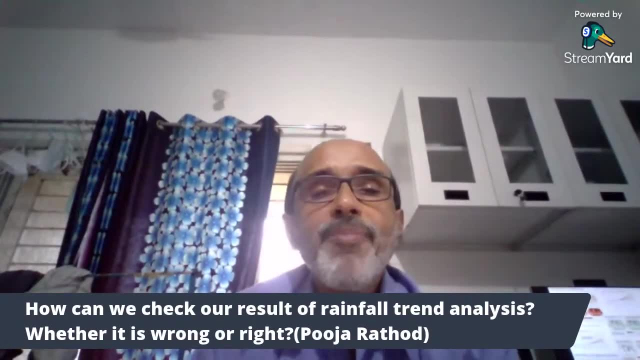 so if the bias is there, then we will be doing the particular method we will be using for bias correction and then we will be. if you are getting good correlation, then that data can be used so generally, uh so rainfall trend analysis, we have to do a 30 years time period and if it is getting 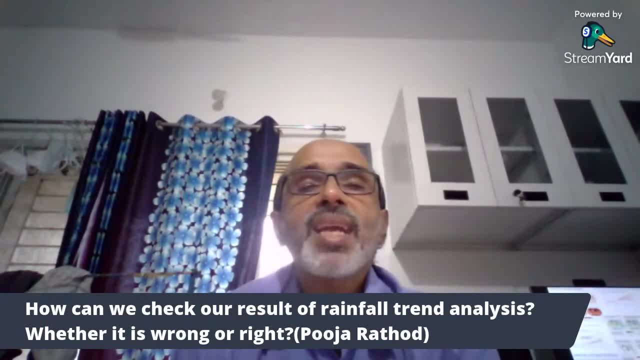 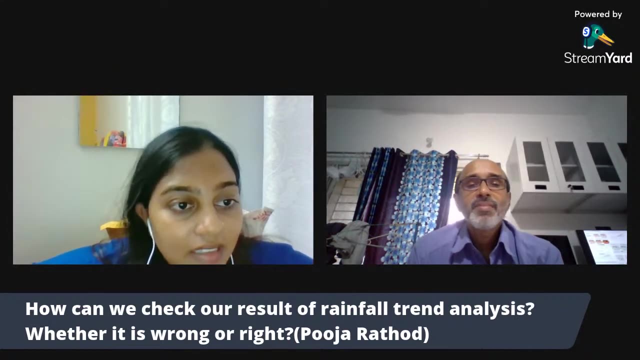 good trench, then that data- we presume that is, whatever the data getting is good, and then that gcm data we can use for further, further projections and further studies. next question: so we have, we don't have more questions, and okay, okay, fine, so uh, we can wind up this section.